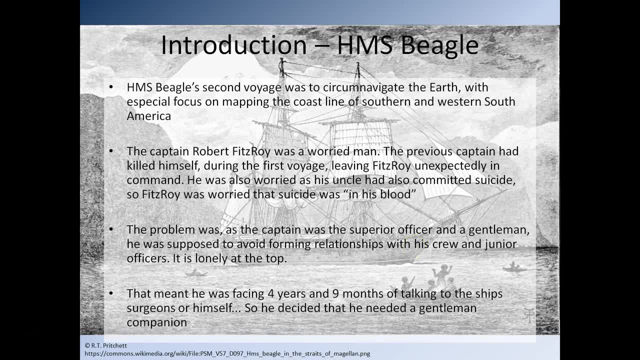 was Captain Robert Fitzroy, and Captain Robert Fitzroy was a bit of a worried man. So during the first voyage, which was also a circumnavigation of the earth, the previous captain had become depressed and he had killed himself. Also, Fitzroy's uncle had committed suicide. 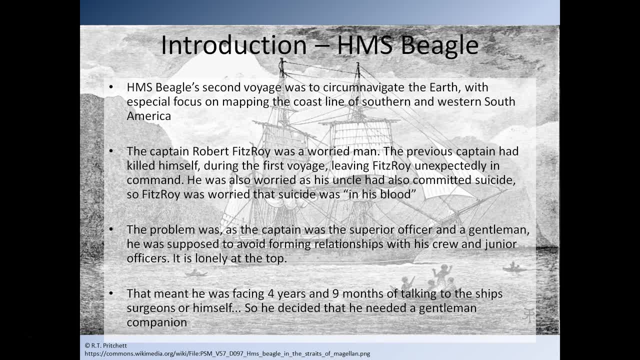 so Fitzroy was worried that suicide was in his blood. At that point there was a view that you know, suicide was essentially something that could be passed along the family bloodline. So the problem was, was that the as the captain, he was considered to be the superior officer and a 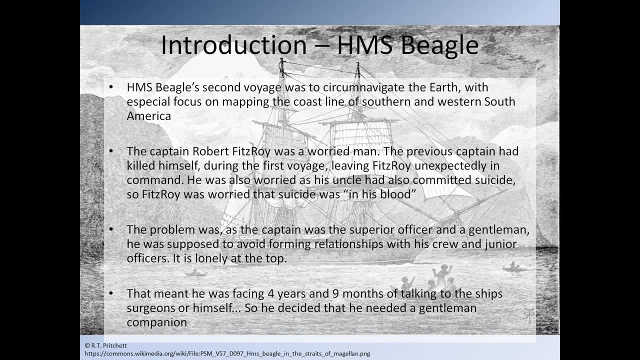 gentleman. so he was supposed to avoid forming relationships with his crew and junior officers, you know, in case some kind of strong relationship you know formed and it made it difficult for him to command the ship. So essentially for poor old Fitzroy it was lonely at the 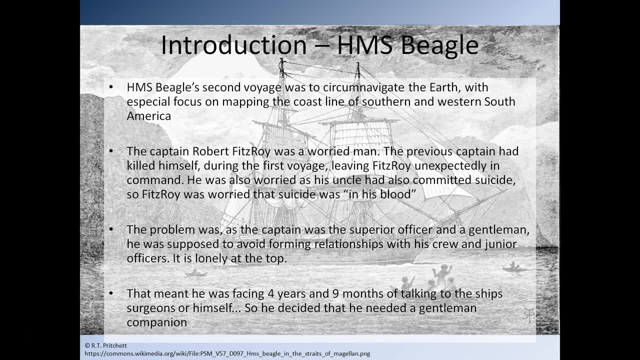 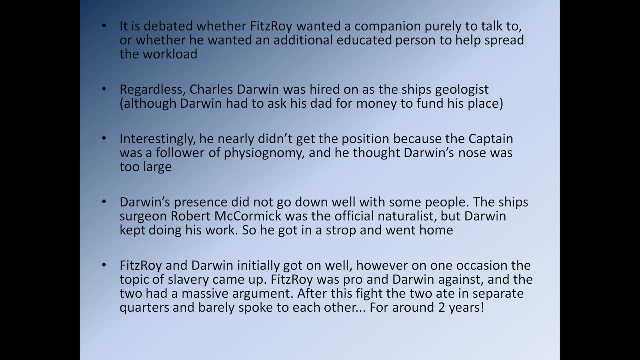 top. So this meant that he was facing, you know, around four years and nine months of talking to the ship surgeon or himself. So he decided what he really needed was a gentleman companion with whom he could converse. So it's debated whether Fitzroy wanted a companion purely to talk. 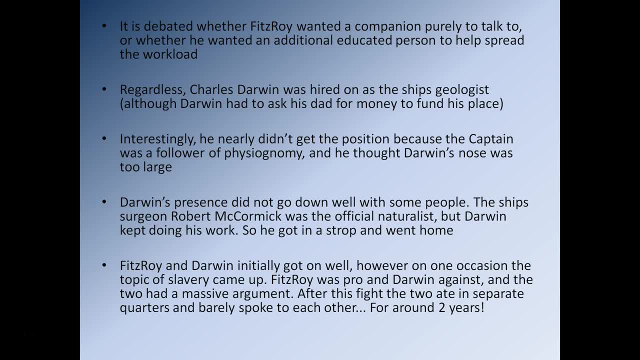 to or whether he wanted an additional educated person to help spread the workload. So at that point it would have been Fitzroy's responsibility and also the ship surgeon. you know Fitzroy's responsibility, especially to map the seafloor and to map the coastline. The ship surgeon would also. 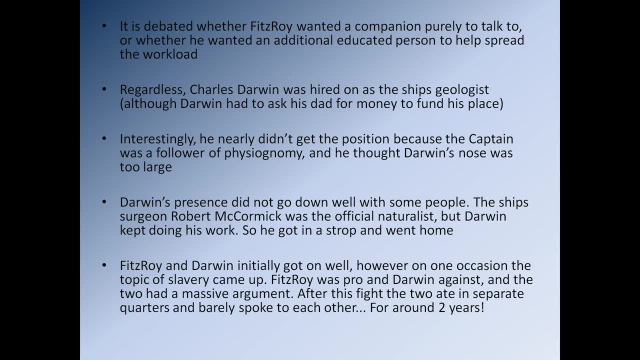 have had the responsibility of looking after the crew and also having to go on to land to collect, you know, animal samples, plant samples and rock samples. So you know both of them had a pretty heavy workload and having a third educated person on board would have helped to alleviate that. 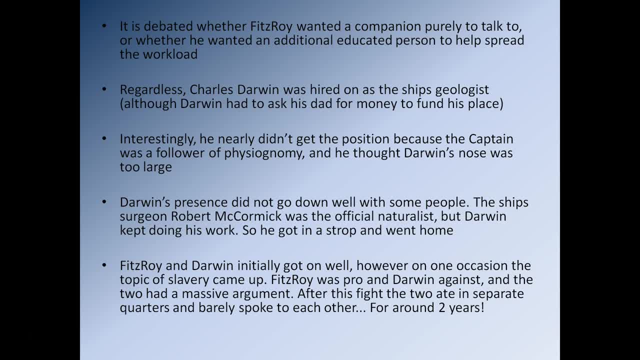 workload to some degree. So, regardless of why Darwin was hired, he became the ship's geologist. It's interesting to actually know that Darwin had to ask his dad for money to actually go on the voyage, So he wasn't actually a paid member of the crew, he was just there as a, you know, an additional person who had to pay his own way. 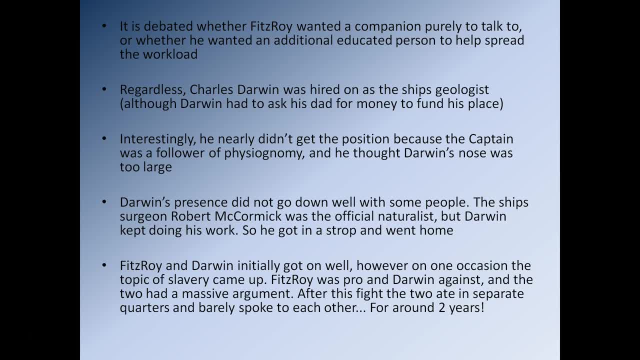 So, strangely, Darwin came close to nearly not getting the position, because Captain Fitzroy was a follower of physiognomy and so he thought that Darwin's nose was too large. So physiognomy essentially is the belief that you can, you know, view someone's personality or work out someone's personality by looking at their facial features. 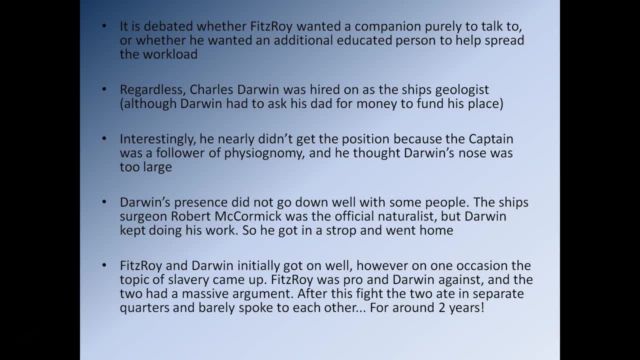 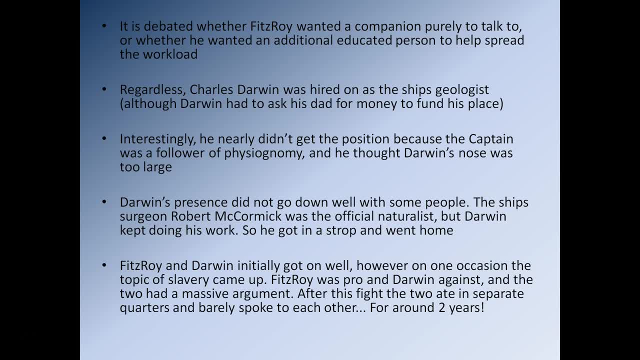 So Darwin's presence did not go down well with some people. So the ship's surgeon, a gentleman called the official naturalist, so it was his job to collect the animal samples, the plant samples and the rock samples. But of course Darwin, as the ship's geologist, kept doing his work. 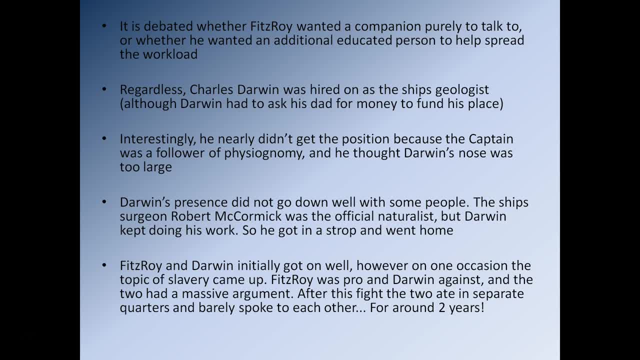 So eventually Robert McCormack got in a strop and Robert McCormack went home to England. So Fitzroy and Darwin initially got on quite well. however, on one occasion the topic of slavery came up and Fitzroy was pro-slavery, Darwin was against slavery and the two of them had a massive argument. 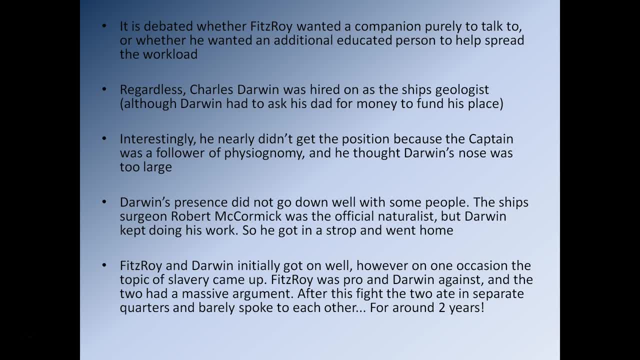 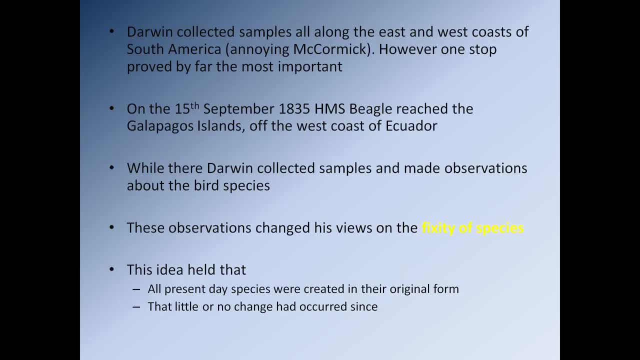 So after that fight, the two of them ate in separate quarters and barely spoke to each other for around 10 minutes. So Darwin collected samples all along the east and west coasts of South America and some, you know, along the way annoying McCormack. However, one stop proved to be by far the most important. 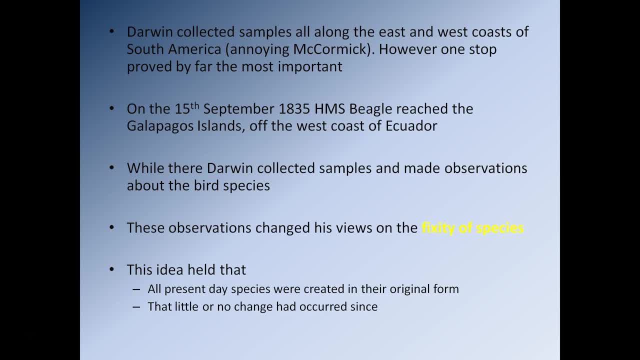 and that occurred on the 15th of September 1835, and that's when HMS Beagle reached the Galapagos Islands off the west coast of Ecuador. excuse me, So while there Darwin collected samples of the Galapagos Islands, he also collected samples of the Galapagos Islands off the west coast of Ecuador. 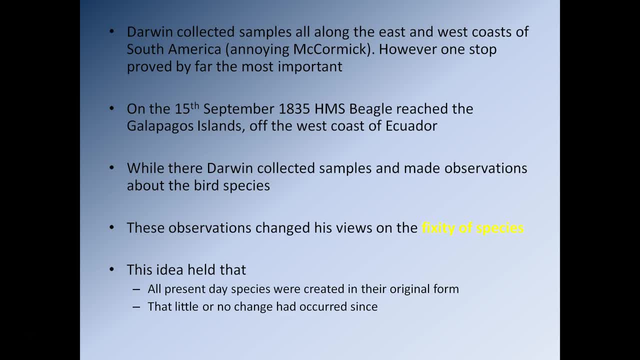 So these observations changed his views on the fixity of species. So what's the fixity of species? Well, the fixity of species is the idea that all present-day species were created in their original form and that, since their creation, little or no change has occurred. Essentially, it's the 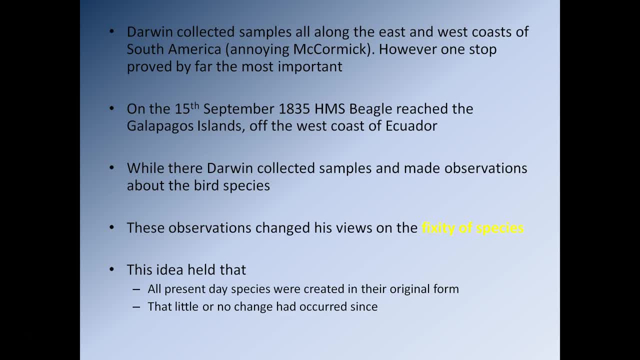 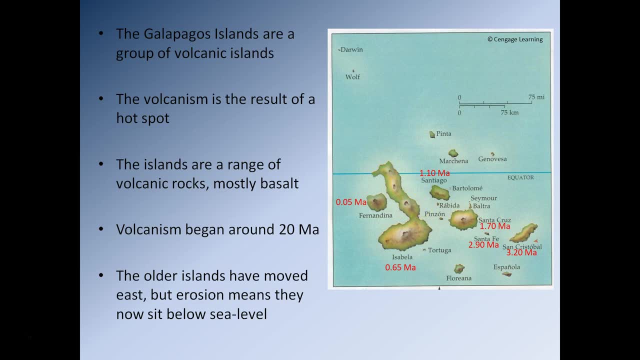 biblical view, Life was created and since then no real change has happened. So the Galapagos Islands have been created since the 15th of September 1835.. Galapagos Islands are a group of volcanic islands, as I said, that sit off the west coast of Ecuador. 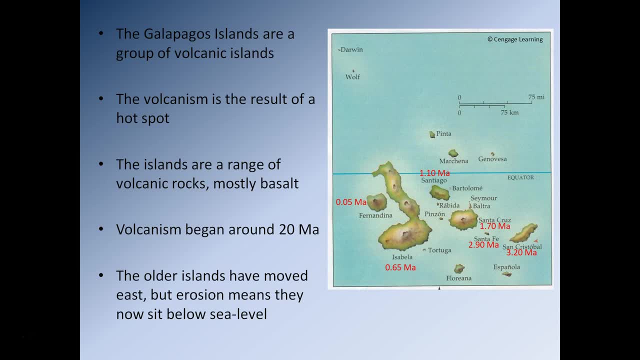 So the volcanism is the result of a hot spot and the islands are a range of essentially a range of different volcanic rocks, mostly basalt, And we know that the oldest islands, or should I say volcanism, began somewhere around 20 million years ago. So we can see over here- this is the picture of the modern Galapagos Islands. and next, 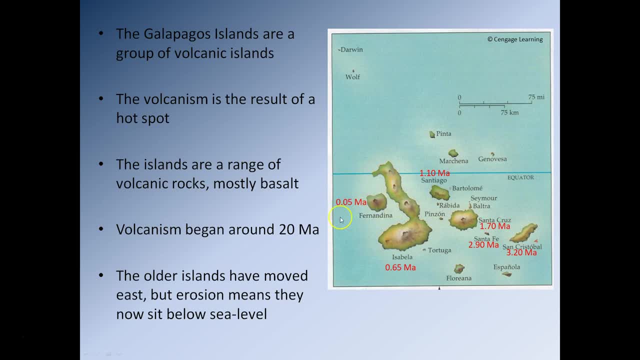 to it is the Galapagos Islands. Galapagos Islands are a group of volcanic islands that are a little bit older than 3.2 million years, So you can see that we're going from around you know, 0.05 million years over here. 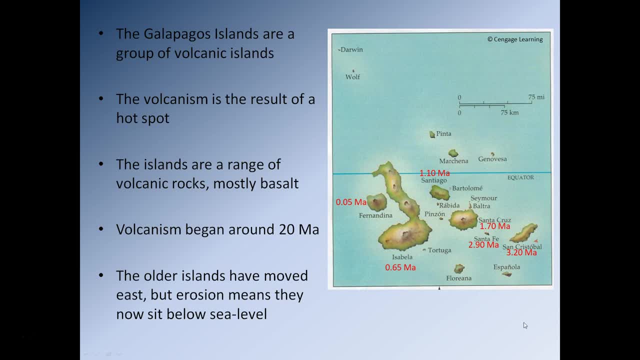 to 3.2 million years over here. So clearly the islands are getting older as we go to the east. So the islands that are even older than 3.2 million years are obviously off towards the east. So they're heading towards the west coast of South America where they will subduct under South America and be lost. 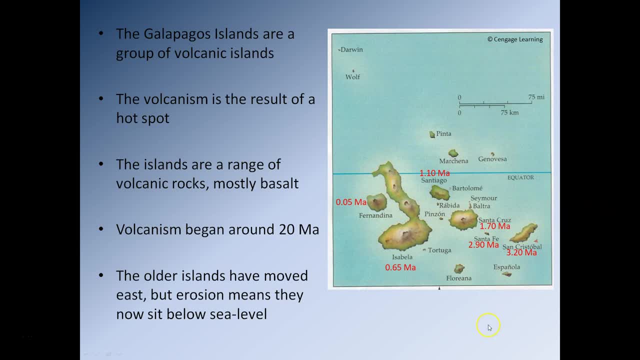 So what essentially is happening is the older islands are moving off towards the east, but of course we can't see the difference. But of course we can't see the difference. We can't see them anymore because they've been eroded down to the point where they now sit below sea level. 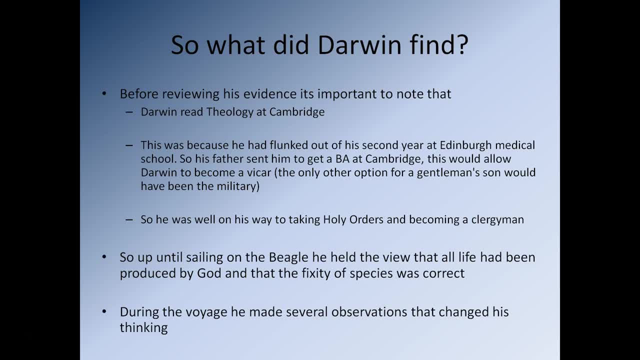 So what did Darwin find? Well, before reviewing his evidence, it's important to note that Darwin read theology at Cambridge University. So this was actually because he had flunked out of his second year at Edinburgh Medical School. So his father sent him to get a BA at Cambridge, and this would allow Darwin to become a vicar. 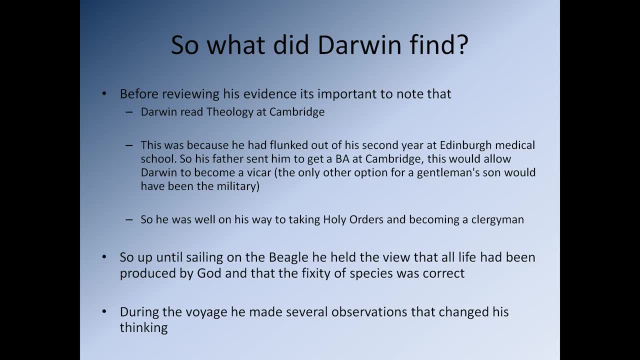 So the only other option for a gentleman's son at that particular point would have been some kind of career in the military, and Darwin really didn't want to get shot at. So essentially, Darwin was well on his way to taking holy orders and becoming a clergyman. 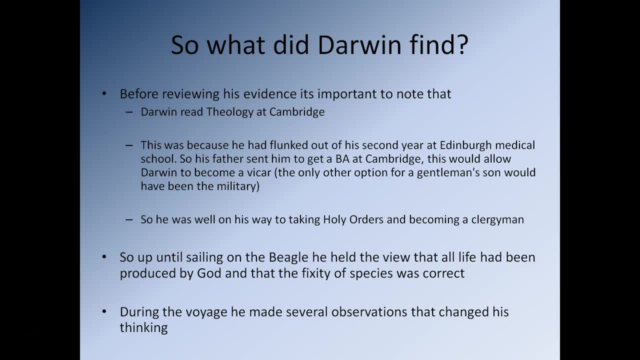 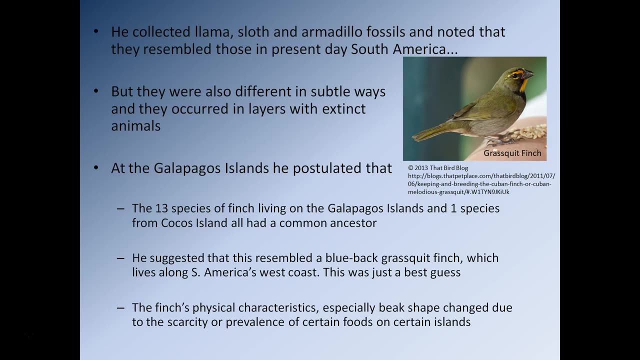 So up until sailing on the Beagle he had the view that the fixative species was correct and you know he followed essentially the standard viewpoint at that time. So during the voyage he made several observations that began to change his thinking on that subject. So as they were going down the the east coast of South America, he began collecting llama fossils. 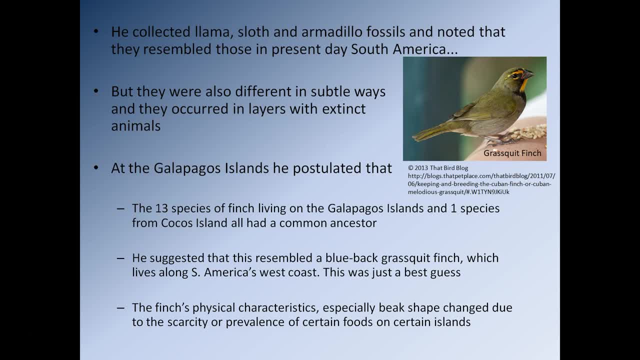 well, sloth and armadillo fossils and he noted that they resembled present-day species that exist in South America. But he also noticed that the fossils he were collecting were subtly different compared to the modern day examples. So there were these slight differences and he couldn't explain that. you know, because the fixative species said that. you know, animals didn't change. 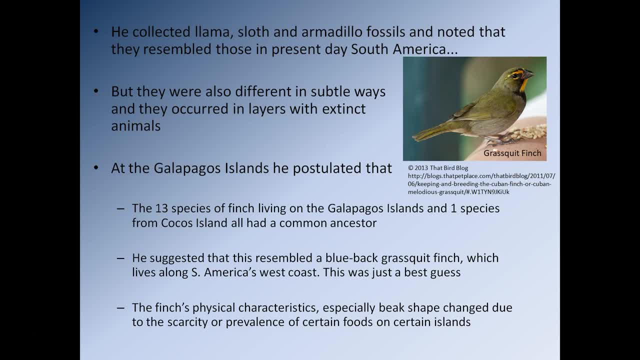 So at the Galapagos Canal he was able to see that there were different species of finches that lived on the Galapagos Islands. So in the Galapagos Islands he postulated that the 13 species of finch living on the Galapagos Islands 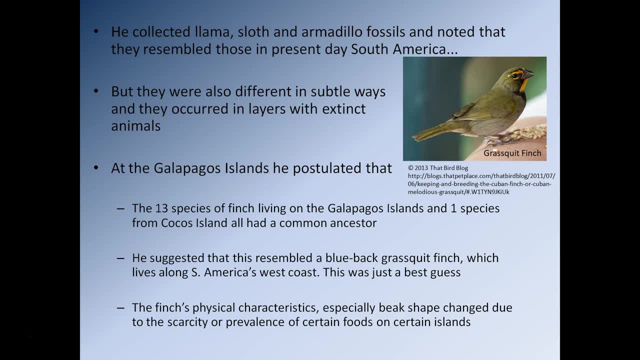 and one species on the nearby Cocos Island all had a common ancestor. He suggested that this resembled a blueback grass quit finch which lives along South America's west coast today, And essentially that was a best guess. it's actually pretty accurate guess. 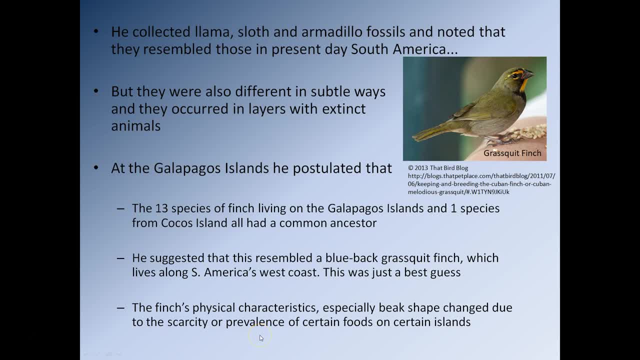 And this is one of the grass quit finches up here. that's what it looks like. So this is a very simple example of the fact that the size of the finches on the Galapagos Islands, especially beak shape, changed due to the scarcity or prevalence of certain foods on certain islands. 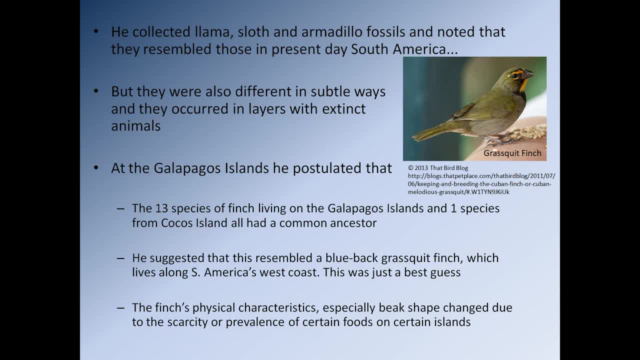 So what Darwin actually spotted was that, as he went from one of the Galapagos Islands to another, he saw that the finches on those islands changed, particularly when it came to beak size and beak shape, And these changes were essentially controlled by what the finches were eating. 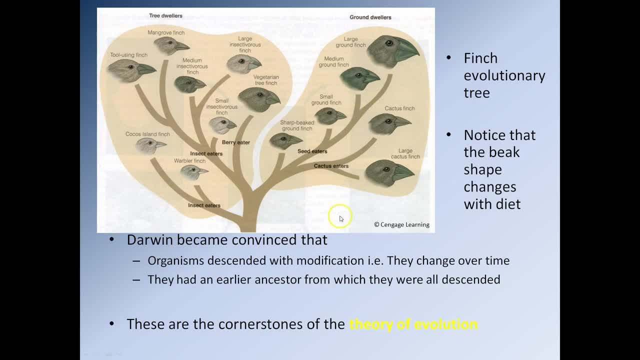 So let's look at this diagram here. So this, this is essentially is the finch. So this is essentially the finch eating the evolutionary tree for the Galapagos Islands. So we're going to note how the beak size and beak shape is going to change with diet. 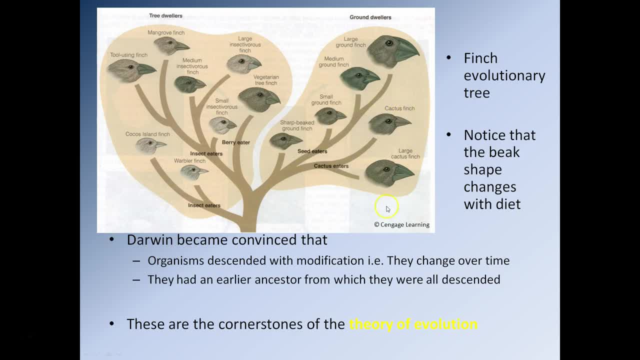 So you can see that this diagram is actually split into several different groups. So over here we have the cactus eaters, here we have the seed eaters, we have the berry eaters. up here we have the insect eaters. over here and we have more insect eaters down here. 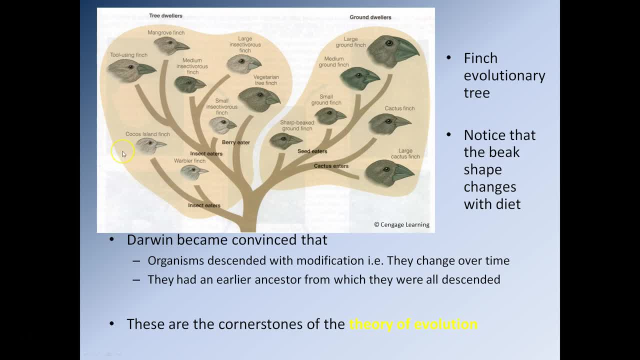 So, depending on what the birds are eating, that's going to affect the beak shape. So let's look at the cactus, So let's look at the cactus eaters, for instance. So you know, depending, you know if your cactus has a very thick, heavy, you know- outer skin. 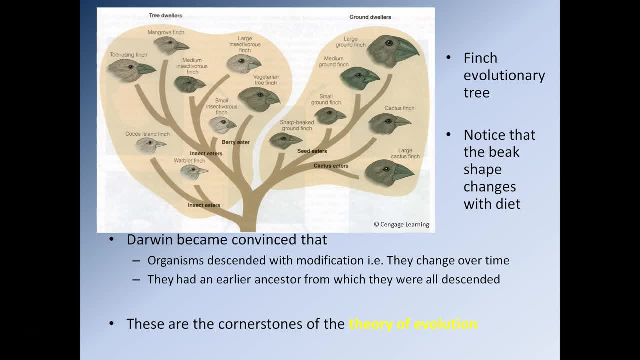 so you know it's very difficult for the bird to obviously get through that skin to the, to the part, you know, to the core of the cactus, which is what it wants to actually eat Essentially. what you need is a big, strong beak, So birds that have to essentially eat their way into very, very thick. 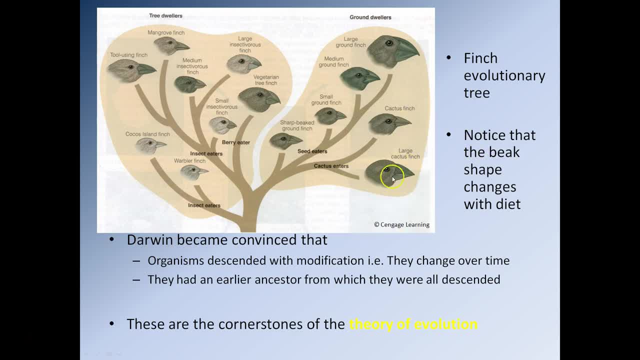 leathery cactuses. cacti have to have big, strong beaks. So that means they have to have these very strong, short stubby beaks And that obviously means is the beak gets larger, they obviously the head has to get larger to support it. 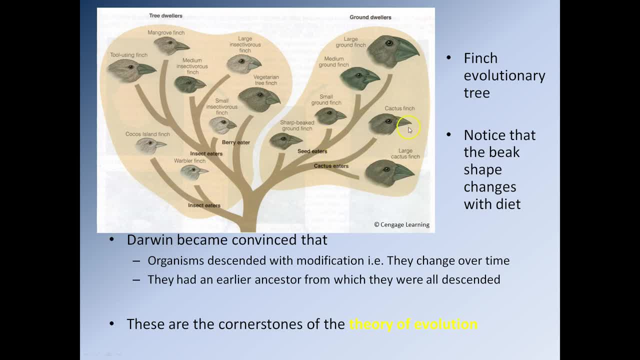 So these finches tend to have quite large bodies. Finches, on the other hand, that tend to be eating cactuses that have, you know slightly. you know, weaker hides requires a little bit less effort. well, they tend to have a beak that's essentially a bit smaller. 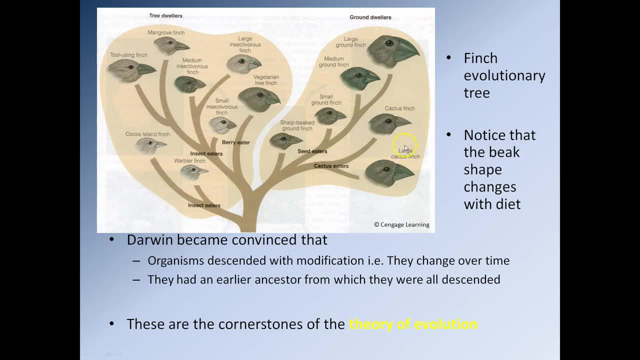 a bit longer and a bit narrower And that's more designed for, kind of like, trying to puncture into the cactus to get to the stuff underneath Now. then we have the seed eaters, So depending on how big and hard the seeding question is. 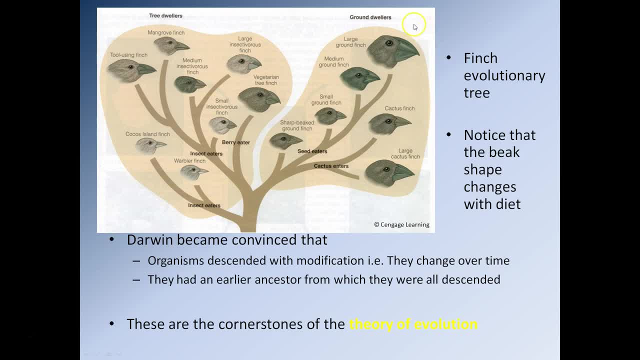 well, that's obviously going to affect the shape of the beak. So birds that have to eat big, hard seeds- well, they need big, powerful beaks. Birds that have to eat smaller, more easily broken up seeds- well they can have smaller, weaker beaks. 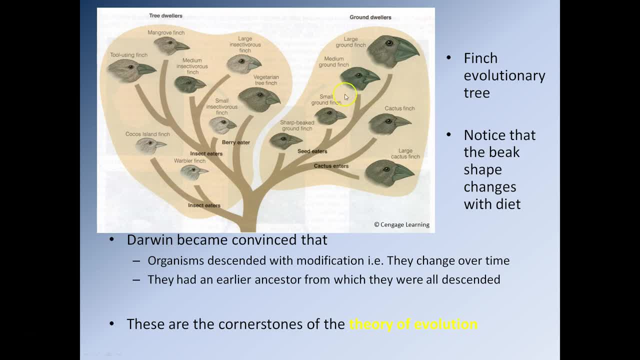 So essentially, depending on whether you know, the seeds were large, small, hard or soft, essentially, once again, we can see the beak shape was changing depending on those requirements. Obviously we have a whole range of insect eating finches over here And once again the beak is going to vary depending on what type of insect they're eating. 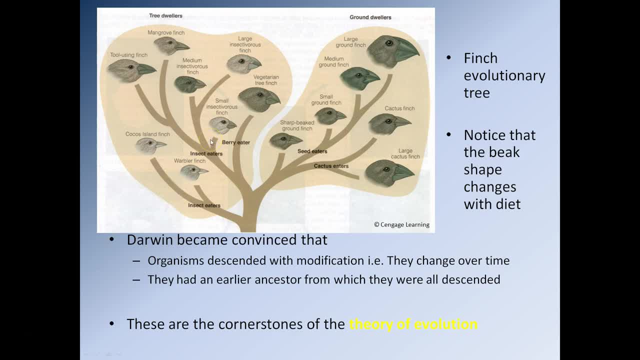 So if the insect is just, you know, walking along, you know the outside of a tree, well then it's not really too difficult to get the insect, And so, you know, beak shape is relatively normal. Now, if the animal in question, however, lives underneath the bark of a tree, let's say 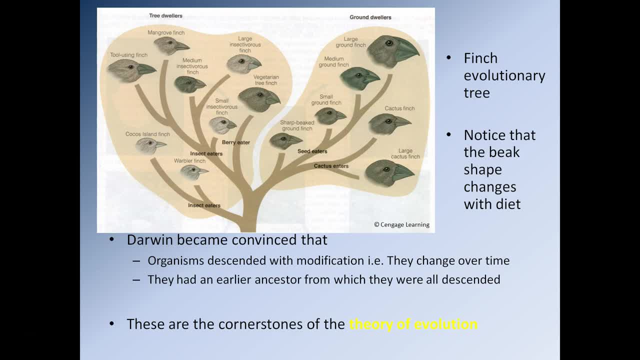 or let's say, in a tree. well, in that case the finches have to take on a different approach. They have to have a long, slender beak so they can get into the burrows made by the insect and pick the insect out. So, depending on you know where the insect lives, that's going to affect their beak shape. 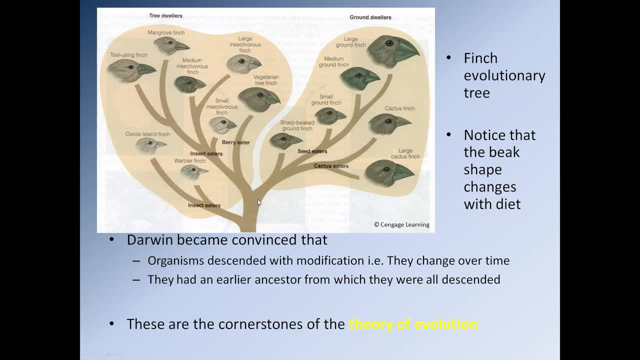 So, as you can see, that the variability in essentially the food source on each of the islands has had a direct effect on the beak shape of the finches that exist on those islands. So this led Darwin to become convinced that organisms descended with modification. 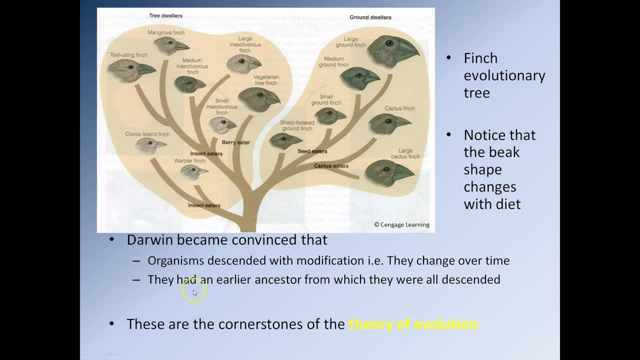 So an organism will change over time And they had an earlier ancestor from which they were all descended. So Darwin realized, you know, they were all you know, they all had these variations in terms of their beaks And, obviously, head size. obviously the bigger the beak, the larger the head. 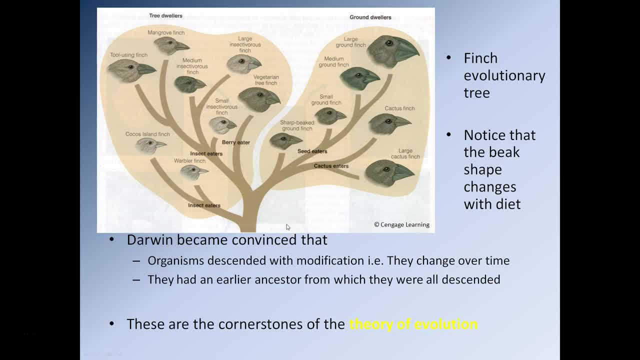 But when it really came down to it they were, all you know, remarkably similar. apart from that, So Darwin postulated they had a- you know, a common ancestor down here And from that common ancestor you had divergence, producing lots of distinct finch species, And essentially that's the cornerstone of the theory of evolution. 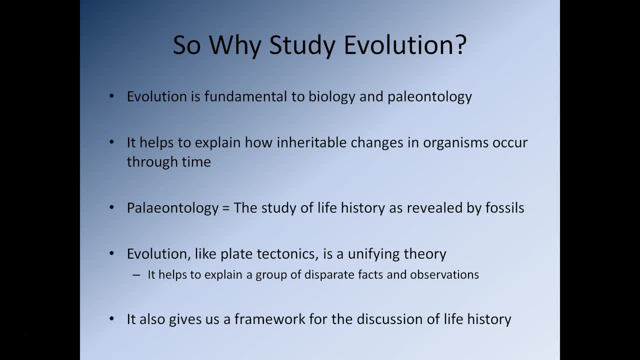 So, obviously, why study evolution? Well, evolution is fundamental to biology and paleontology, So it helps to explain how inheritable changes in organisms occur through time. So an inheritable change is a change is some kind of feature that a parent can pass on to its offspring. 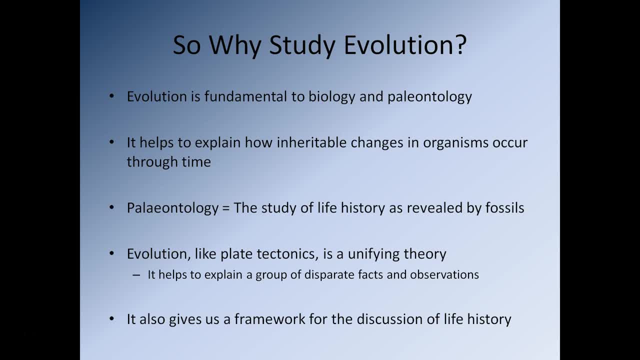 So paleontology is, of course, the study of life history as revealed by fossils. So evolution, like plate tectonics, is what we refer to As a unifying theory. it brings together lots of pieces of evidence And once you have the explanation, once you have the theory of evolution, 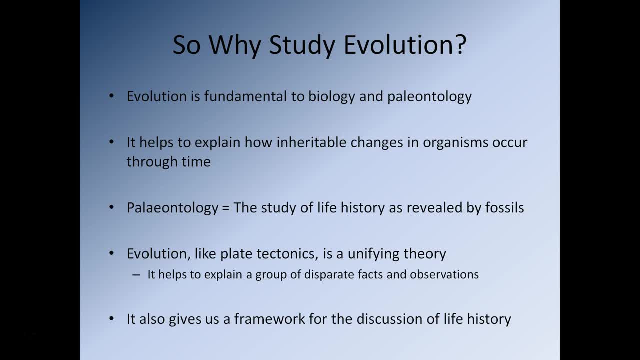 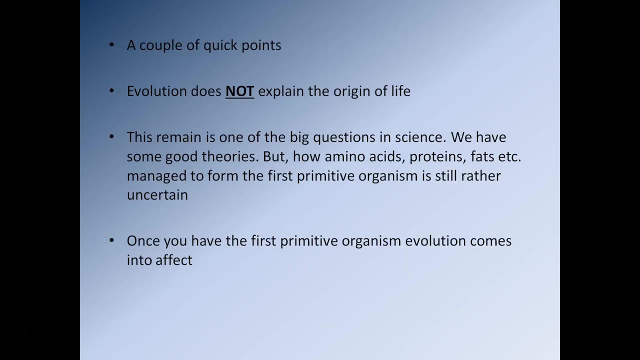 All these disparate pieces of evidence can be explained under the under the, under the umbrella of that particular theory, in this case evolution. So it also gives us a framework for the discussion of life history. So quick couple of points. So evolution does not explain the origin of life. 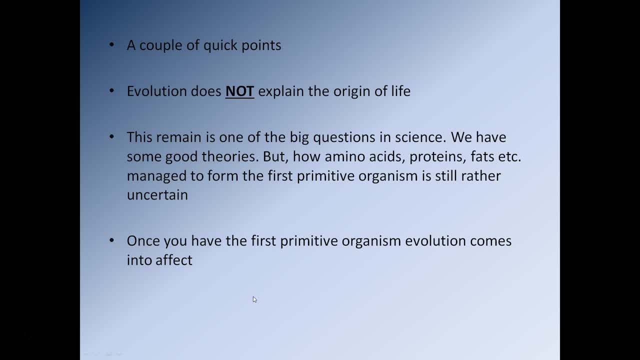 That's one of the key things we have to remember. So you know this. you know, the origin of life remains one of the big questions. We have some good theories, But how amino acids, proteins, fats, etc. manage to form the first primitive organisms is still rather uncertain. 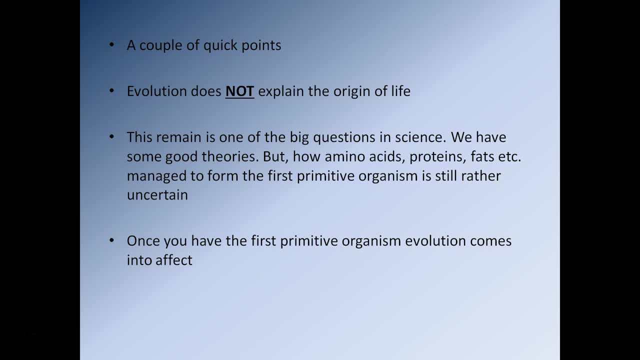 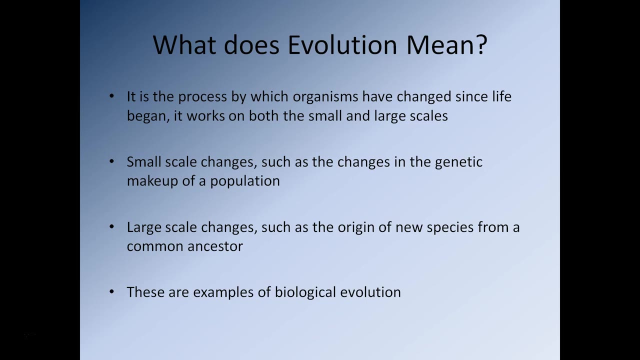 And we have to be honest about that. So, of course, the important thing is this: Once we have the first primitive organism, evolution then comes into effect. So what does evolution actually mean? So it is the process by which organisms have changed since life began. 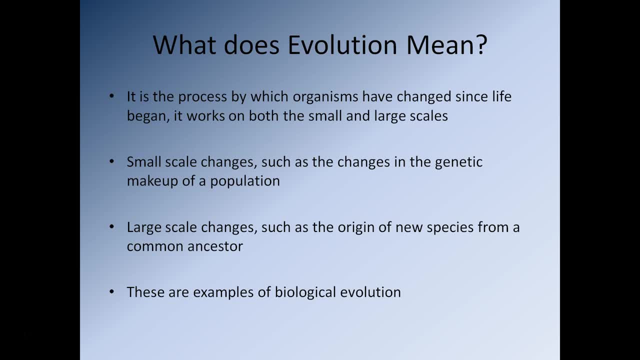 And it works on both large scales and small scales. So small scales, changes Such as changes in the genetic makeup of the population, can occur, Whereas large scale changes, such as the origin of new species from a common ancestor. So you know, sometimes you can get very minor changes in the population. 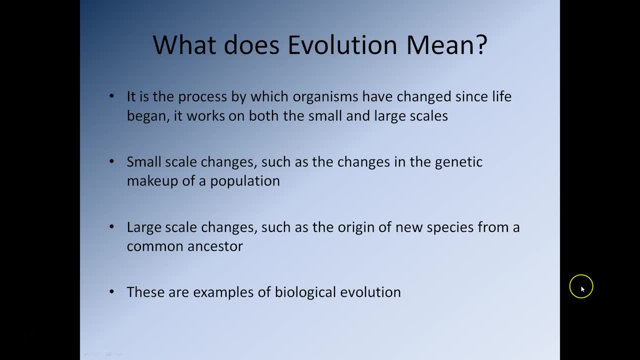 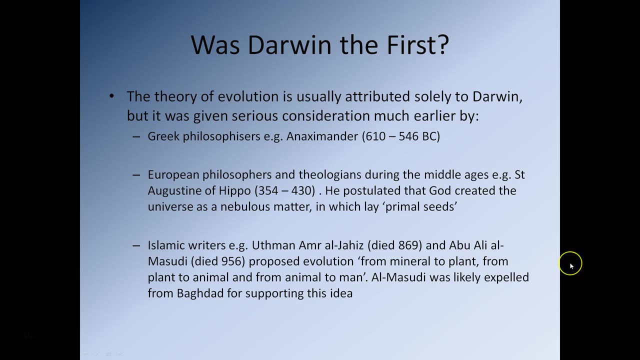 And in some cases you can get very major changes, And essentially major changes lead to the formation of a new species. So these are examples what's referred to as Biological evolution. So was Darwin actually the first to propose evolution? Well, the theory of evolution is usually attributed. 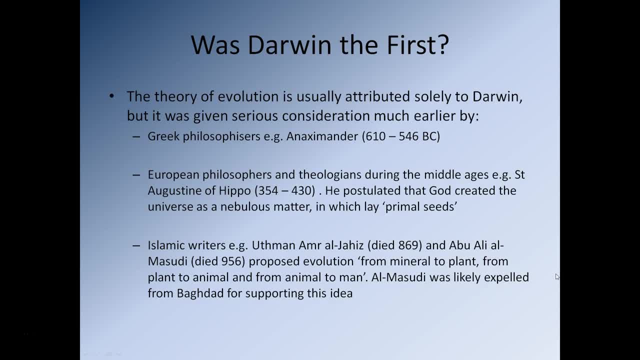 Sorry, it's usually attributed solely to Darwin, But it was actually given serious consideration much earlier. So the first you know people to actually, you know, think about Where did life come from and is life, you know, changing over time, Were the Greek philosophers. 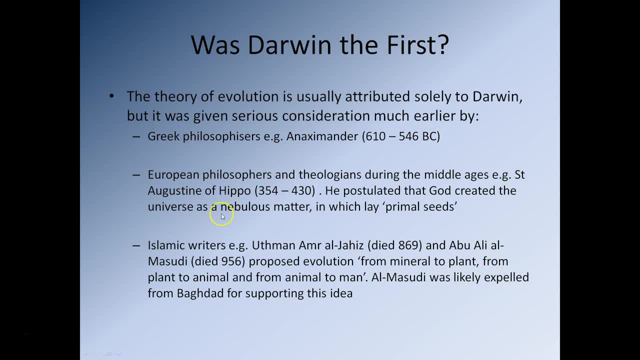 So the Greek philosophers, you know, postulated on the problem. Obviously, then later on, we have European philosophers And theologians during the middle ages, like Augustine of Hippo. So he postulated that God created the universe as a nebulous matter In which lay primal seeds. 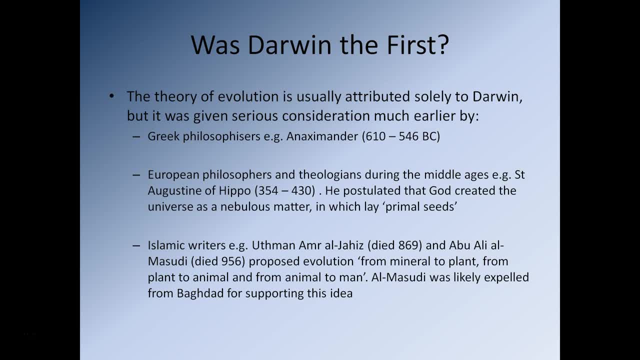 So essentially, what he was saying was is that, You know, depending on the exact conditions, Certain primal seeds would activate and certain animals would appear. Essentially, it meant that animals were constantly appearing and dying out through time. So we then had Islamic writers, And I do apologize for my terrible pronunciation of these names. 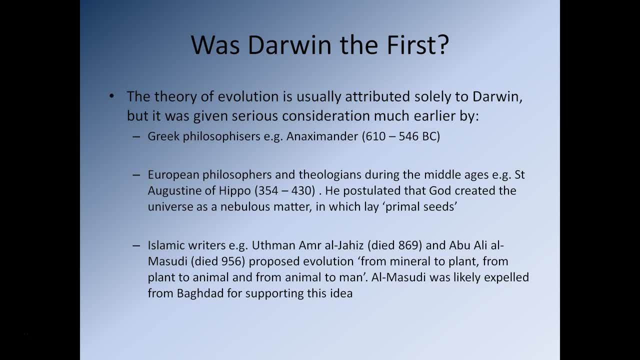 We have Uthman al-Aziz and Abu Ali al-Masadi, And they proposed evolution from mineral to plant, From plant to animal And from animal to man. And this idea was actually so controversial That al-Masadi was actually likely kicked out of Baghdad for supporting that particular idea. 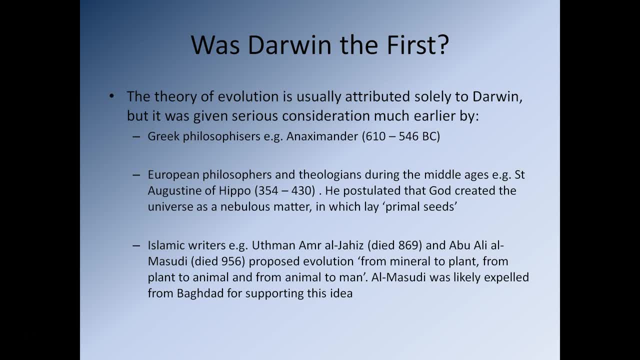 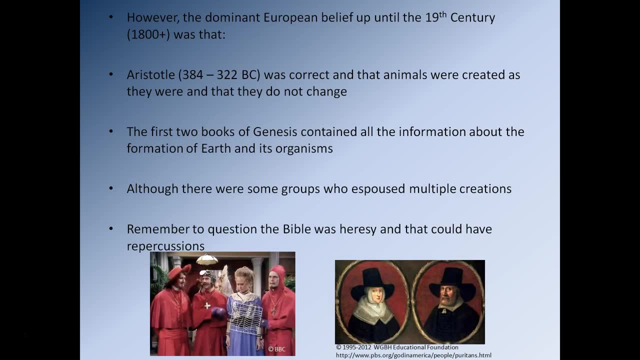 So there were, you know, there were people that did actually think about, you know, evolution. They were postulating, Whether you know, Life was actually changing through time. However, the dominant belief in Europe up until the 19th century Was that Aristotle was correct. 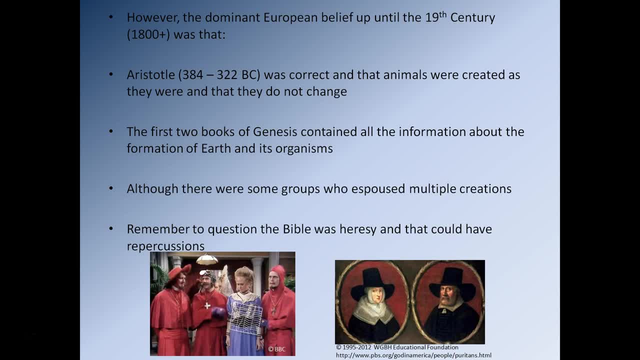 And Aristotle essentially said that animals were created as they were And they do not change. So essentially that means the first two books of Genesis contain all the information About the formation of the earth and its organisms that you require Now. there, of course, were some groups that you know espoused multiple creations. 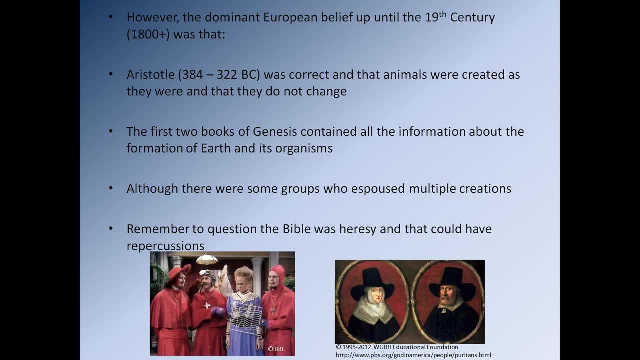 To explain. you know Why you got some animals dying out and some animals appearing, But you know when it really came down to it. People who didn't, you know, have an idea of evolution or an idea like evolution, Essentially kept that idea to themselves in most cases. 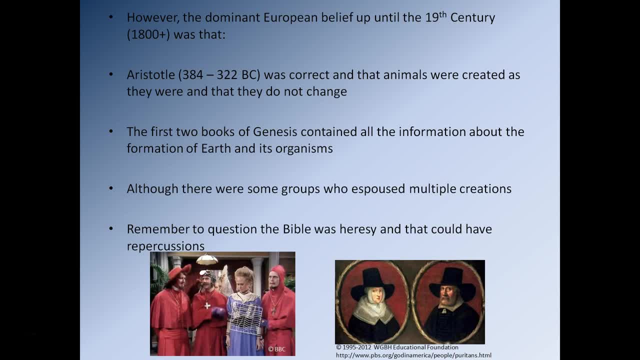 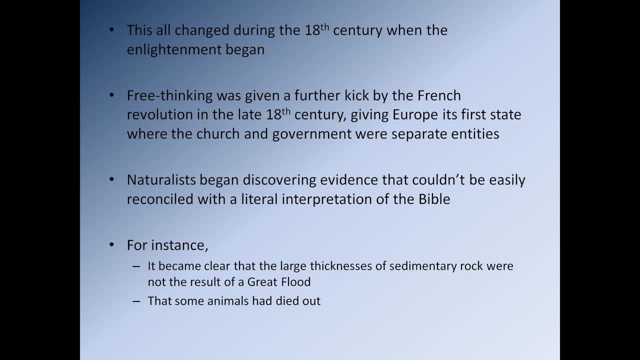 Because to question the bible was heresy And that could have very serious repercussions. So this all changed during the 18th century when the enlightenment began. So the enlightenment was given a further kick by the French revolution In the late 18th century. 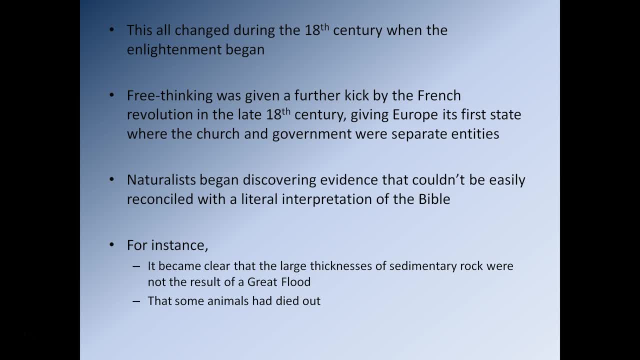 So what this did is it created Europe's first state Where the church and the government were separate entities. So you know, before then, you know, the church and the government had to essentially work as one. But once the French revolution happened, You had a government that was working independently of the church. 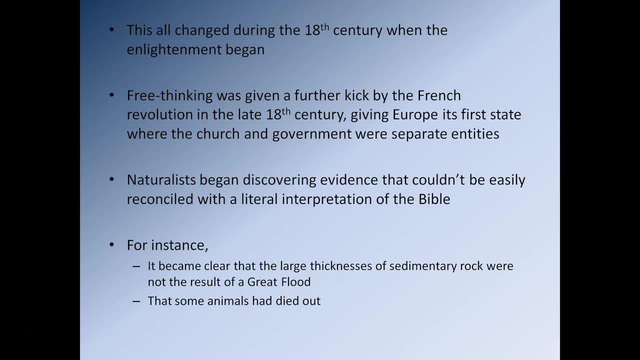 And therefore the government could fund scientific works that it decided were of value. So naturalists began to discover evidence that could be easily That- sorry, that couldn't be easily- reconciled with a literal interpretation, The bible. so, for instance, it became clear that the large thicknesses of sedimentary rock that we see 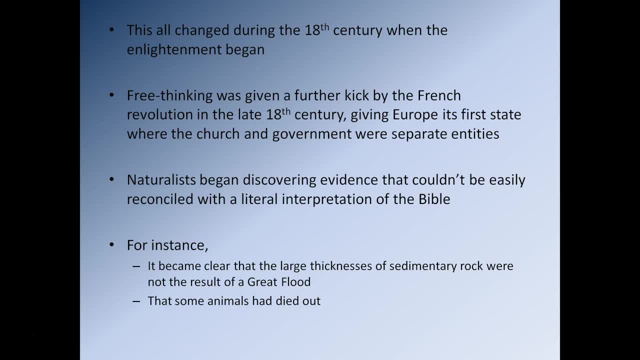 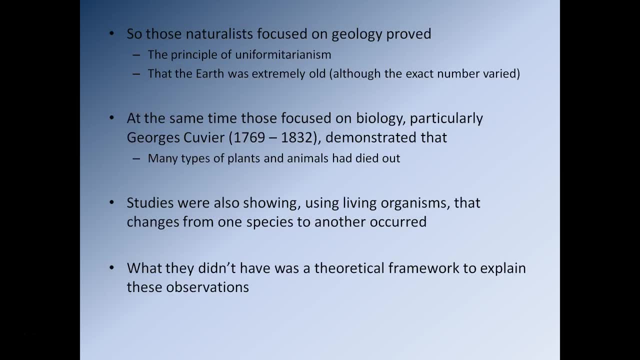 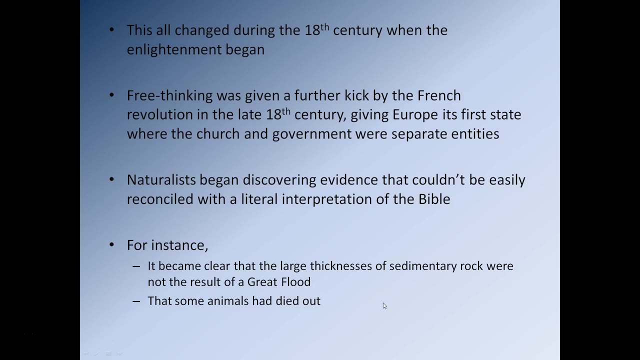 Could not have been created by a single great flood. It also was becoming more and more clear that some animal species had died out. You know that's a real problem if you assume that you know animal species You know don't change. if animal species aren't changing, then they shouldn't be dying out. 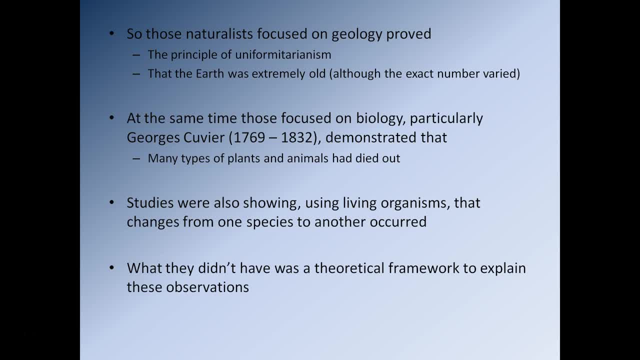 So naturalists that focused on geology. They started the principle uniformitarianism. If it's happening today, it's happened in the past, And they also began to realize the earth was extremely old. Of course, we've already touched on this already in some earlier lectures. 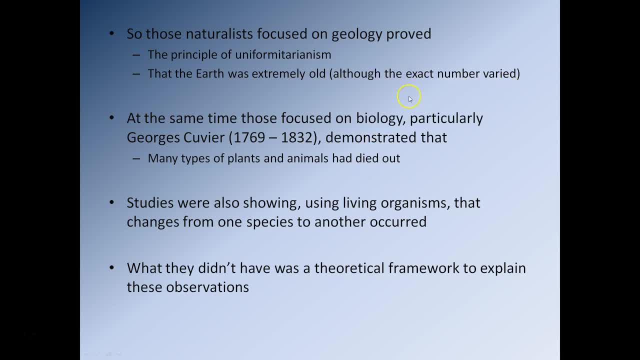 And we know that. you know, when they were trying to calculate this age, They came up with quite a large range of possible options. So at the same time, there were people who were focused on biology, Particularly Georges Cuvier, And he demonstrated that many types of plants 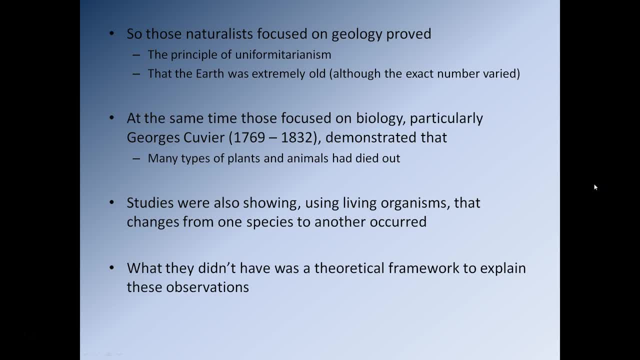 And animals had died out. So he was making observations about plants and animals, You know, whereas geologists were making observations about animals, you know from the fossil record, And both groups were realizing that, you know, some animal species, essentially, over time, had disappeared And then new animal species had appeared. 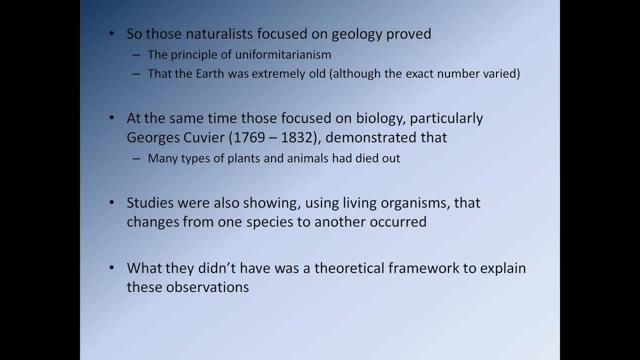 So studies were also showing, using living organisms, that changes from one species to another occurred. So, of course, at this, you know, this is the kind of point. when we had selective breeding Beginning to become, you know, important, It came to, you know, things like cattle and dogs, you know. 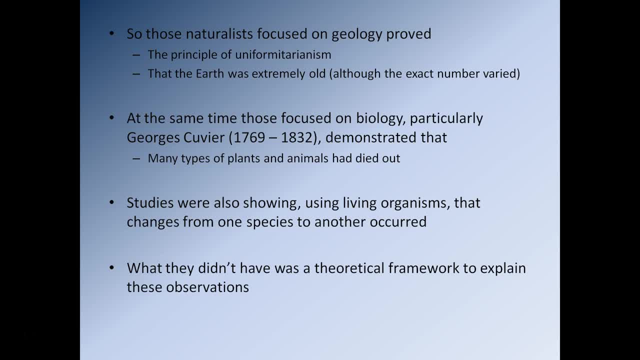 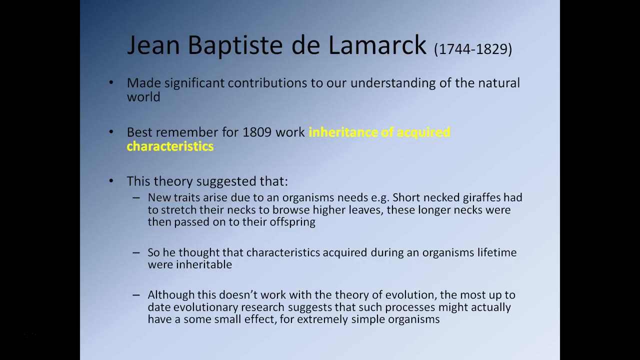 So all of a sudden, it began to become clear that you know, by selecting certain species, By selecting certain traits, you could make significant changes to the physical appearance, For instance, of a species. So what they didn't have was a theoretical framework to explain these observations. 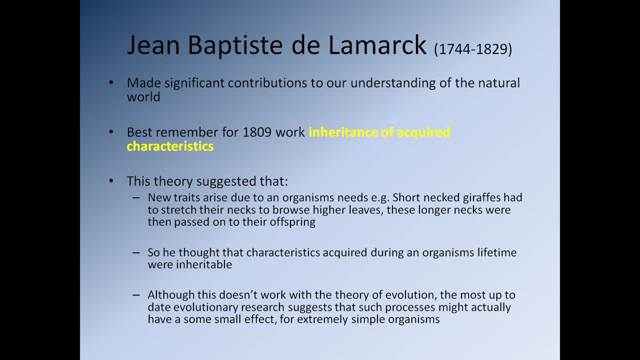 So this brings us on to Jean-Baptiste Delamarque, And he made significant contributions To our understanding of the natural world. So he's best remembered for his 1809 work, inheritance of acquired characteristics. So Delamarque's theory suggested that new traits arise due to an organism's need. 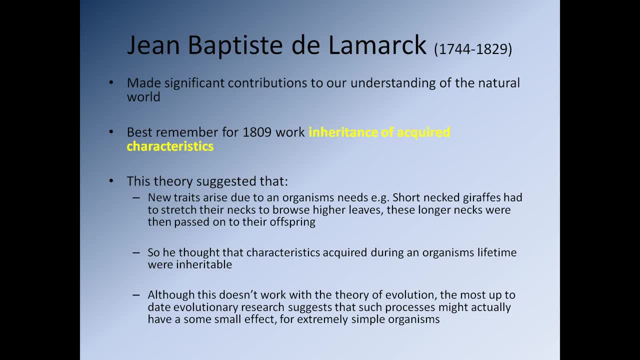 So he was saying that essentially, if you imagine a situation where you had lots and lots of short necked giraffes And there was some kind of change in the environment And it meant that all the really good leaves started growing right at the tops of the trees- 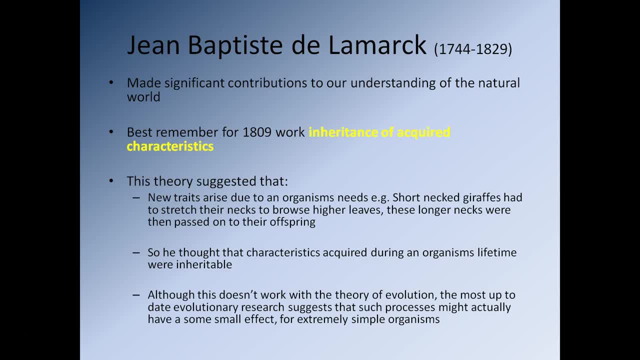 And so, essentially, in order to reach those, you know, leaves right at the top of the trees, The giraffes really, really, really had to stretch their necks And, in the process of stretching their necks, to try and reach these leaves at the top of the tree, 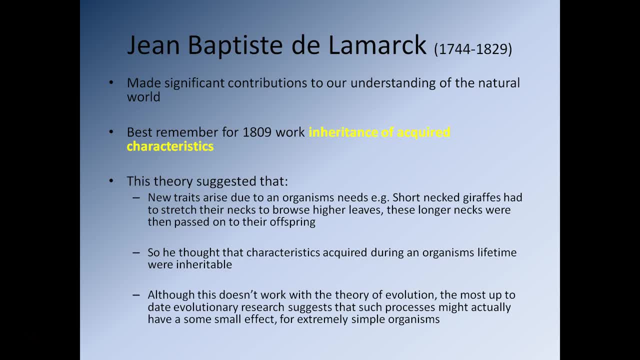 Their necks became longer And then they could pass on that characteristic to their offspring, So they would produce offspring that naturally had long necks, So they could reach the the leaves at the tops of the trees. So Delamarque was essentially saying that the characteristics that were acquired 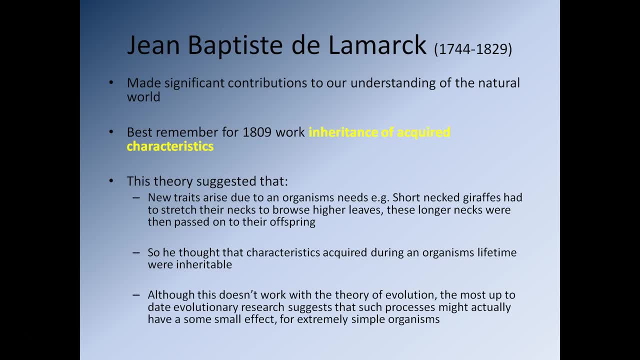 Especially the characteristics an animal had Were acquired during an organism's lifetime, And that they were inheritable And could therefore be passed on to their offspring. Now, although this doesn't work with the theory of evolution, The most up-to-date evolutionary research suggests that such processes might actually have some small effect. 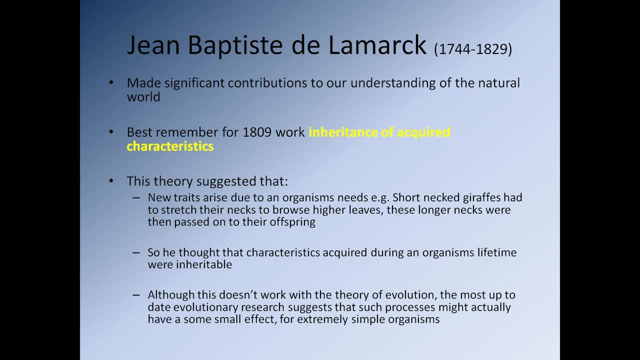 For extremely simple organisms, Extremely simple organisms, But when it really comes down to it, Complex organisms like you know: giraffes, humans, birds, etc. This particular idea doesn't actually work. But what, essentially what Delamarque is doing Is he's realizing that over time, characteristics are changing. 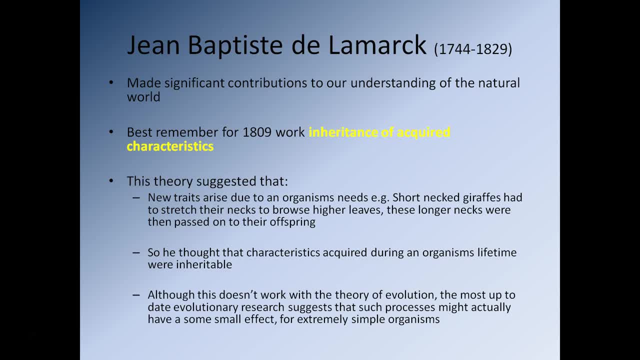 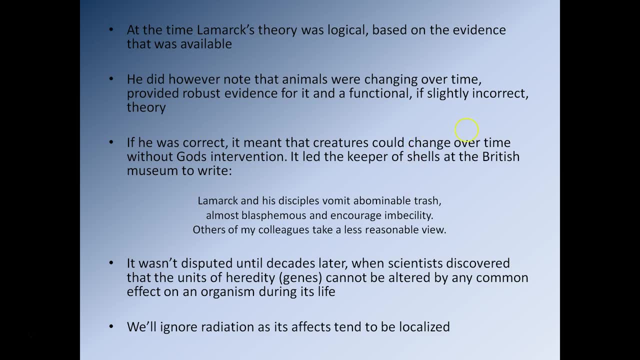 And those characteristics are appearing or disappearing Depending on environmental stresses. The organism is changing for some reason, So at the time, Delamarque's theory was logical, based on the evidence that was available. He did, however, note that animals were changing over time, as I said. 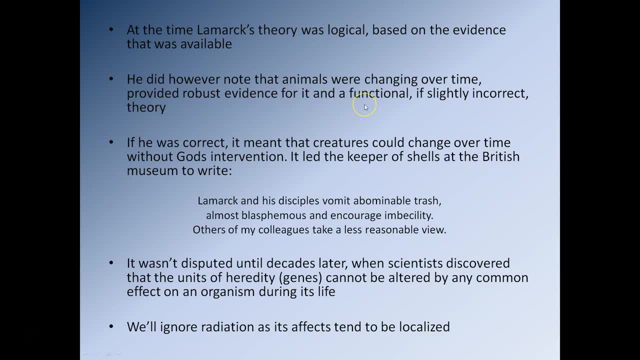 And he also provided robust evidence for this, And his idea was functional, if slightly incorrect. So if he was correct, It meant that creatures could change over time without God's intervention, And it led to the Keeper of Shells at the British Museum writing. 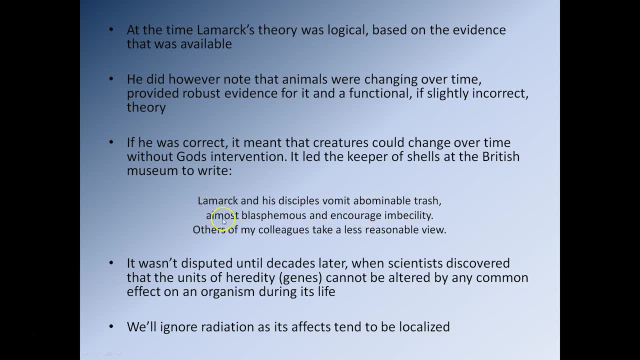 Delamarque and his disciples vomit abominable trash, Almost blasphemous, and encourage imbecility. Others of my colleagues take let's try this again. Others of my colleagues take a less reasonable view. So essentially He's saying that Delamarque's ideas are essentially complete and total rubbish. 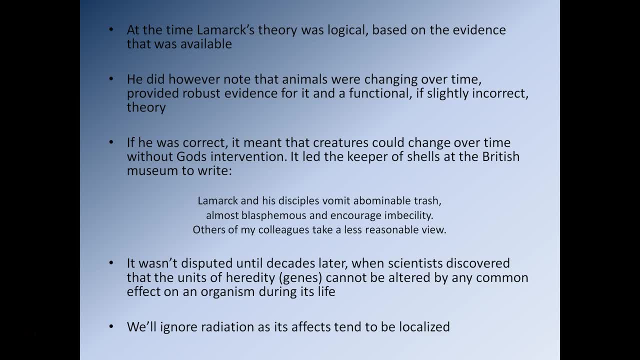 And that some of his colleagues take an even stronger view on that particular idea. So essentially, his ideas weren't by no means popular. So it wasn't disputed until decades later, When scientists discovered that the units of hereditary information, genes- Cannot be altered by any common effect on an organism. 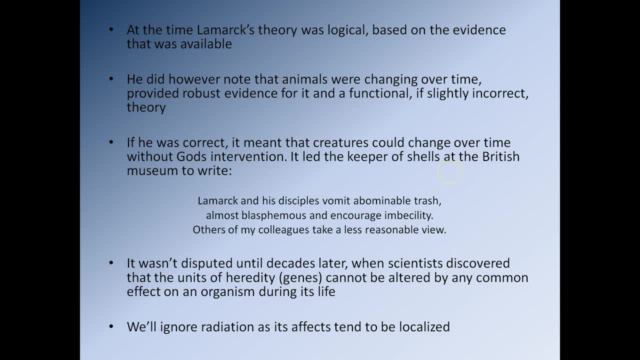 During its lifetime. So essentially, Delamarque's ideas made sense until we knew about genes. Once we knew about genes and DNA, Then all of a sudden You know how these traits were passed on from parents to offspring- Essentially became far clearer. 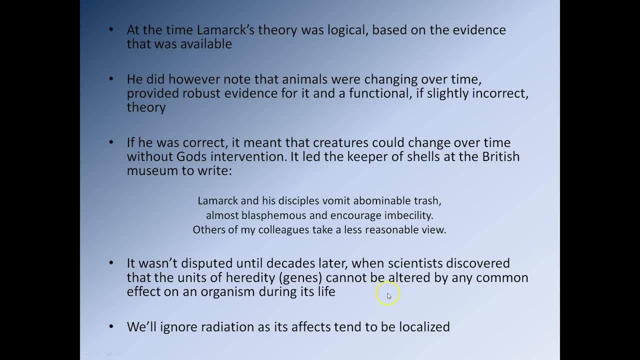 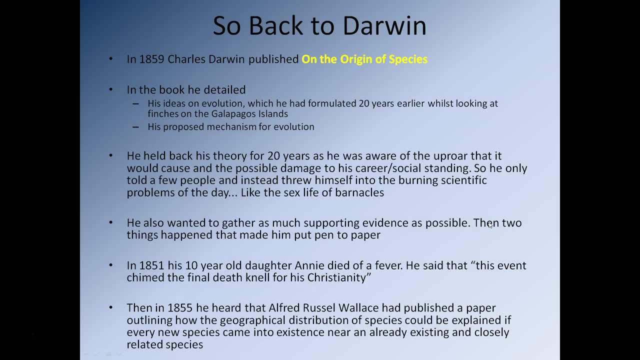 So obviously, in terms of you know, changes to genes during the lifetime of an organism, Well, we'll ignore radiation for now. So anyway, back to Darwin. So in 1859 Darwin published on the origin of species And in his book he detailed his ideas on evolution. 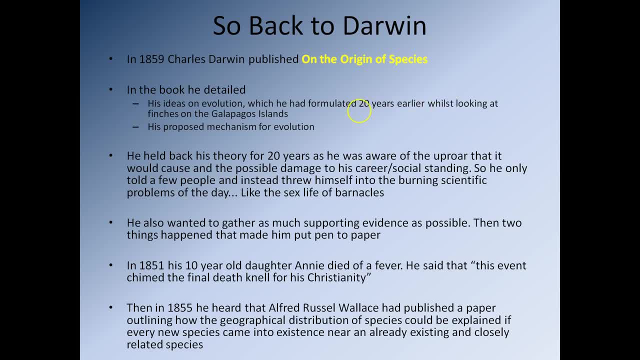 Which he had formulated 20 years earlier. whilst looking at the finches on the Galapagos Islands, Note that number: 20 years. It took him a very long time to actually publish his work And within the book he also proposed a mechanism for evolution. 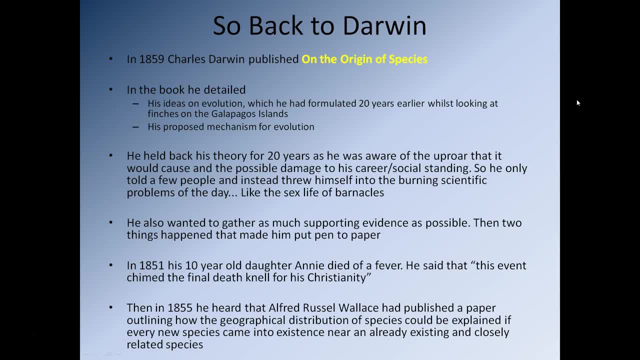 So why wait 20 years? So he held back his theory for 20 years as he was aware Of the uproar that it would cause And the possible damage that it that would do to his career and social standing. So when Darwin came back to the United Kingdom, He married, and he married very, very well. He married a woman with a lot of money And so he became essentially, you know, quite a significant person in social circles, And so he didn't really want to damage his standing in social circles. You know, people might not want to talk to him. 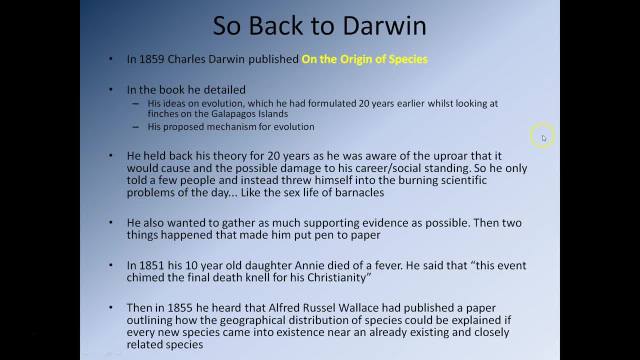 Have a dinner parties, etc. So So he only told a few people about his idea And instead he threw himself into you know other burning scientific problems of the day, Like the sex life of barnacles. So the other reason why he waited so long: 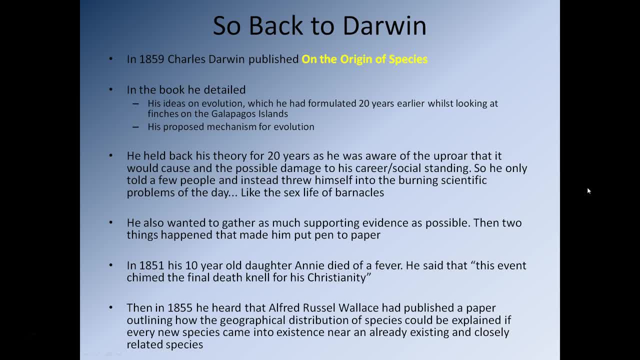 Is. he also wanted to gather as much supporting evidence as he possibly could. He knew that if he was going to publish this work, It was going to cause a lot of- you know, a lot of uproar And therefore, if he knew he was going to tell people about it. 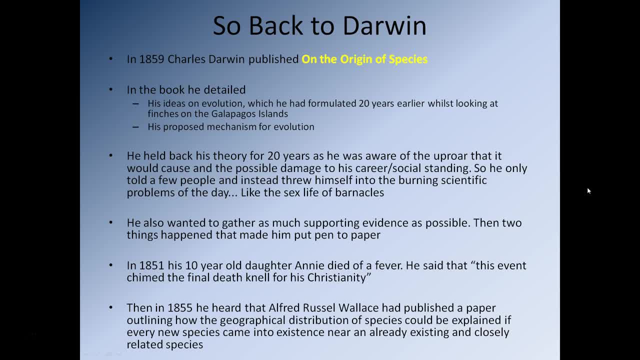 You know, he had to have as much evidence to defend himself as he possibly could. So in 1851 his 10 year old daughter, Annie died of a fever, And Darwin said that this event chimed the final death knell for his Christianity. 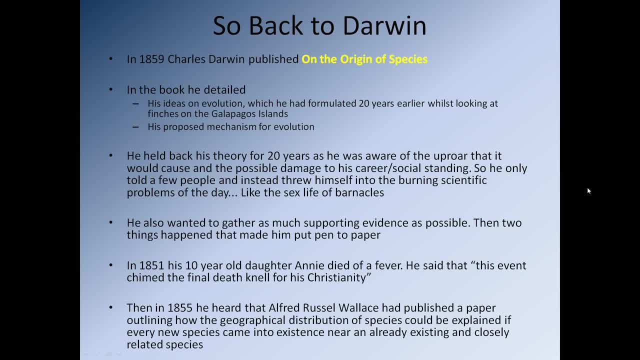 So from this point on, Darwin, you know, was no longer really worried about the feelings of his friends And he was just going to go for it. So another spurring factor was that in 1855 he heard the gentleman called Alfred Russell Wallace Had published a paper outlining how the geographical distribution 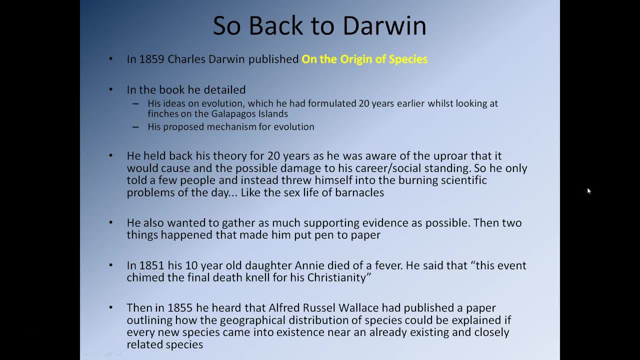 Of species could be explained if every new species came into existence Near an already existing and closely related species. You're sitting there thinking: What am I saying? Well, Wallace was working in Southeast Asia And the area of Southeast Asia he was working in. 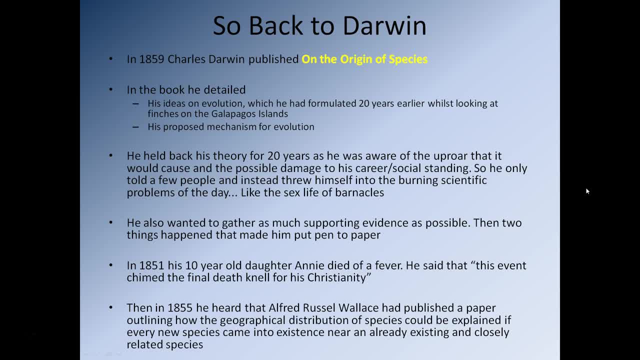 Had lots of very, very deep river valleys, And these deep river valleys were essentially separated by small mountain ranges Or at least very, very big hills, And so that meant that it was very, very Difficult for animals from one one of these valleys. 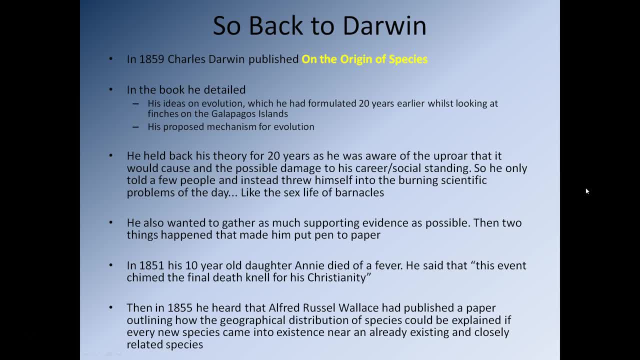 To make it over these mountains, slash hills into the other valley, So essentially, each of these valleys was isolated from the next valley along, And so what Wallace realized was that if you went from, If you had an animal, that were turned up in Valley A. 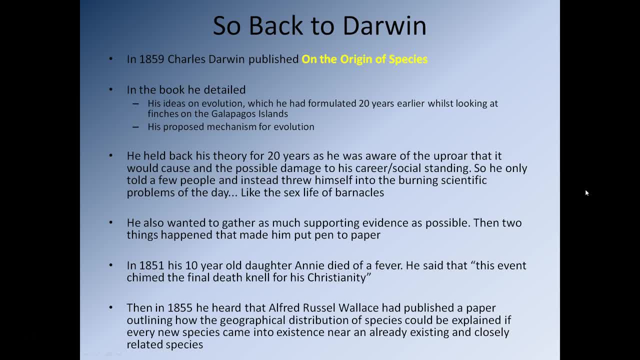 And you went to Valley B, You could see the same animal, but it would be slightly different. If you then went from Valley B to Valley C, You would have the same animal, But it would be even more different compared to the animal in Valley A. 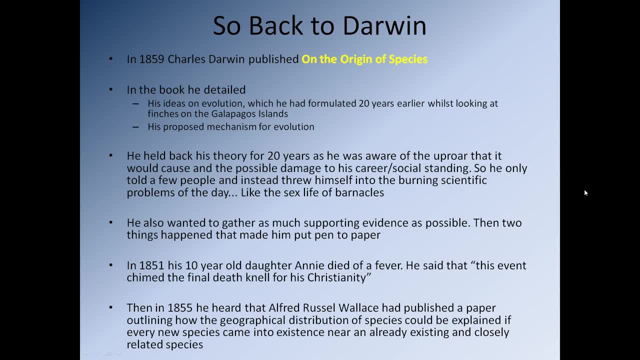 Go to Valley D, You would see approximately the same animal, But it would be even more different to the animal that initially started in Valley A. So each time you went along, you know the valleys. Essentially, you would see animals become more and more different. 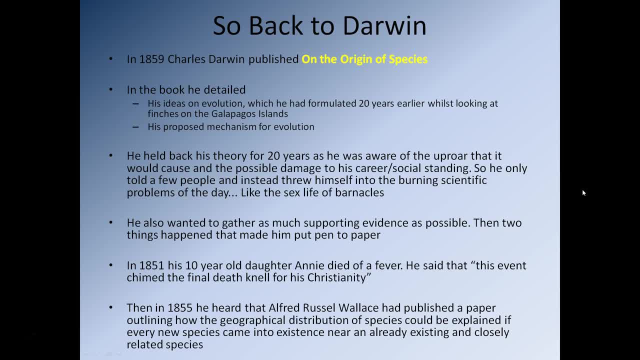 From the animal in the first valley, And so he began to realize that, you know, these organisms were adapting To the environment in each of the valleys And therefore, as they adapted to the environment in each of the valleys, They began to take on new body shapes. 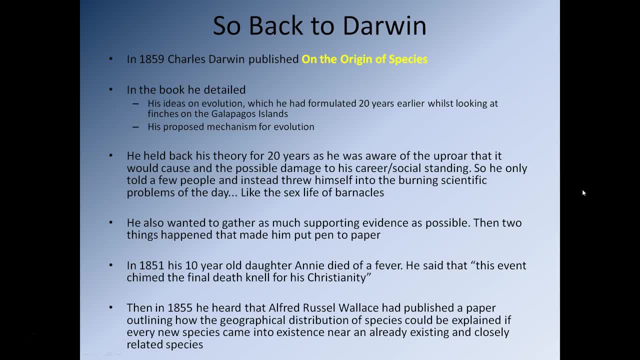 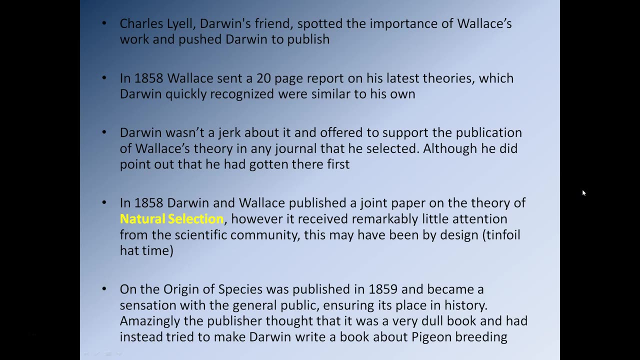 You know, they've got to take on Evolutionary features to adapt to those environments, And so the further, essentially the further he got from the starting valley, The more different the organisms became. So Charles Lyell, Darwin's friend, spotted the importance of Wallace's work. 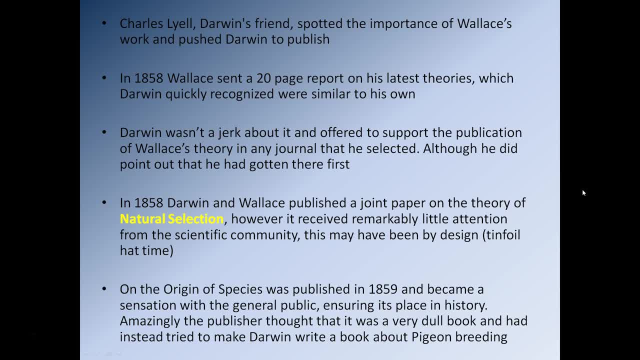 And pushed Darwin to publish. So in 1858, Wallace sent Darwin a 20-page report on his latest theories, Which Darwin very quickly realized was similar to his own. So you know, Darwin could have been, you know, nasty about it. He could have tried to stop Wallace at all costs. 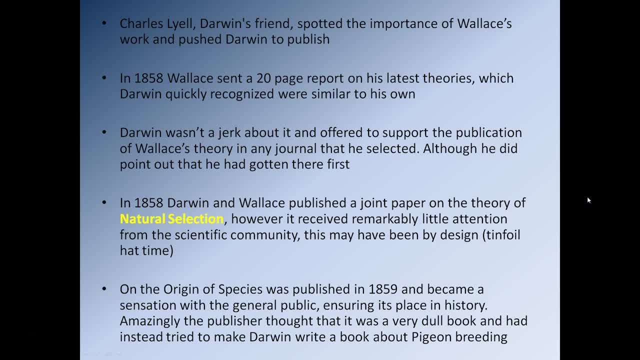 But he didn't. So Darwin wasn't a jerk about it And he offered to support the publication of Wallace's theory in any journal that he selected. So you know, Darwin would support Wallace, He would help him get his ideas published, Although there was one caveat to that. 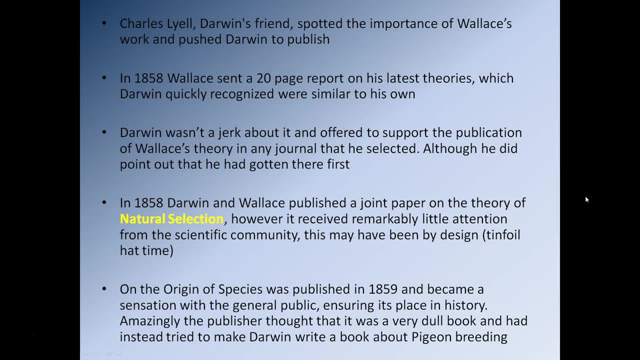 Wallace would have to accept that Darwin came up with the idea first. So what happened was there was a compromise And in 1858 Darwin and Wallace published a joint paper On the theory of natural selection. So when it really comes down to it, 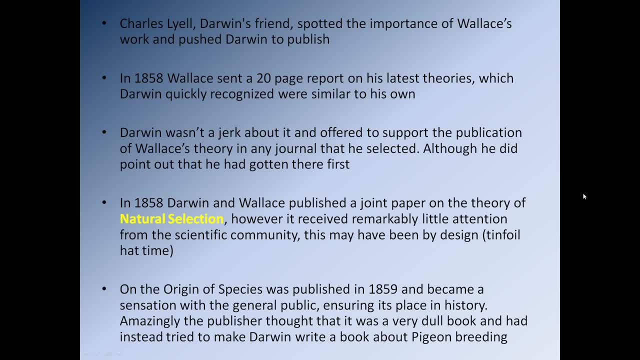 Although we think of Darwin as essentially the person that came up with the idea of evolution, It is, in fact, Darwin and Wallace who came up with the idea of evolution. However, the paper they wrote together in 1858 actually received remarkably little attention From the scientific community. 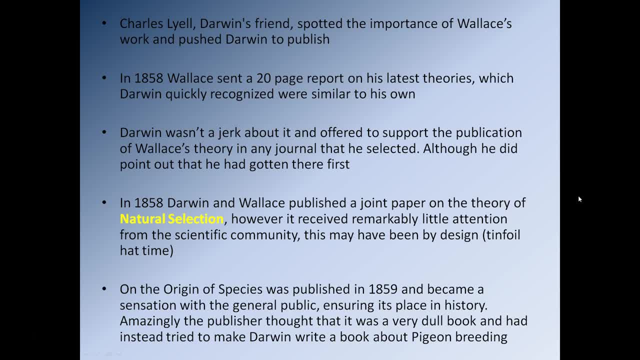 And this may have been by design. There's some suggestions that maybe Darwin's friends did their best to maybe hide the publication. You know, From the, from the larger scientific community, And you know in, you know, to make sure that Darwin would, you know, get all the praise by himself. 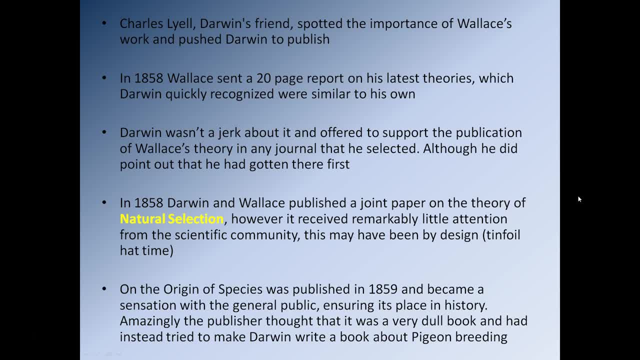 That's debatable, though. So in 1859, Darwin published on the origin of species, And it became an instant sensation with the general public, ensuring its place in history. So amazingly, when the publisher of the origin of species first read Darwin's initial manuscript. 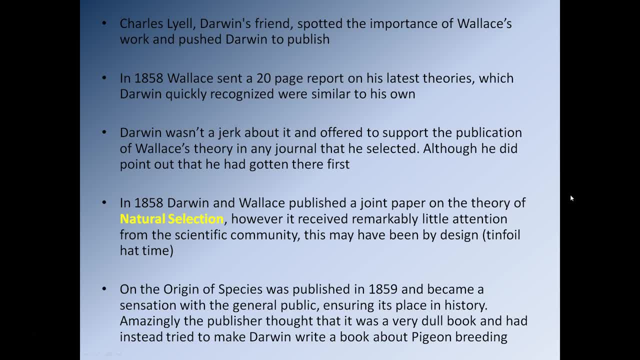 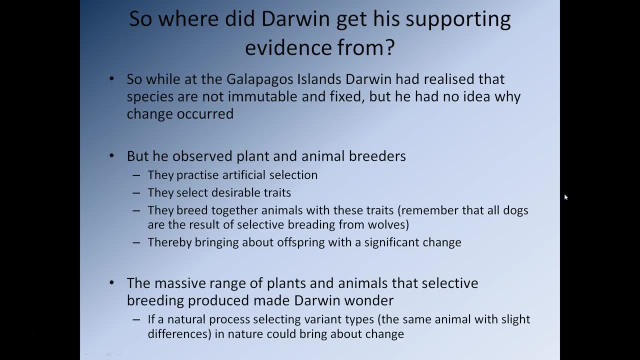 He thought that it was a very dull book And had instead tried to make Darwin write a book about pigeon breeding, Because he thought it would be more successful And would make them both more money. So where did Darwin get his supporting evidence from? 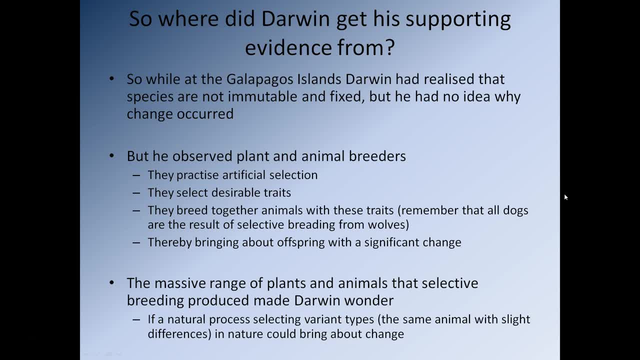 So remember, he got his, you know, his initial evidence was from the Galapagos Islands. So he, you know, saw those different species of different species of finches And he was writing about. you know how the you know the finches would change Depending on what the primary food source was. 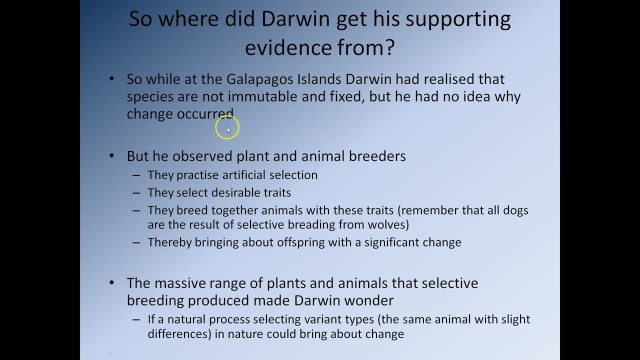 So essentially on the Galapagos Islands, Darwin realized that species are not immutable And fixed and essentially they changed over time. But he had no idea why that change occurred, So he had to try and explain it. So during the 20 years that Darwin essentially waited to publish his work, 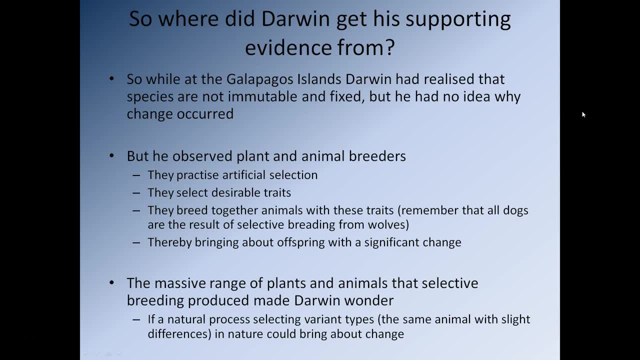 He observed plant and animal breeders. So plant and animal breeders essentially practice artificial selection. So they select desirable traits And they breed animals together that have those desirable traits. So you have to remember that dogs are the result of selective breeding from wolves. 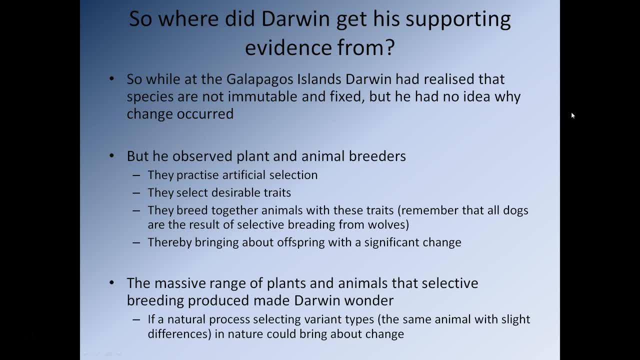 So you know just, the vast majority of dogs look relatively little like wolves, don't they? So clearly, over time, desirable traits have been selected And you've got different. you know lots and lots of different breeds of dog Created from the original wolf. So by selecting these desirable traits, 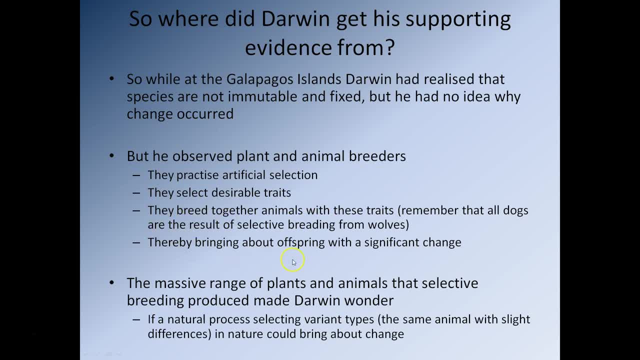 And breeding animals together that have these desirable traits, You bring about offspring that has a significant change From the generations that have come before it. So the massive range of plants and animals that selective breeding Has produced made Darwin wonder. So Darwin began to think if a natural process selecting variant types 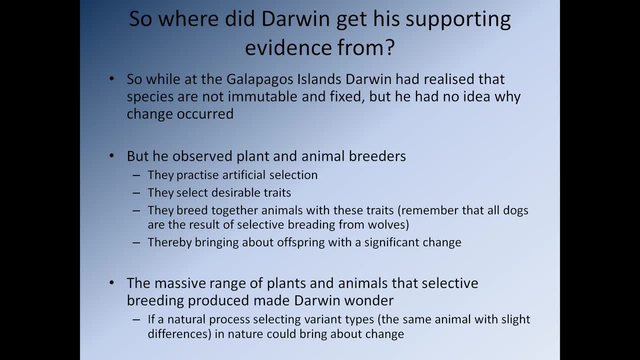 So essentially, a variant type is the same animal with a slight difference In nature could bring about change. So essentially. so let's read that sentence again: If a natural process could select variant types in nature, could bring about change. Essentially, there's lots of slight variations in a population. 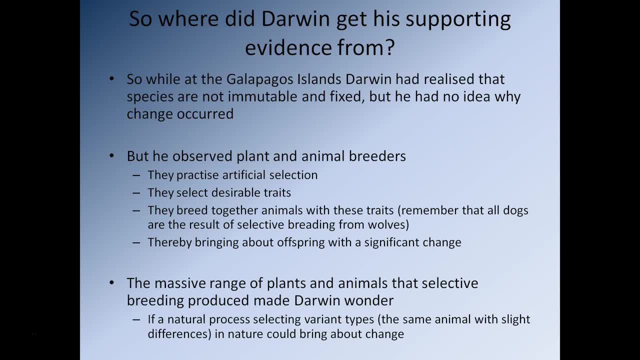 And Darwin suddenly realized: well, if there's some kind of natural reason to select A certain variant within that population, Let's say tall people, short people, for instance, Tall giraffes, short giraffes, You know, maybe there would be some reason to select. 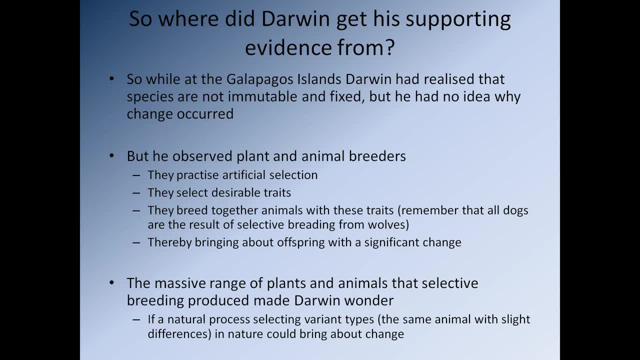 You know one of one of those particular subgroups And, of course, if there is some reason to select that subgroup, That subgroup is going to become dominant within the population. Okay, I've suddenly realized I've run well over the 20 minute break point. 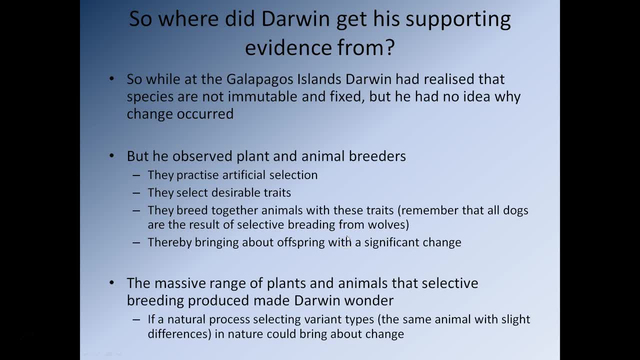 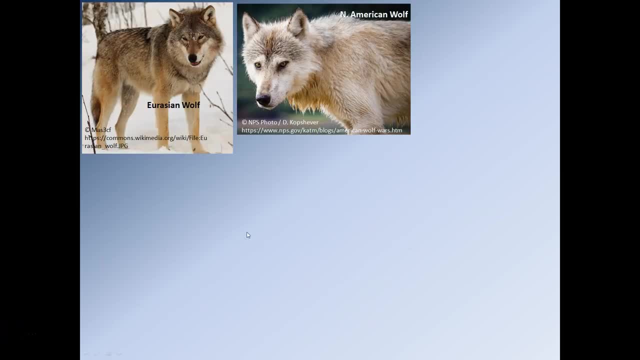 So, anyway, let's take a. let's take a second now. So pause the presentation, Get up, have a walk around And come back to me in a few minutes, Okay, so let's think about dogs. So here we go. So these are wolves. 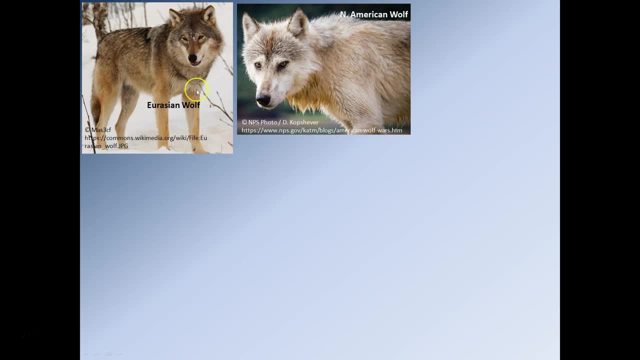 Wolves come in essentially two main groups: There's the North American wolf And there's the Eurasian wolf. The latest research suggests that the vast majority of dog species Are evolved from the Eurasian wolf. So there you go. that's what it looks like. 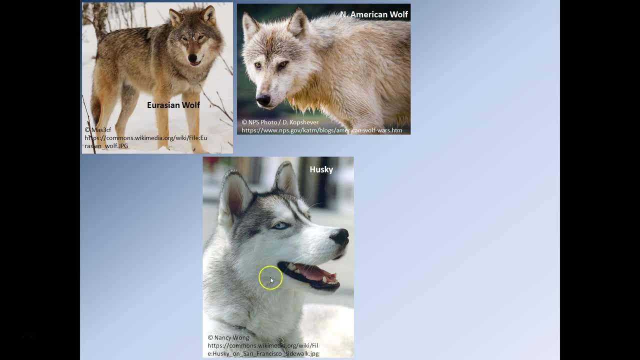 And you know some dog species like the husky. Well, you can see the similarities there. You know they don't look that different. You know even a Jack Russell terrier. You can kind of see some similarities, But you have differences creeping up. 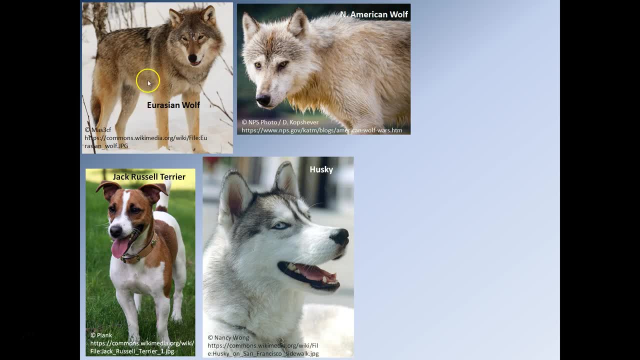 You know differences in the fur, Differences in size, obviously. You know differences in ear shape, etc. etc. So you know, by selectively, you know by selecting certain traits You've got, you've begun to produce offspring That differ significantly from the common ancestor. 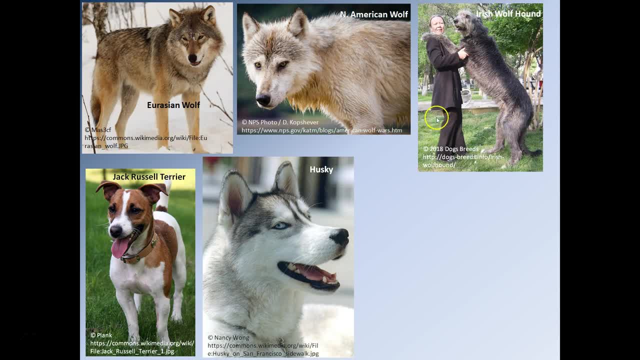 You know. then you have dogs like the Irish wolfhound Which is, I think, the largest dog out You know, largest breed of dog out there. And then of course, If you go to Rickstreams You can end up with dogs like the pug. 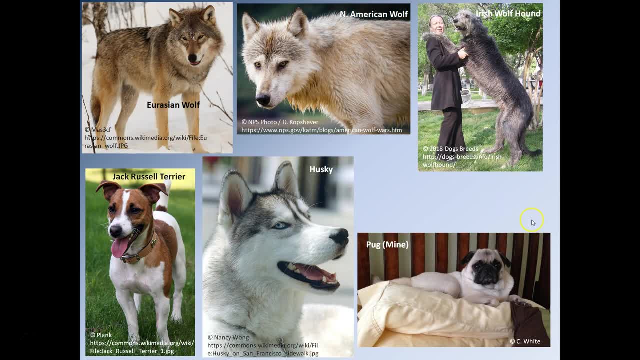 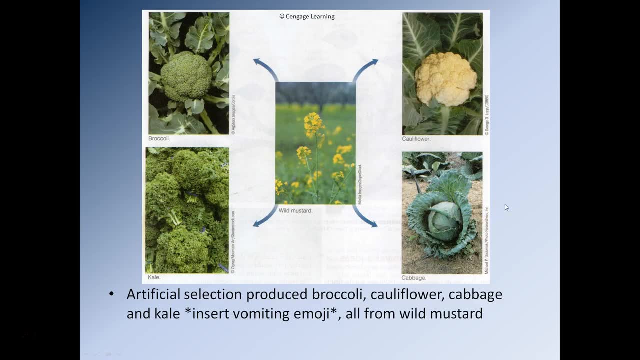 This is my pug here, This is Paddington And in fact, if you listen carefully, You might be able to hear Paddington snoring next to me right now. So that's animals. You can do the same thing in plants, With plants. 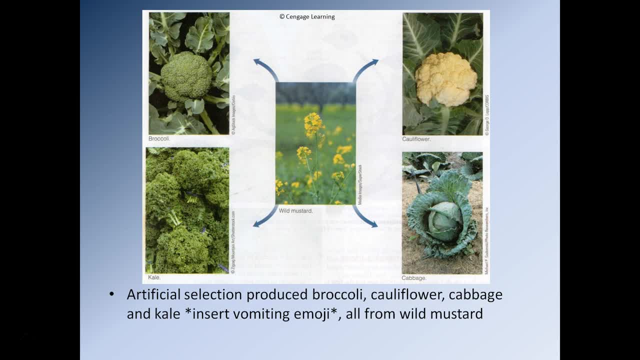 So artificial selection has produced broccoli, Cauliflower, Cabbage and kale, All from wild mustard. So this is the essentially the common ancestor And by selectively breeding certain traits You've ended up with these four very distinct plants. So, essentially, if you just have a process that can select certain traits, 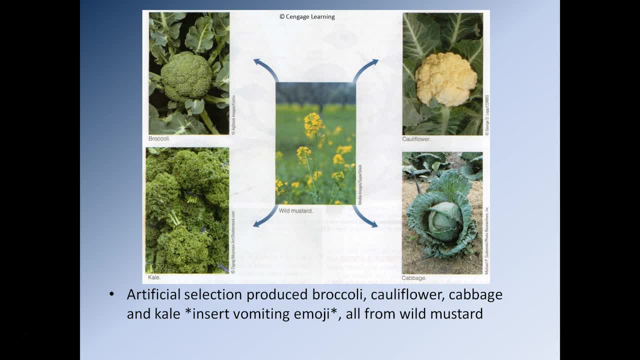 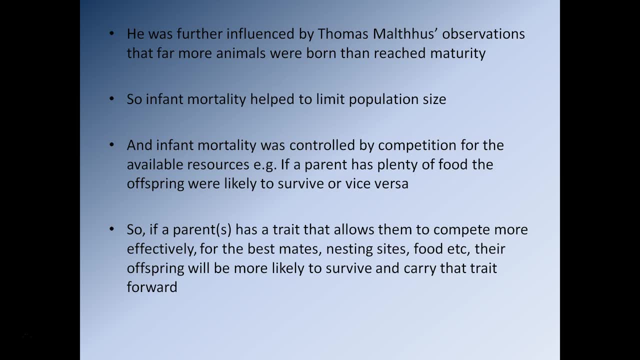 Over time the process will produce offspring That are noticeably different from the ancestor. So Darwin was further influenced by the work of Thomas Malthus, And his observations were that far more animals were born than reached maturity. So it was also realized That infant mortality helped to limit population size. 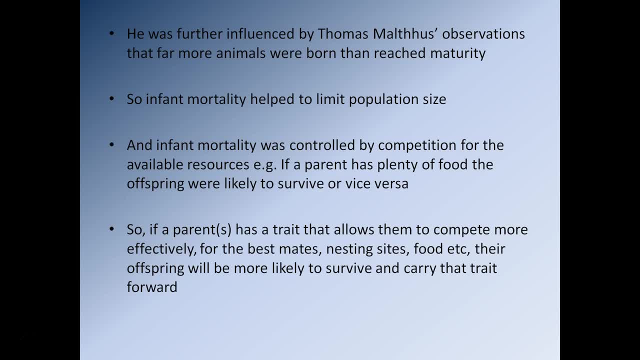 And infant mortality was controlled by competition for available resources. So if a parent has plenty of food for the offspring, The offspring is more likely to survive. If the parent can't get enough food for the offspring, The offspring is less likely to survive. 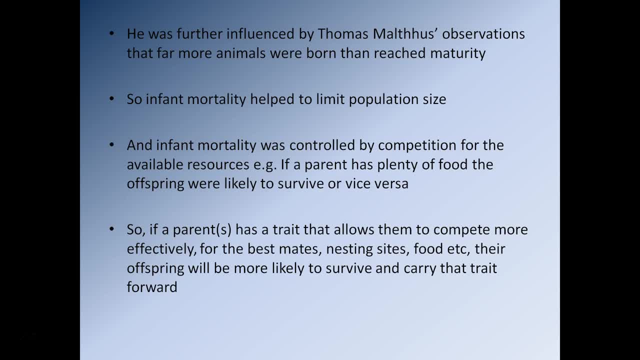 So, essentially, the parent has to have the correct adaptations for the environment. And because it has the correct adaptations for the environment, It's going to be more successful. And because it's more successful, It means there is a greater chance its offspring will survive to adulthood. 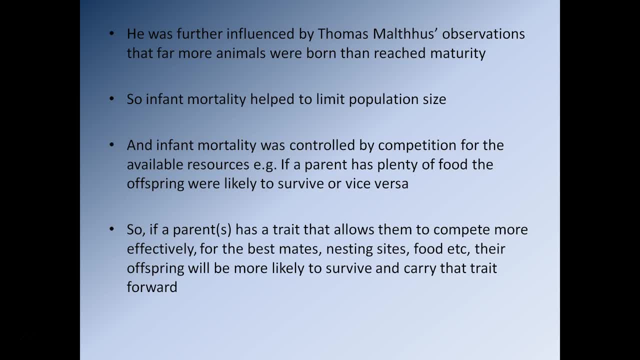 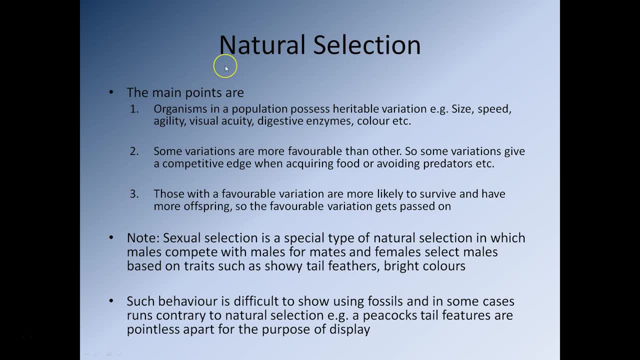 That's the basic argument that's being made by Darwin. So what about natural selection? So the main points of natural selection are: Organisms in a population possess heritable variations. So that's things like size, speed, agility, visual acuity, digestive enzymes, color, etc. 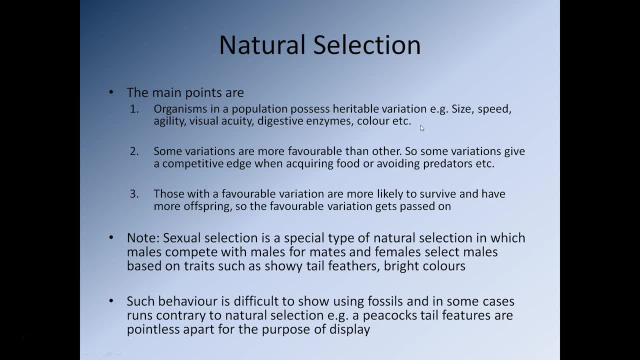 And these heritable variations Can be passed on from parents to offspring. So some variations are more favorable than others. So some variations give a competitive edge When acquiring food, Avoiding predators, Hiding from predators, You know, etc. So those with a favorable variant. 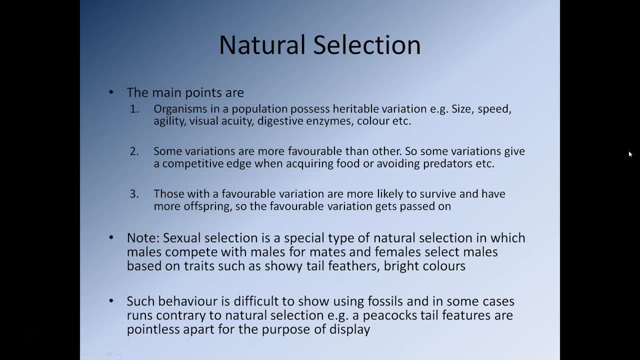 Are more likely to survive. They are more likely to have offspring, And so the favorable off, The favorable variant, Is more likely to get Passed on. So we should note There's actually an additional type of selection, Which is called sexual selection. 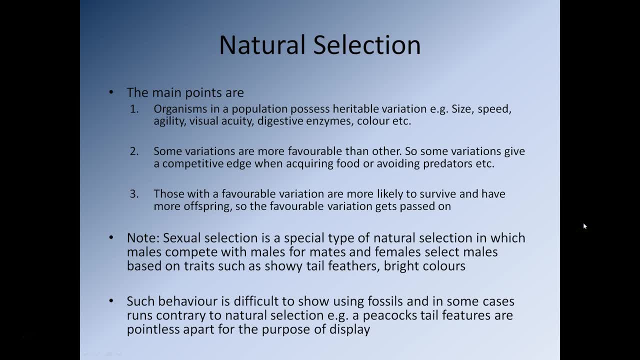 And that's a very special type of natural selection, And in that case, Selection is a type of selection In which males compete with other males And for females essentially, And the females select those males Based on traits such as showy tail, feathers. 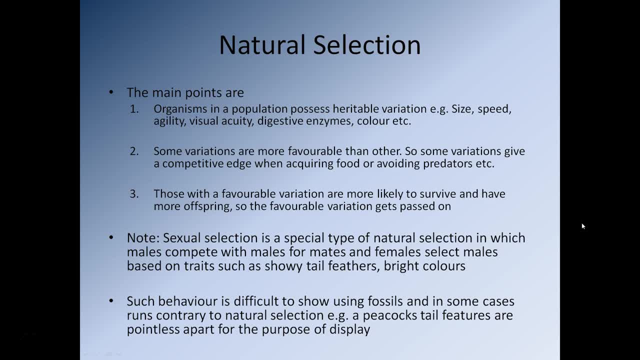 Bright colors, Who's got the biggest horns, etc. And you know, on the whole, This goes against the theory of evolution Because, you know, If you've ever seen a male peacock, You will know that a male peacock Is actually, you know, held back. 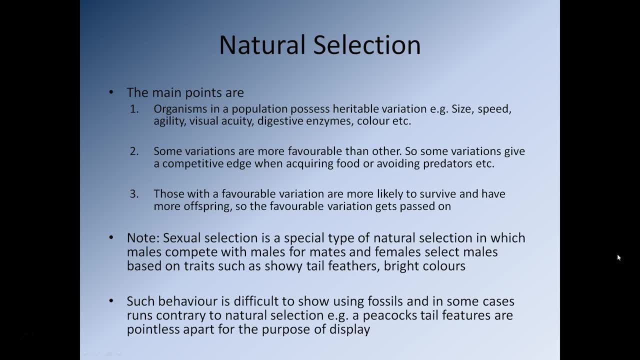 By that huge tail that it has, It gets in the way. It's actually, from an evolutionary point of view, It's completely useless. The only time it is actually helpful Is when you know the males are competing for mates. So you know. 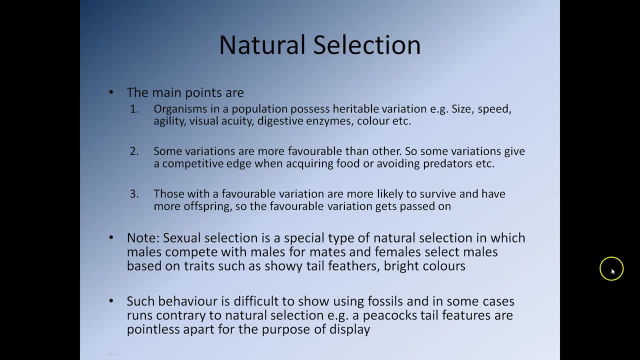 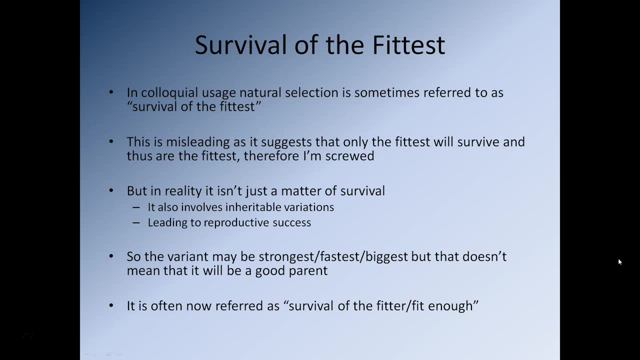 So that's actually a slightly different type of selection That runs against normal natural selection. So that brings us on to survival of the fittest, Which I dare say is a term that you have heard. So in colloquial usage, Natural selection is sometimes referred to as survival of the fittest. 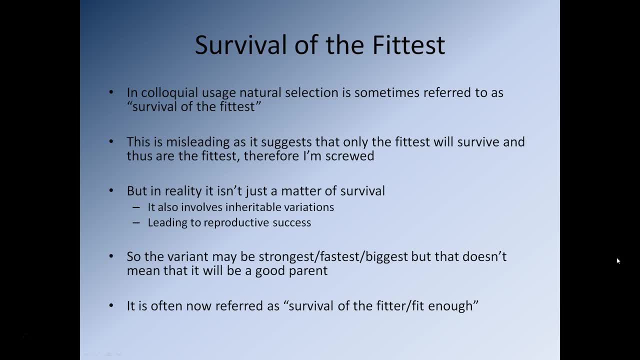 So this is slightly misleading, As it suggests that only the fittest will survive, And thus they are the fittest. But in reality it isn't just a matter of survival. It also involves inheritable variations Leading to reproductive success, So the variant may make you the strongest. 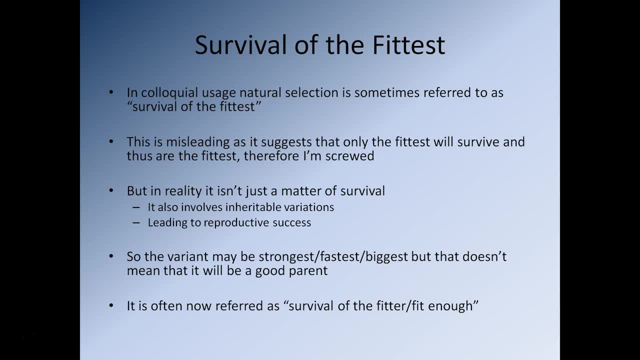 The fastest, The biggest, But that doesn't mean that you will necessarily be a good parent. So that, essentially, has now been rewritten as survival of the fitter Or survival of the fit enough. So you know, just imagine that. you know, you're a chicken. 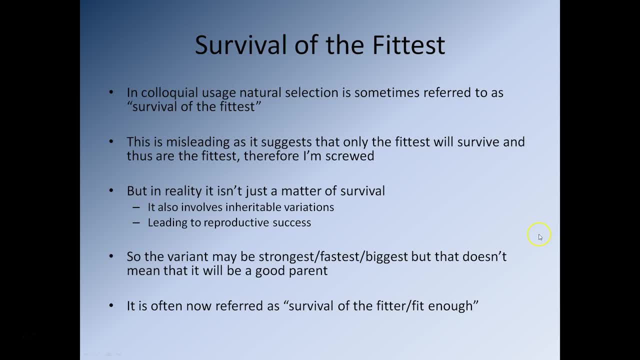 Okay, And you could be the biggest, meanest, nastiest chicken out there. You're the strongest, You're the fastest, So you can out compete all the other chickens really easily. You get all the food And so of course you know that. you know you get the best mates. 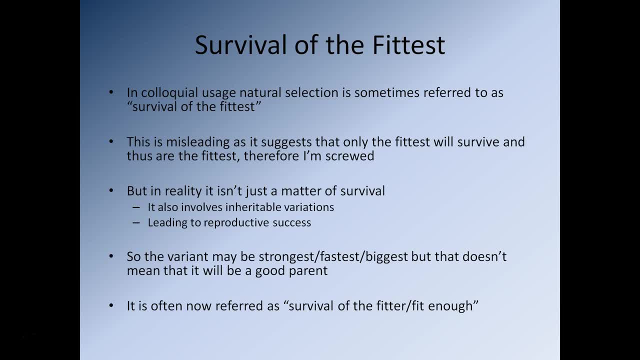 You lay your egg And, of course, because you're the biggest chicken, you sit on your egg to keep that egg warm And you essentially break it Because you're so big. So obviously, in that case, yes, you know, you might have the traits that make you the most. 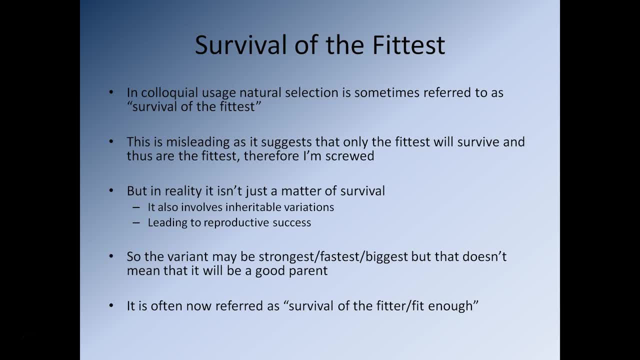 you know, effective adult, But they end up making you quite a bad parent, And so that means that your genetic, you know, your, your inheritable characteristics are not going to get passed on to the next generation. So there's always a balance, And so that's where this survival of the fitter, survival of the fit enough idea comes in. 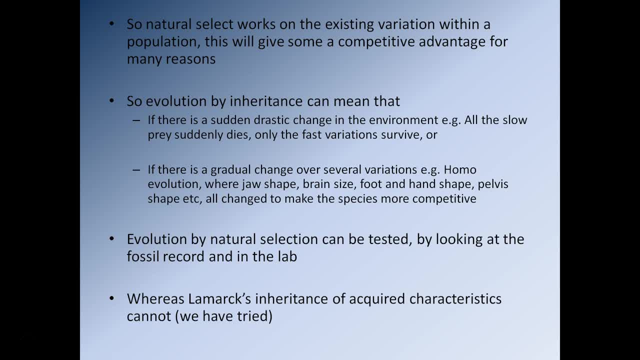 So natural selection works on existing variation within a population And this will give some a competitive advantage for many reasons. So once again this goes back to you know a population of giraffes. You know, let's say half the population is tall giraffes. 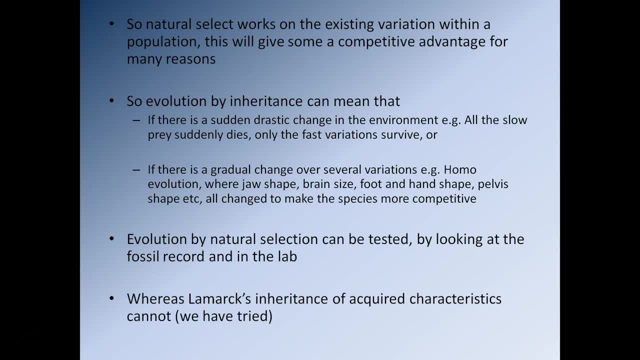 Half the population is short giraffes And you know something in? the environment changes And it means that all the leaves are suddenly growing on tall trees. Well, if you're the 50% of the giraffes that have long necks, you're fine. 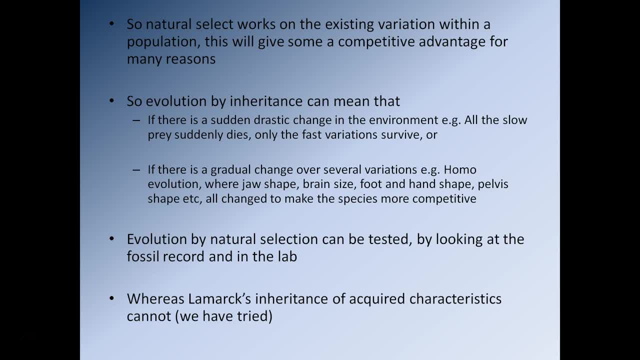 If you're the 50% of giraffes that have short necks, you're in real trouble. So evolution by inheritance can mean that if there is a sudden drastic change in the environment- So for instance, all the slow prey dies and only the fast variations survive- 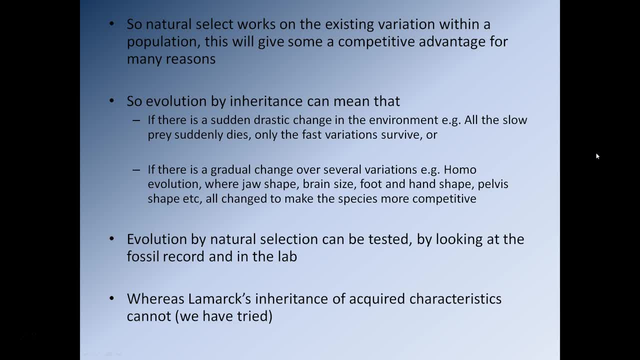 Or if there is a gradual change over several variations, So eg Homo sapiens. So the evolution of the genus Homo, Where, for instance, you'll get jaw shape, brain size, foot size, hand shape, pelvis shape, etc. will change over long periods. 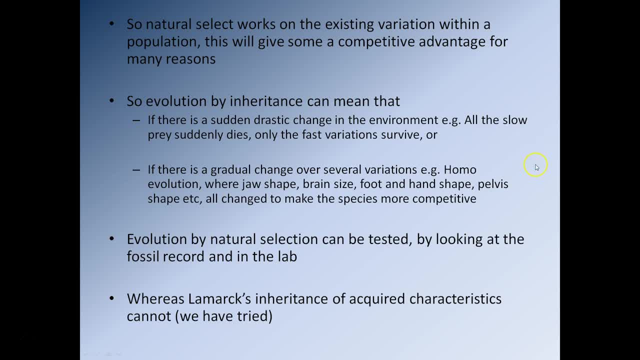 So, essentially, change can be driven by short-term events, Or it can be more of a gradual, long-term process. So evolution by natural selection can be tested by looking at the fossil record and its evolution the lab, whereas Lamarck's inheritance of acquired characteristics cannot be. we've tried it, we failed. 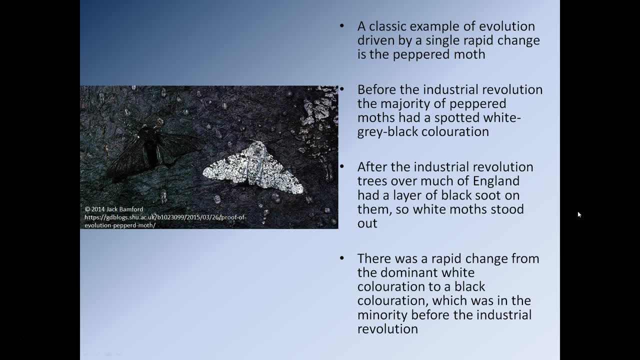 so a classic example of evolution driven by a single rapid change is the pep and moth. so before the industrial revolution, the majority of pep and moths had a spotted white, gray, black color. there it is there. okay, that's the standard pep moth. so a lot of the forests in the united 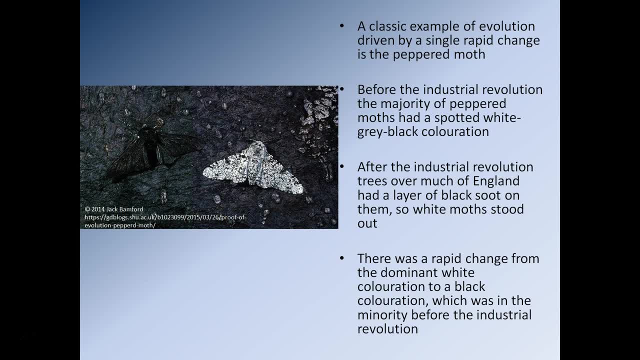 kingdom contain ash and elm. they tend to have quite light bark, and so you know this kind of coloring on a pep and moth is very, very effective. the pep and moth lands on the tree. it's very difficult to see them. therefore they can avoid predators. if they avoid predators, they're more. 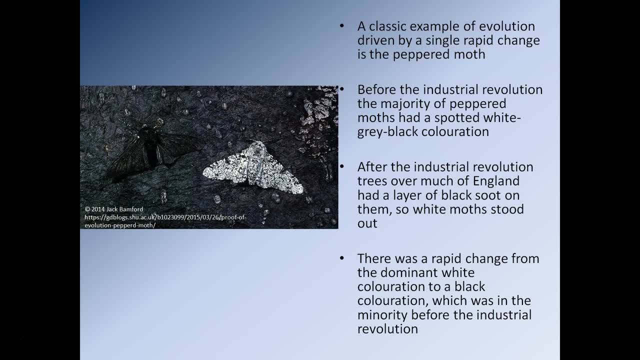 likely to survive. if they can survive, they're more likely to breed and therefore they are more likely to pass on that inheritable characteristic to their offspring. however, approximately 200 plus years ago, the industrial revolution began in the united kingdom, and the industrial revolution in the united kingdom meant that lots and lots of coal was burned, and that meant lots and lots of soot. 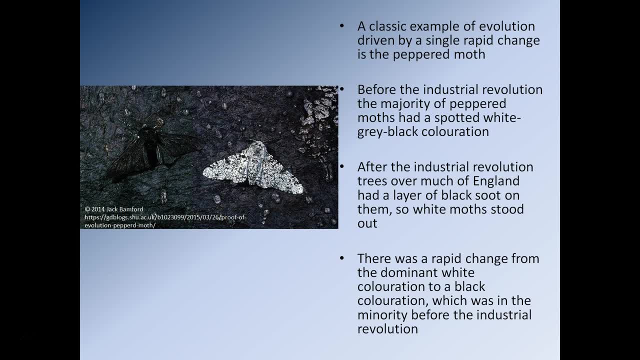 was produced and this soot went on to cover, you know, very, very large areas of the united kingdom and it meant that lots of trees close to industrial centers were suddenly black. you know the, the, the bark got stained black by all the soot coming from the factories. 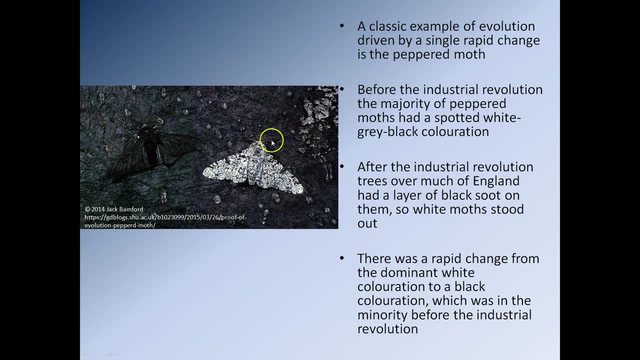 and so, all of a sudden, having this- you know, white coloration was a evolutionary disadvantage- all of a sudden, you stood out. you were more likely to get eaten. you were therefore less likely to, you know, live to adulthood. you were therefore less likely to successfully reproduce and to pass on your inheritable characteristics to the next generation. 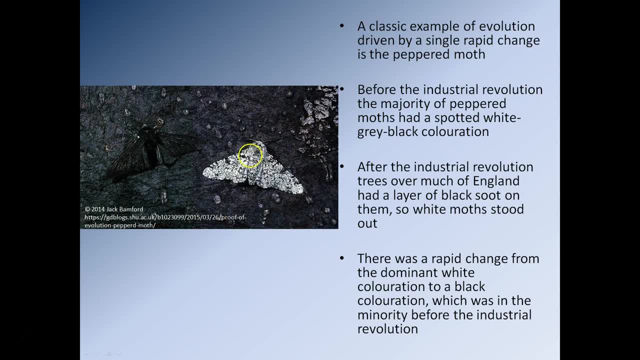 so there was a rapid change from this white coloration to the dark coloration over here now. before the industrial revolution, the dark coloration which you can see here was in the minority. however, as soon as the industrial revolution starts, the trees start getting covered in black soot. 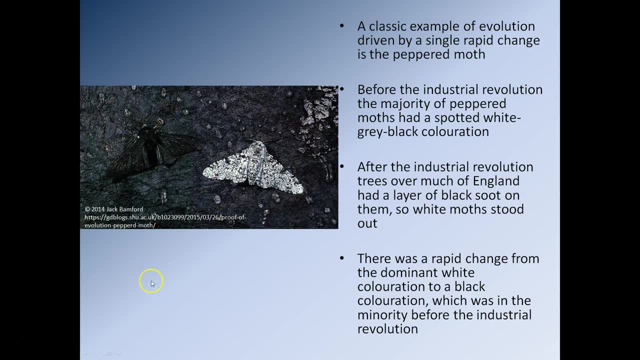 well, all of a sudden, having the black coloration becomes an evolutionary advantage. now, all of a sudden, the black peppered moths. well, they are more likely to survive to adulthood, they are more likely to reproduce and therefore they are more likely to pass their inheritable characteristics. 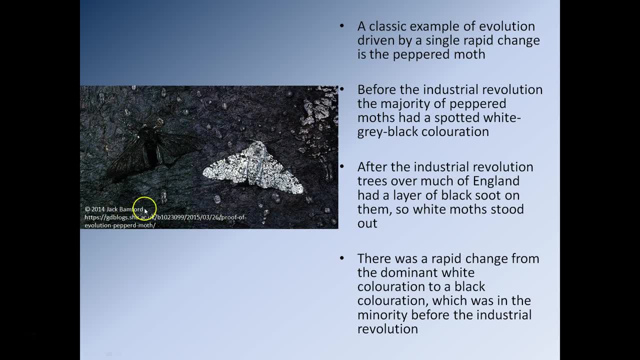 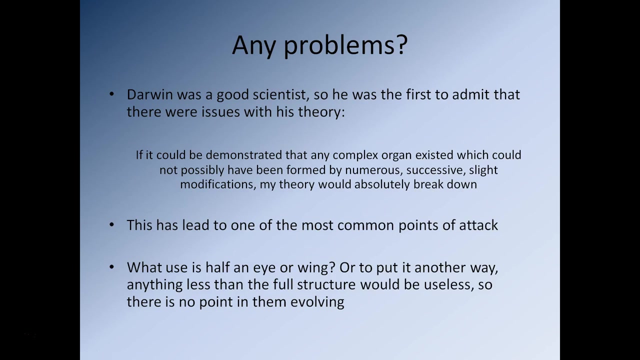 on to the next generation. so essentially, that's. you know, one small change creates significant. it creates a significant shift in the makeup of a species we essentially see. in this case it goes from white to black. so any problems with the theory of evolution? well, Darwin's a good scientist, so he was the 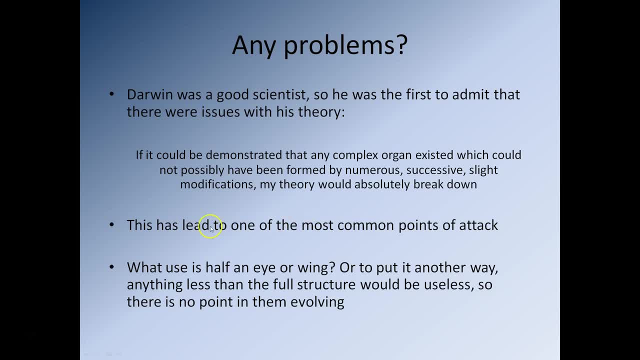 first to admit that there were issues with his theory and before we get into them, let's just pause here. so pause the presentation, get up, have a walk around, come back in a couple of minutes, so okay. so, as i was saying, Darwin was a good scientist and he was the first to admit that. 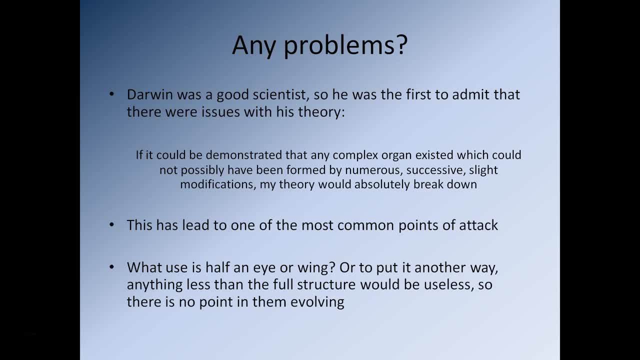 there were issues with the theory of evolution. so he clearly stated: if it could be demonstrated that any complex organ existed which could not possibly have formed by numerous successive slight modifications, my theory would absolutely break down. so if you can essentially find an organ in the huge volume of writing, this could be a much larger organism. so if you can find an organ in the 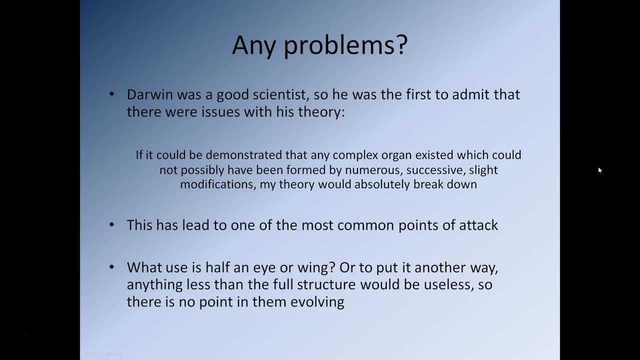 human body or in the body of a dog or, you know, a bumblebee or anything like that. that could not have been made by lots and lots of small steps. essentially that makes evolution fall to pieces, because you can't just have organs you know appearing out of nowhere. it has to be a gradual. 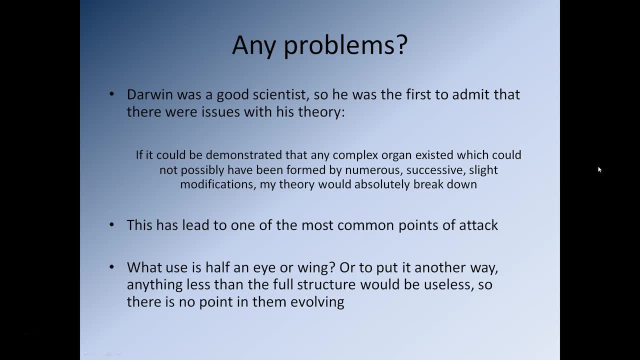 process that brings about their appearance. so this has led to one of the most common points of attack when it comes to evolution. that point of attack is this: what use is half an eye? what use is half a wing? so, to put it another way, anything less than the full structure would be. 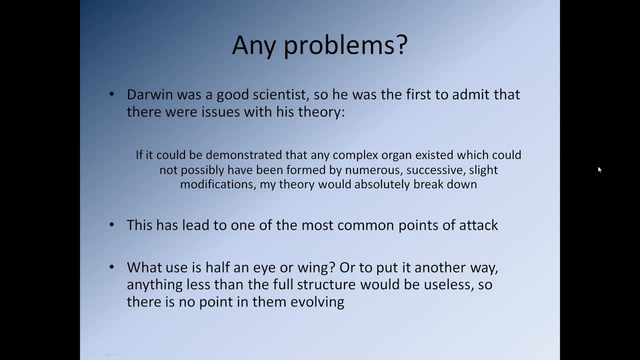 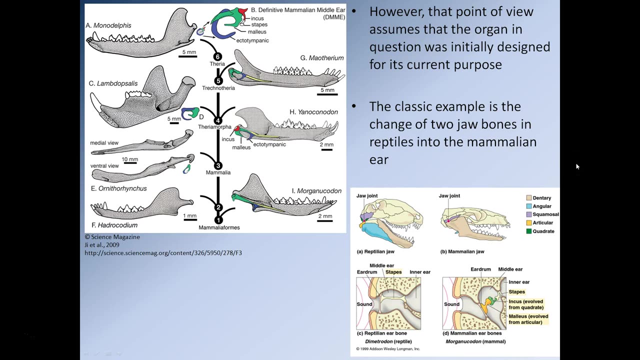 useless. so if that, you know, if half an eye is useless, well what's the point in evolving it in the first place? as soon as you come, you know, as soon as you, you know, if you come at it with that point of view, evolution very quickly becomes, you know, incorrect. however, that point of view assumes 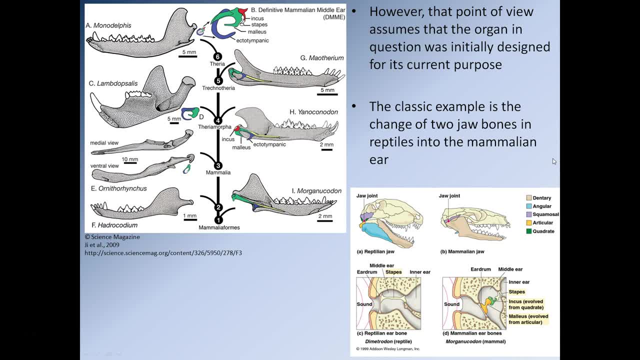 that the organs in question were initially designed for their current purpose, and the classic example is the change of the jawbone in reptiles into the mammalian ear. so okay, so let's look down here in the bottom right to start with. so here's a reptile. 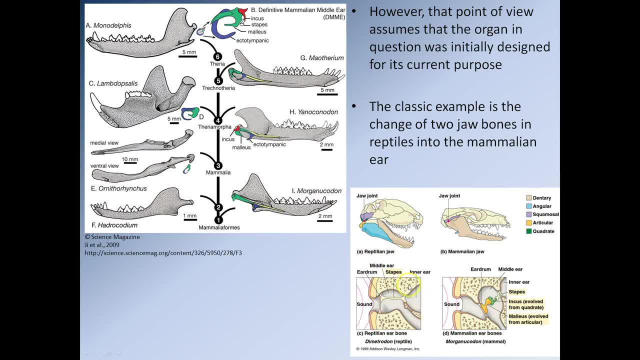 and here's a mammal. so let's look at the ears. so in the case of a reptilian ear, you can see here's the eardrum, here's the inner ear, and they're connected by a single bone. okay, so this single bone is called the stapes and essentially because it's only a single bone, it 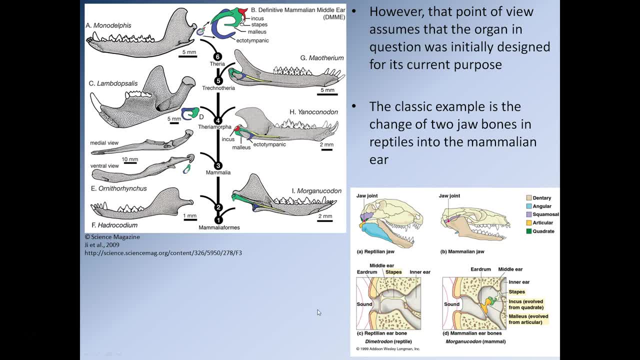 means that reptiles have pretty horrendous hearing. they're not great. now compare that to a mammal. so here's the eardrum again. here's the inner ear. now look at the mammalian ear. it consists of three bones. okay, the malleus, the incus and the stapes, and once again- well, not once again, but 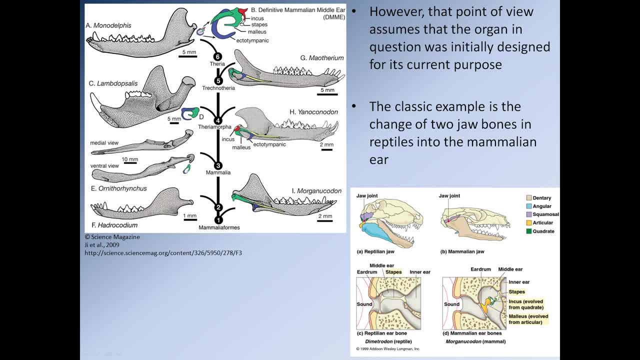 in this case, because you have these three bones, it acts essentially as an amplifier, and so that means the noise that comes into your ear essentially is amplified, and so you can hear better than a reptile. so it's an evolutionary advantage. so the question becomes: is well, where did these bones? 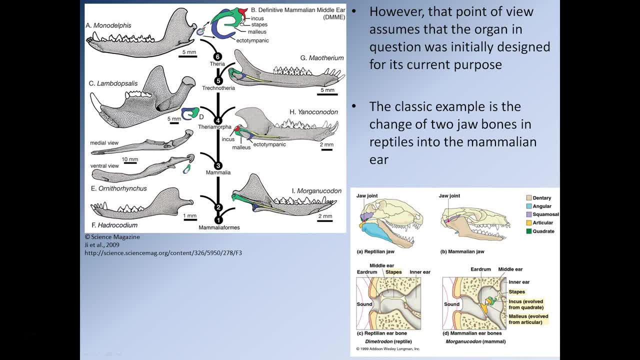 come from. they've got to come from somewhere. they can't just appear out of nowhere. and so when we look at the uh, when we look at the bones of uh reptiles and we look at the bones of mammals, what do we see? well, over time, what we begin to see is we begin to see that the bones in question 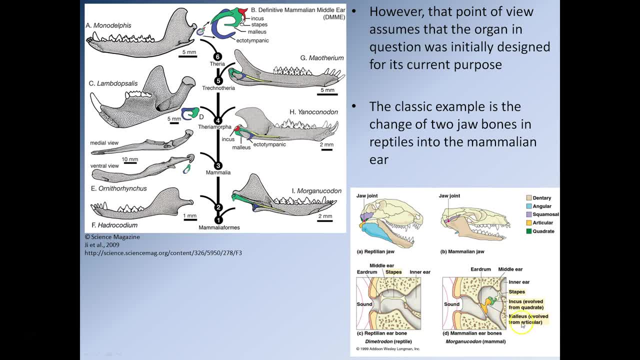 okay, so the malleus malleus essentially evolved from the us articular bone, which is this green bone right here- you can just see, you can just make it out there on the jaw- and the incus evolved from the quadrate, which is this bone. where are we so? the 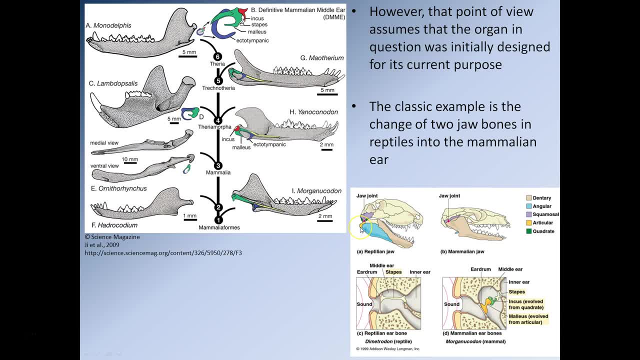 quadrate is the green one, the articular is the yellow one. okay, and so what we see is that these two bones are common in the jaws of reptiles, and what we notice is, by the time we look at mammals, we notice that the bones have gone, so reptiles evolved into mammals. 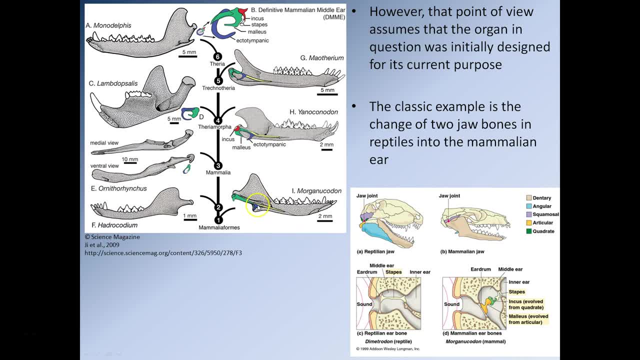 and these two bones have disappeared. what's happened is slowly, over time, they've moved from the jaw and they've slowly moved up into the skull and they've essentially been incorporated into the ear. so these bones didn't just magically appear out of nowhere. they are essentially 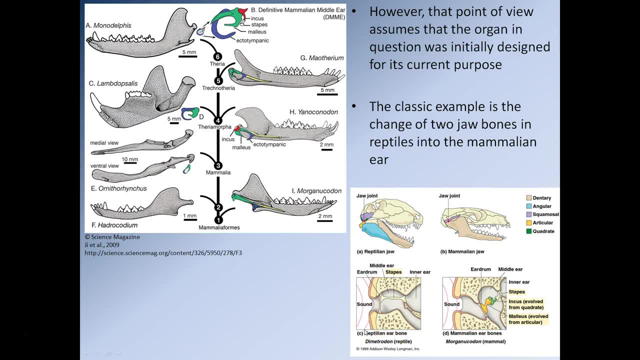 other. you know parts of the body that have been repurposed. okay, so you know. so, once again, you just start thinking of feathers. what's? you know? what's the point of feathers? well, the most likely reason to develop feathers is simply for retaining heat. so it would seem that you know, you know a significant number. 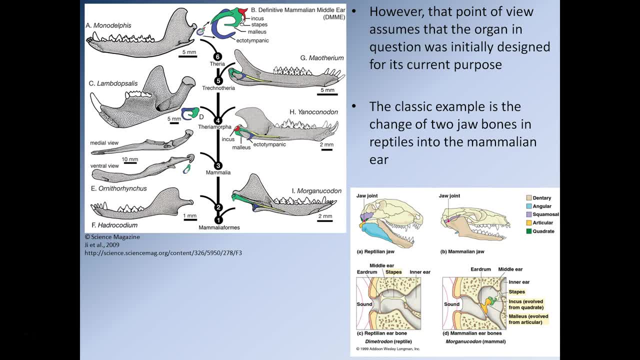 of dinosaur species that we now know of appear to have developed feathers. so, initially, feathers developed, to you know, retain heat, and so well, what happens? well, eventually, the feathers on the arms begin to become larger. as they become larger, all of a sudden, you can start to use them for. 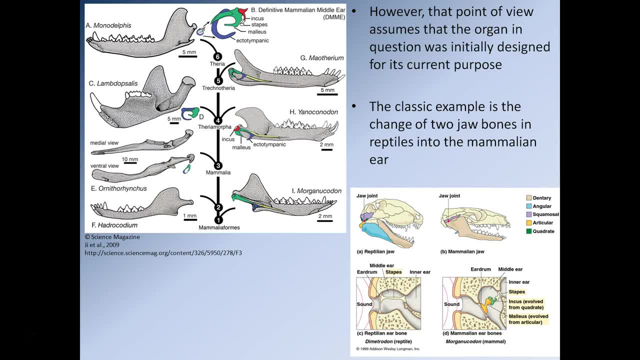 gliding. well, think about it, birds. birds don't use their forelimbs, do they? they use them to fly, but when a bird lands somewhere, it obviously stands on its hind limbs and it uses its beak. okay, so the same goes for dinosaurs. when it really comes down to it, dinosaurs only require 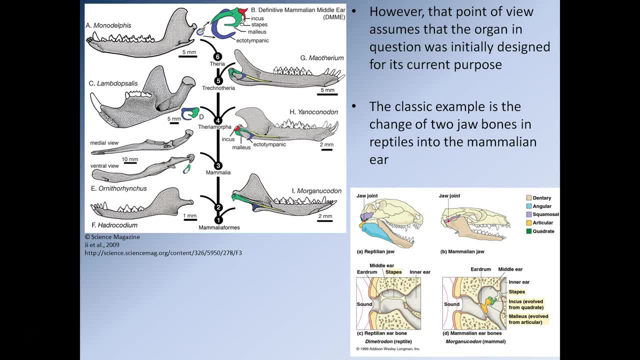 only require their two hind limbs and, essentially, their head. the forelimbs, when it comes down to it, on the whole aren't that important. i mean, look at the forelimbs of a Tyrannosaurus rex, for instance. they're pretty much completely useless. so all of a sudden, as soon as you start developing large feathers on the forelimbs of you know small 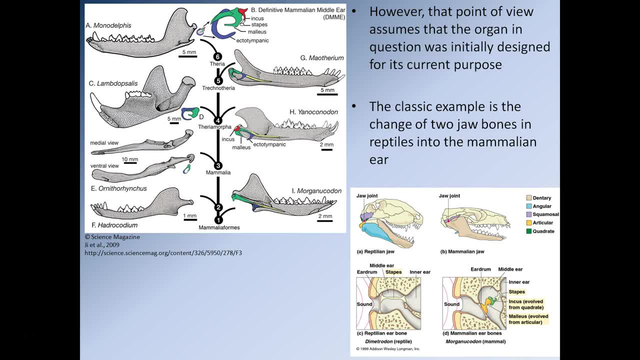 dinosaurs, like raptors- okay, think of velociraptors from Jurassic Park. well, once that begins to happen, essentially, you have these large feathers, you have these forelimbs and all of a sudden your animals can start gliding, and then you start to end up with organisms like and like Archaeopteryx. 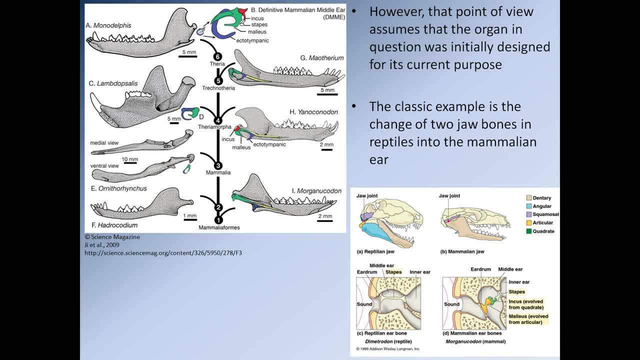 which we'll discuss more when we come on to Mesozoic evolution. and once you have animals that can start to glide, well, over time the forelimb begins to become larger and larger and become more and more specialised, until you end up with organisms that essentially can have. 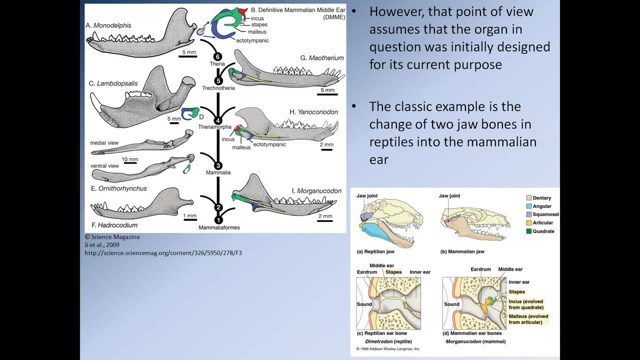 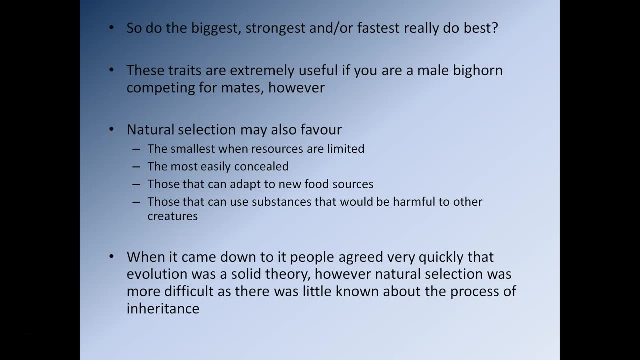 powered flight, they can flap their wings to produce sufficient lift to actually get off the ground. so, once again, the initial structure has absolutely nothing to do with the use that it ends up performing. so the next question is is: do the biggest, the strongest or the fastest really do? 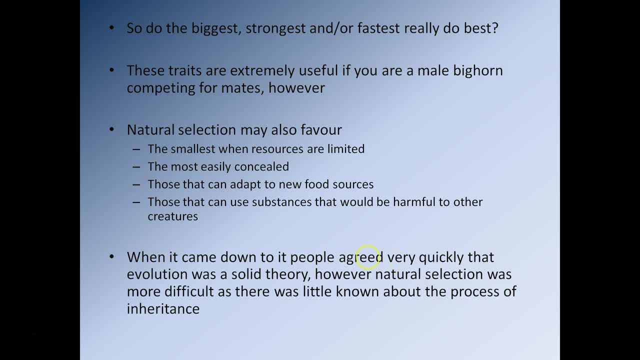 best. we've already kind of touched on this. so these traits, being the most important features of the biggest, the strongest, the fastest, are extremely useful if, for instance, you're a male bighorn competing for mates. however, natural selection may also favour the smallest when resources are. 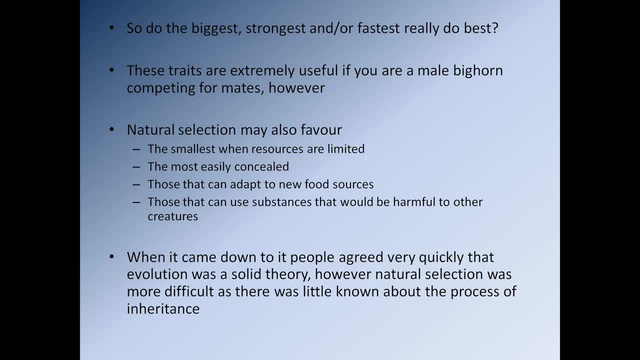 limited, obviously, if there's less food going around. you know, being smaller and requiring less food is an advantage. they can also sometimes favour the most easily concealed. they can favour those that can adapt to new food sources and evolution, can favour those that can, those that you can use substances that would be harmful to your environment and therefore can be harmful to 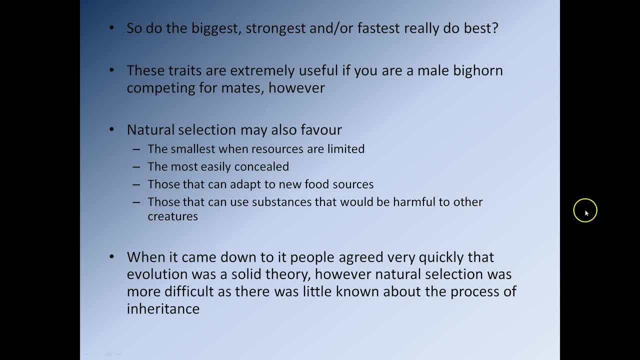 other creatures, and the classic example for this is new york city rats. so you know, over time, uh, the rat population in new york has become a real problem, and so obviously you know what the rat catchers do: they put down poison to try and kill the rats. the problem is is imagine you have a. 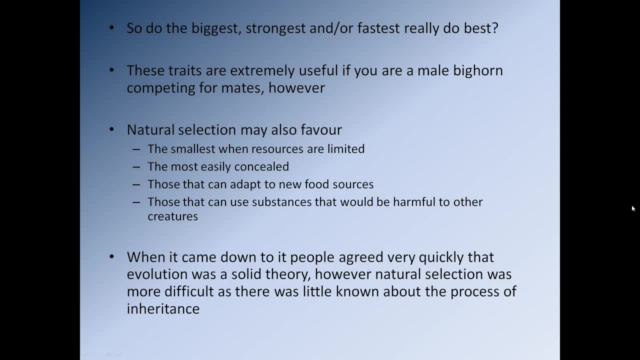 situation where you put down a new poison and let's say it kills 75 percent of the rat population. the problem is: is the other 25 percent of the rat population can eat that poison and not die? so what happens? well, that 25 percent now breed and essentially, the next generation is now immune. 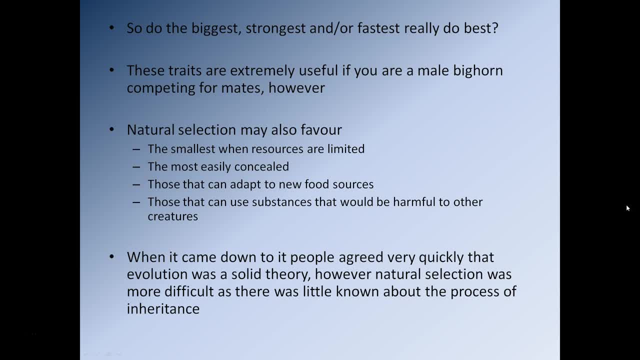 to that poison. so you put a new poison down. that's that kills off 20. you know, let's say, that kills off 75 of the population. well, once again you've still got 25 of the population, yeah, alive. so that one's now. you know that next generation is now, you know, uh, is now- resistant to that particular poison. 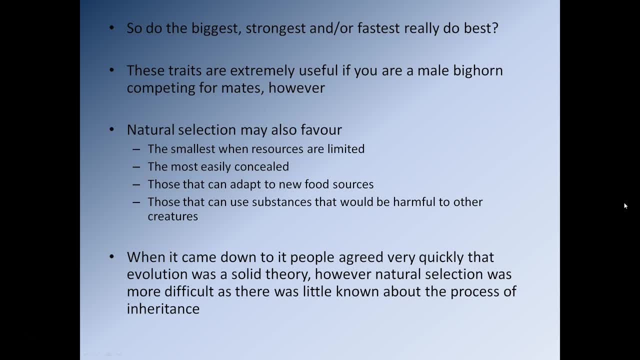 so now you have a you know, a you know a generation that's now resistant to two poisons, and every time you use a new poison, part of the you know part of the community you know is is uh is not affected by it, and so that uh inheritable characteristic gets passed on to the next. 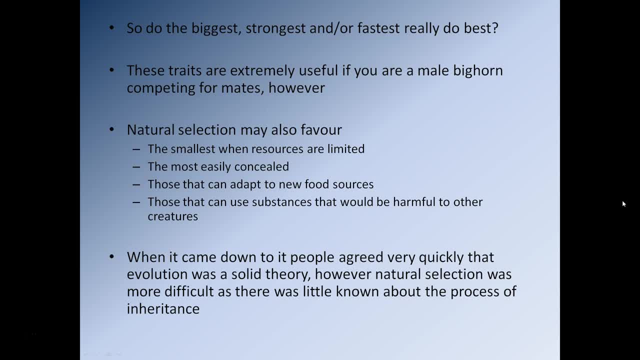 generation, and so new york city rats have slowly but surely been becoming more and more resistant to more and more poison, so they're getting more and more difficult to kill off. so when it, when it came down to it, people agreed very quickly that evolution was a solid theory. it made complete sense based on the evidence that was available. 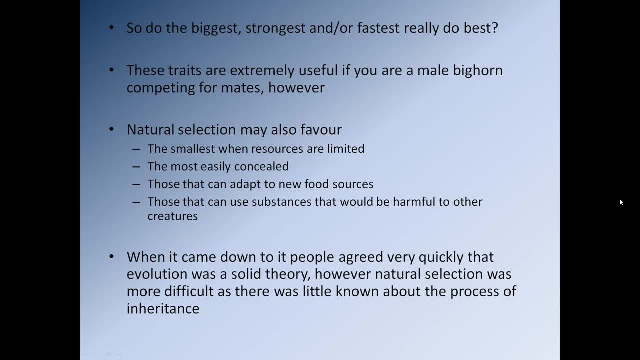 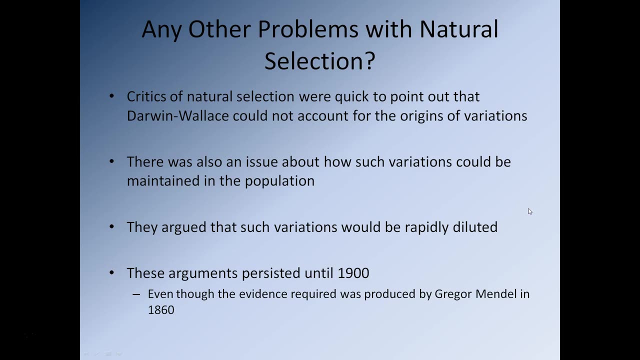 however, natural selection was more difficult as there was little known about the process of inheritance. how do parents actually pass on the inherited and inheritable characteristics to their offspring? so are there any other problems with natural selection? well, critics in natural selection were quick to point out that the darwin wallace model could not account for the origins. 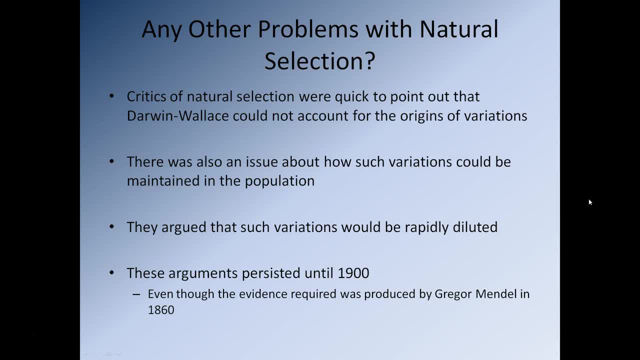 of variations. where do they come from? okay, so you know. if you imagine you have a, you know, a population of 100 drafts, 99 of the drafts have short necks and then one of the drafts has a really really long neck. so the obvious question is: 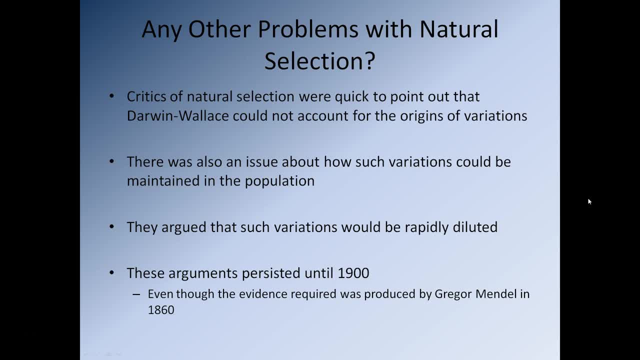 well, where did that one long neck giraffe come from if the rest of the population has short necks? so there's also an issue about how such variation could be maintained in a population. so let's say the long neck draft. you know, it reaches adulthood and it gets. 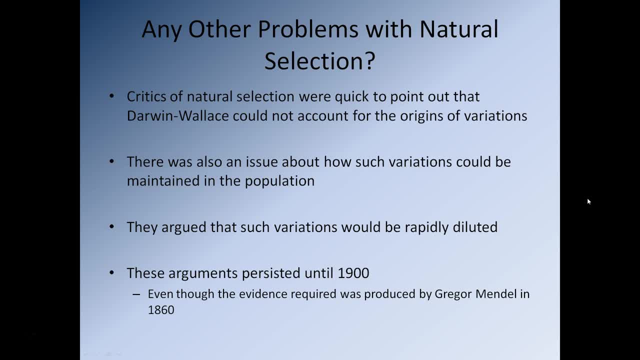 to the point where it can breed. well, it breeds with a short neck draft. well, surely that would mean the offspring would essentially be a medium neck draft. that medium neck draft then breathes eventually once it reaches adulthood, and that produces a short neck draft with a slightly longer 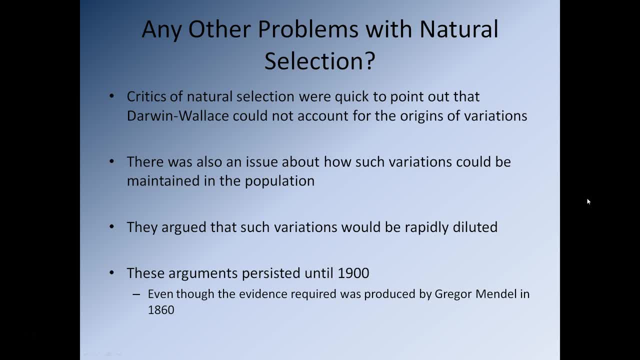 than average neck, and then, as you breed again, and again and again, the each generation essentially loses the long neck trait. that was the basic argument, and so essentially that means that any variation would very, very rapidly be diluted in the long neck tradition. so that's exactly what we're. 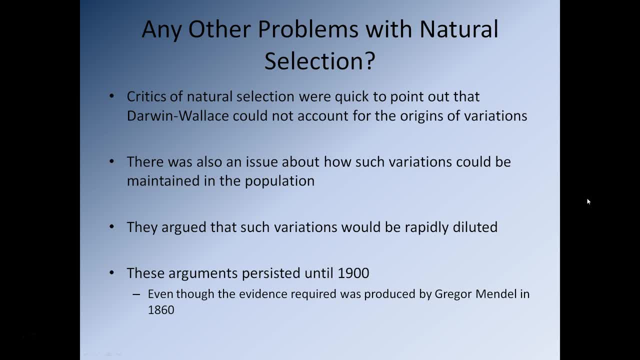 diluted in the population and would therefore be lost, So these arguments actually persisted until the very early 1900s. interestingly though, the actual evidence to explain why these variations could persist in a population was actually produced by a gentleman called Gregor Mendel in the 1860s. 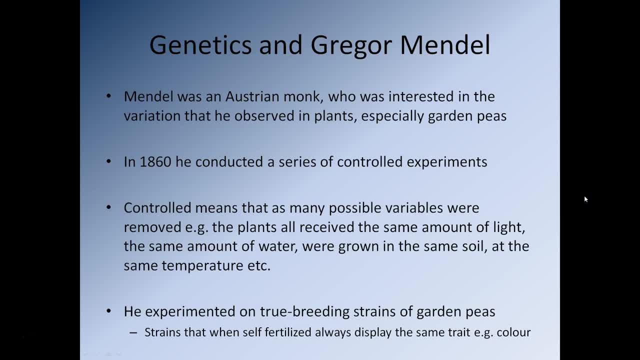 So what did Mendel actually find? So Mendel was an Austrian monk and he was interested in the variation that he observed in plants, especially garden peas. So in 1860 he conducted a series of controlled experiments. Now, controlled means that as many possible variables are removed. 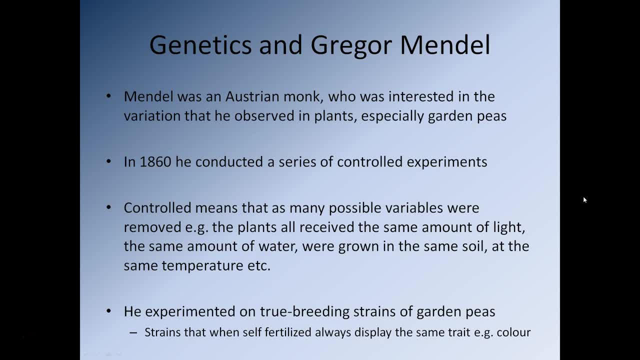 So he was growing plants. so what he would do is he would make sure that all the plants received exactly the same amount of light. they each received exactly the same amount of water. they were all grown in exactly the same soil. they were all grown at exactly. 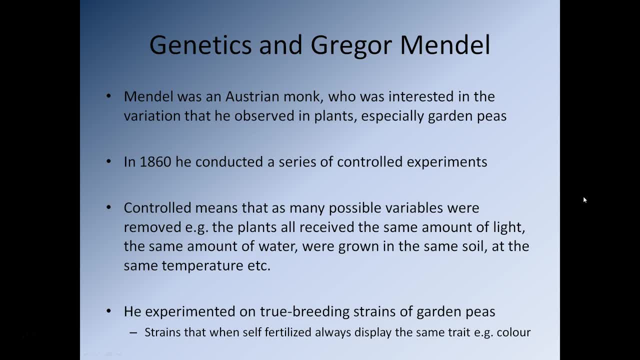 the same temperature, And by doing all of that, he was able to measure the variation in the population. And by doing all of that, it means you instantly remove variables that could have affected your results. So what he did is he experimented on true breeding strains of garden peas. 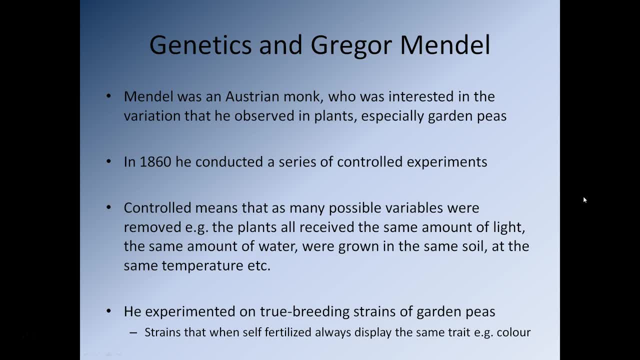 So what's a true breeding strain? A true breeding strain is a type of plant that if you self-fertilize it, OK. so if you make the plant self-fertilize, the offspring it produces will always have the same traits as the parent. 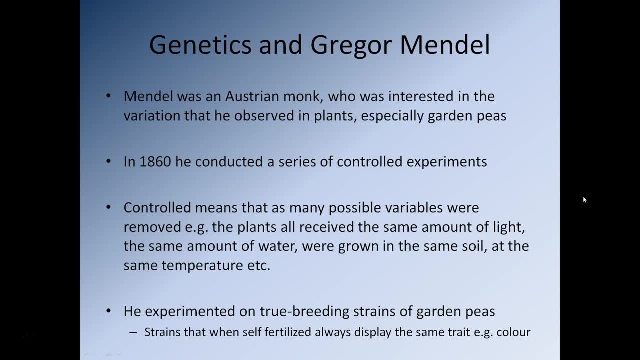 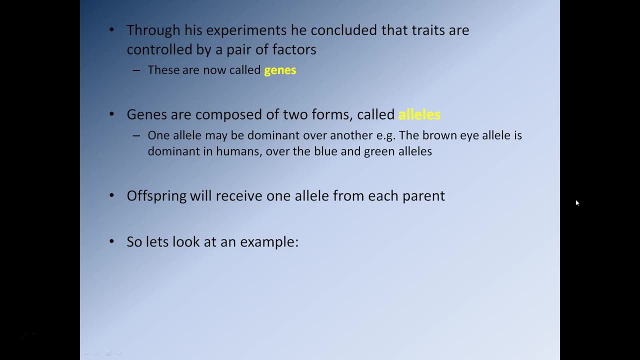 In this case, colour. So Gregor Mendel. he had a question: Who is this? OK, so he has a question. Mendel would self-fertilize pink pea plants and the offspring they produce would be pink. So through his experiments he concluded that traits are controlled by a pair of factors. 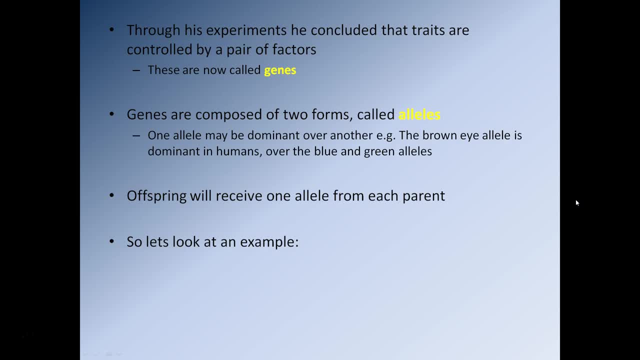 which are now called genes. So genes are composed of two forms called alleles, So one allele may be dominant over the other. So, for instance, in humans the brown eyed allele is typically dominant over the blue or green eyed allele. So you know. so, if you have, 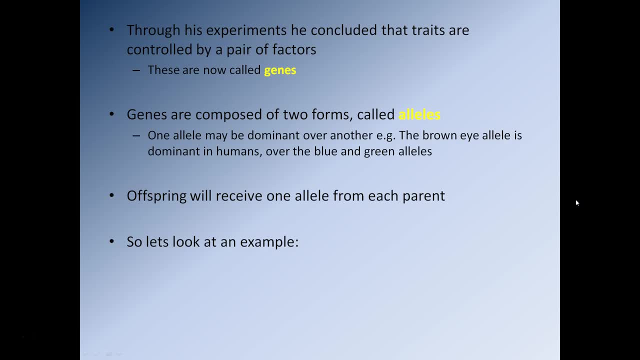 one parent with brown eyes, one parent with blue eyes, it's more than likely any offspring will have brown eyes. Now, that's not always the case, to be clear, but you know it occurs in the majority of cases. So offspring will receive one allele from each parent. So let's look at an example. 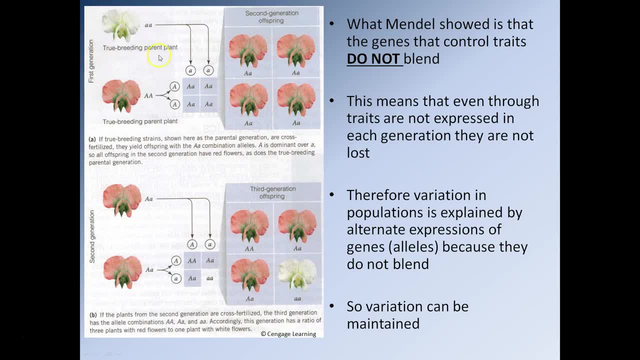 So here's the situation. So Mendel took a true breeding white pea plant and a true breeding pink pea plant. So the alleles for the white breeding pea plant are lowercase a lowercase a and the alleles for the true breeding pink plant are uppercase a uppercase a. Okay, so each one of these alleles. 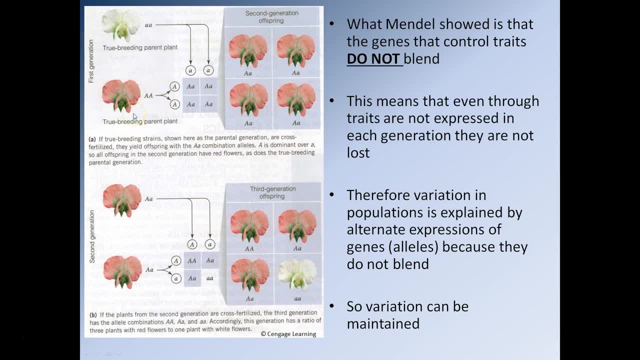 would have come from the parent that made this plant, So okay. so if you say: right, when this plant breathes with this plant here, Well, one allele is going to go one way, one allele is going to go to the other way, and those alleles are going to combine to form the offspring. Okay, so that means we have uppercase a and uppercase a. 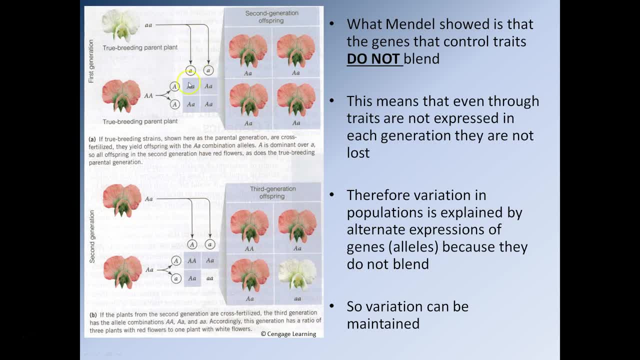 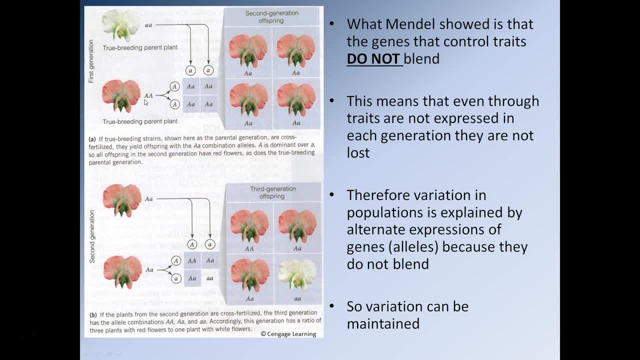 allele is dominant. Okay, so the uppercase a allele is dominant and the pink allele is dominant, So the pink allele is dominant. therefore, pink is dominant over white. So that means our four offspring each have the dominant allele, and so that means the offspring are going to be pink. Okay, so that's. 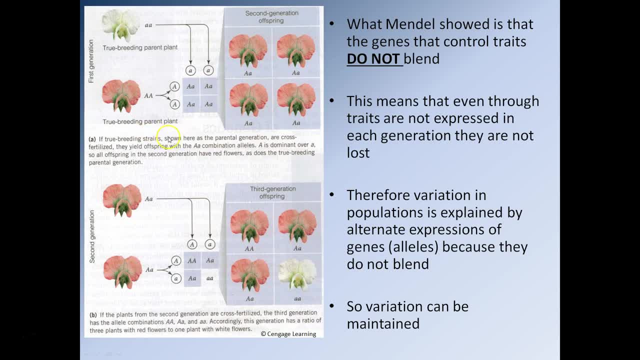 stage one. So then, what Mendel did is he then took some of the offspring and he bred them together. So as soon so he bred the offspring together. so one, the offspring, obviously uppercase a lowercase a two alleles, and the second offspring, uppercase a lowercase a two alleles. 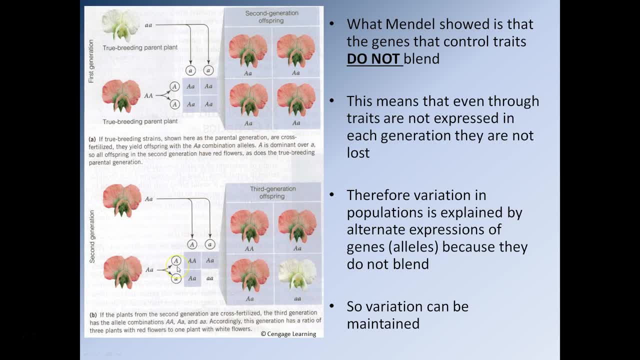 But, once again, when you, when you breed them together, one allele, one allele comes from one parent, one allele will come from the other parent. So uppercase a, uppercase a gives you a plant that has an allele mixture of uppercase a, uppercase a. That means the pink. the plant will be pink. 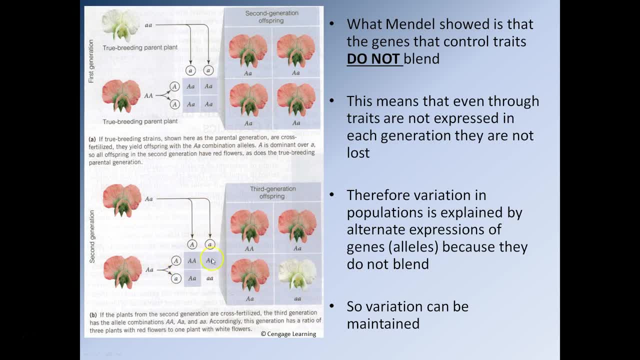 Uppercase a to lowercase a. Well, once again the uppercase a allele will be dominant, so the plant is pink. Uppercase a to lowercase a. once again, uppercase a allele. lowercase a case A allele. so the plant is going to be pink. but lowercase a to lowercase a. 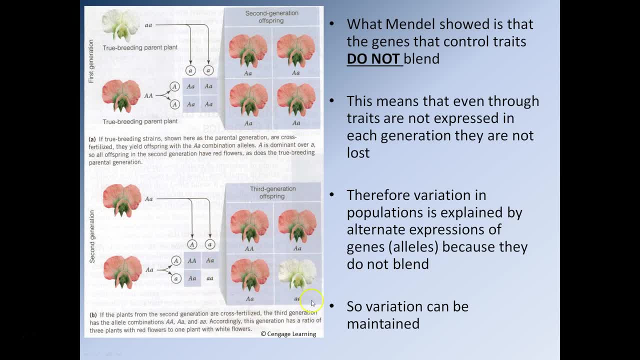 gives you two lowercase a alleles and the plant will be white. So, all of a sudden, Mendel has shown that the genes that control traits do not blend, so they don't get lost. So essentially, what we're saying here is a long-necked giraffe. 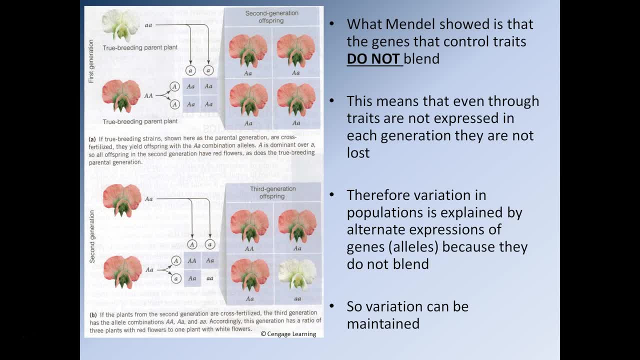 breeding with a short-necked giraffe will not produce a medium-necked giraffe, because those traits don't, you know, don't combine. So this means that even though traits are not expressed in each generation, they are not lost. So in this, 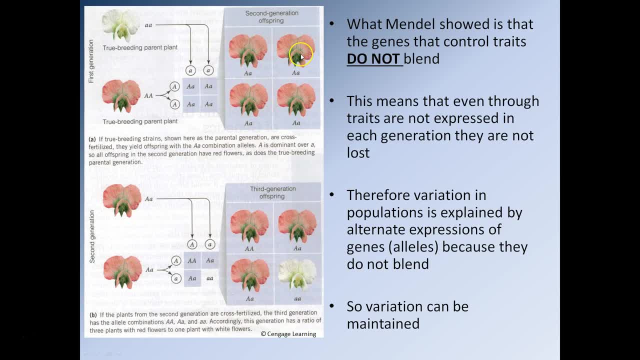 generation, there are no white pea flowers. however, the trait that produces white pea flowers has not been lost. it's there in the genetic material. all you need are two correct parents to breed, to produce the offspring that has the variant. therefore, variation in populations is explained by uh is explained by alternate expressions of. 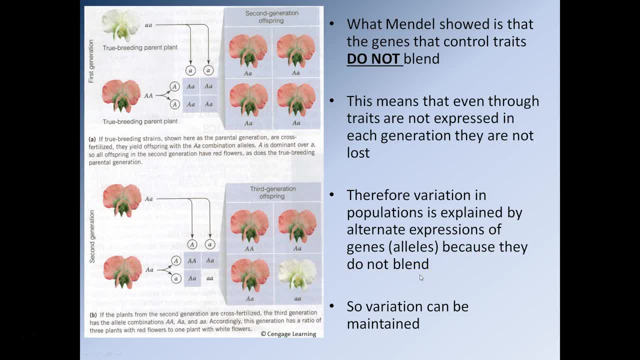 genes because they do not blend. so essentially, you know every generation. it's just essentially a case of shuffling the deck. you know the deck being the genetic information for both parents and pretty much seeing what turns up. so that means that variation can be maintained if the 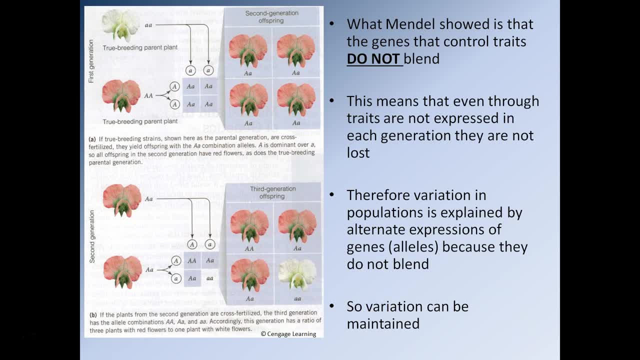 genes aren't being lost. they are always there in the gene pool, somewhere. it just requires the correct parents to come together and essentially, you know if you, if they have the correct genetic makeup, that means variants that have been hidden for a long period of time can reappear. 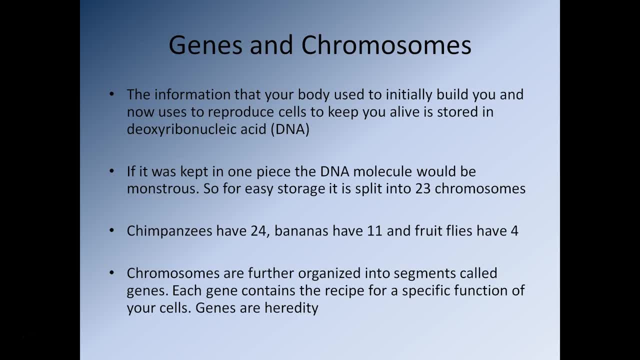 so the information that your, that your body, uh, used to initially build you and now uses to reproduce cells to keep you alive, it's stored in dna. so if it was kept in one piece, the dna molecule would be truly monstrous. so, for easy storage, what happens is organisms split the. 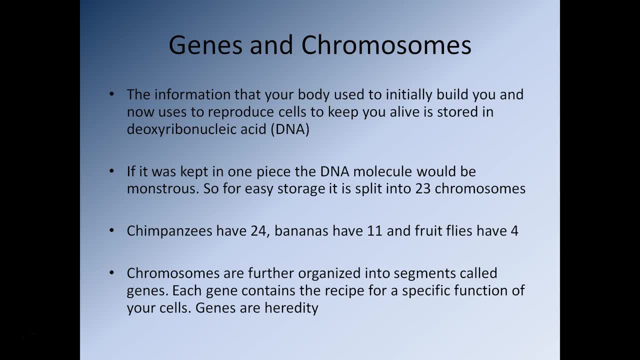 dna into chromosomes. now, in the case of chrome, in the case of human beings, we have 23 chromosomes. so just for argument, just for points out, chimpanzees have 24 chromosomes, bananas have 11 chromosomes, fruit flies have four. so the number of chromosomes varies between species. 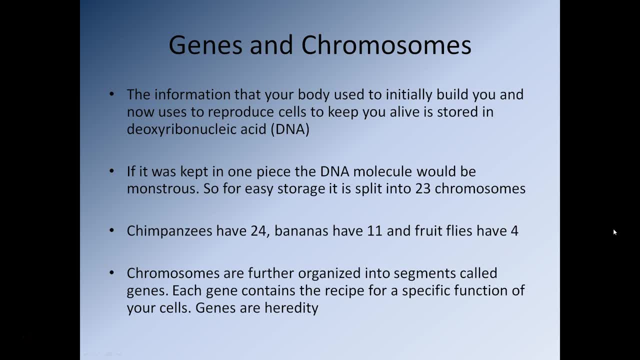 and the number of chromosomes does not denote intelligence- okay, because i'm almost certain that a banana is less intelligent than a fruit fly. so chromosomes are further organized into segments called genes, and each gene contains the recipe for a specific function of your cells. now, genes are hereditary, so that means the genetic information that makes up your 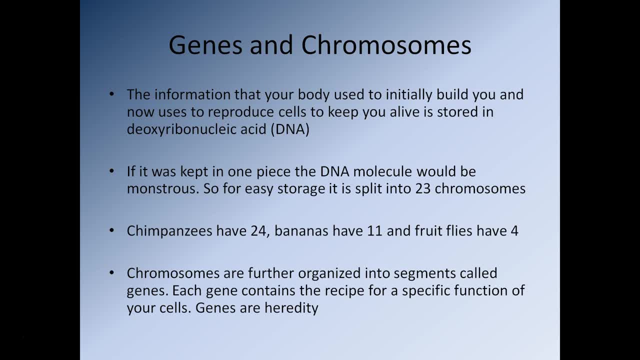 DNA is not a genetic information. it's a genetic information that makes up your DNA. so that means the genetic information that makes up your DNA is a genetic information that makes up your DNA, and therefore your chromosomes, is passed on from your parents, half of it from your mother, half of it from your father. 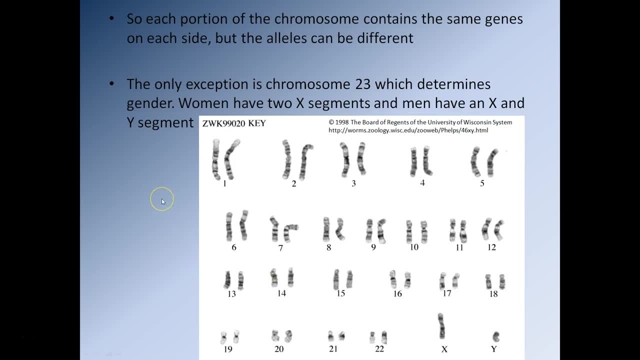 so each portion of the chromosome contains the same genes on each side, but the alleles can be different. so if we just know, for argument's sake, let's just look at, you know, chromosome number one here, imagine, we have an allele, so we have the same genes on both sides, but on this side the 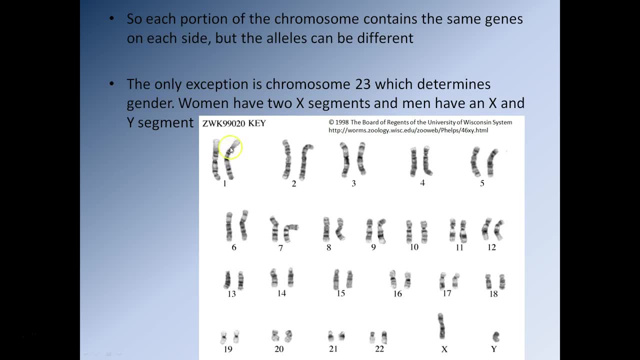 allele is for brown eyes. on this side, the allele is for blue eyes. in that instance, the brown eyes, the allele would be dominant. okay, so if we look at the, if we look at these chromosomes here- this is from a human being- we can see the chromosomes either side are mirror images of each other. now, 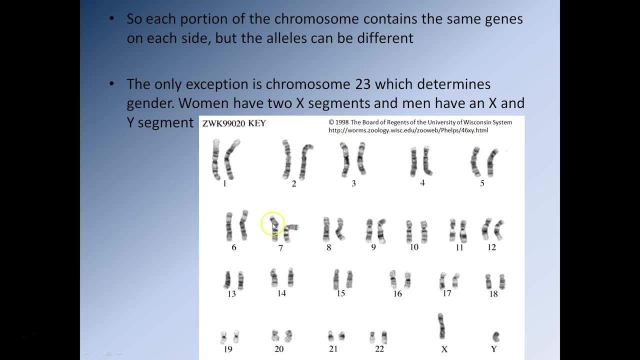 there are. there is some variation, you can see. that's purely due to the angle at which the photograph was taken. okay, that means they appear slightly different, but the chromosomes either side are the same. that's the one exception to that is chromosome 23. that's the only exception to that is. 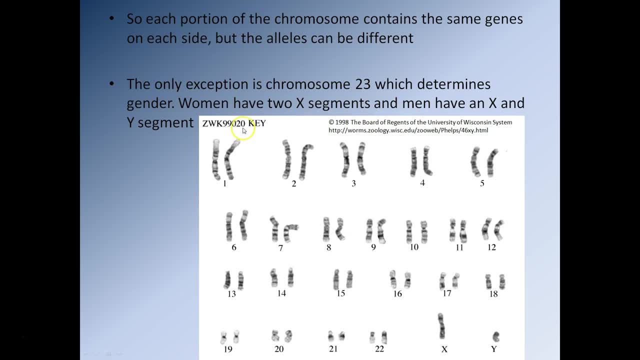 chromosome 24, that's the one that controls gender. so in the case of women, there are two x chromosomes, or two x segments, should i say, and that means there's an xx chromosome. in the case of men, we have the xy chromosome, so that's the only time where difference occurs. the other 22 chromosomes: 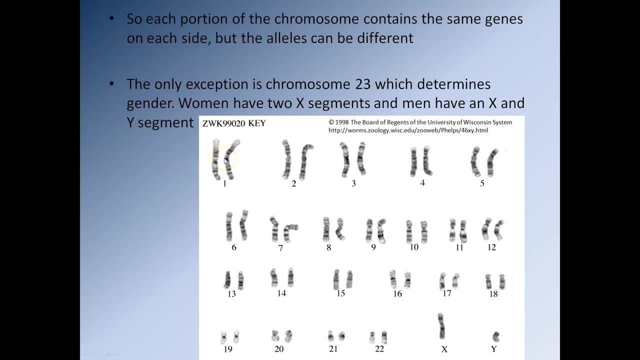 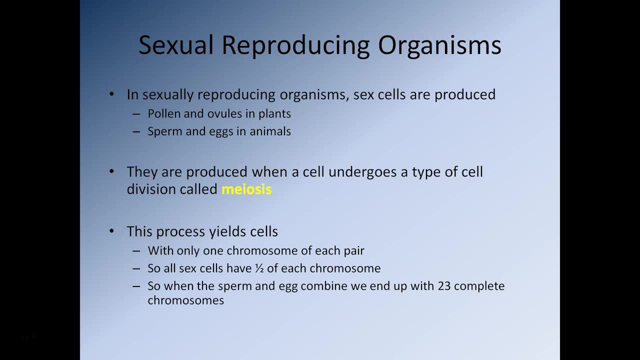 should, are pretty much mirror images of each other, each side. so this then brings us on to sexual reproduction. do you know what? it's nearly been 20 minutes. good place to pause, so let's stop here for a few minutes. once again, pause the presentation. get up, have a walk around going to drink water and come. 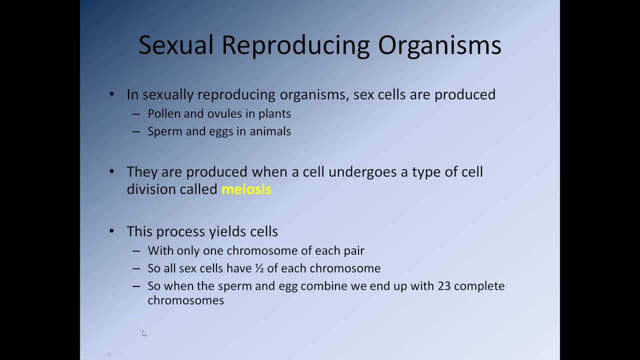 back to me in a few minutes. so okay, so on to sexual reproduction. so in sexual reproduction organisms produce sex cells. so the sex cells are either pollen and ovules in the case of plants, or sperm and eggs in the case of animals, and they are produced when a 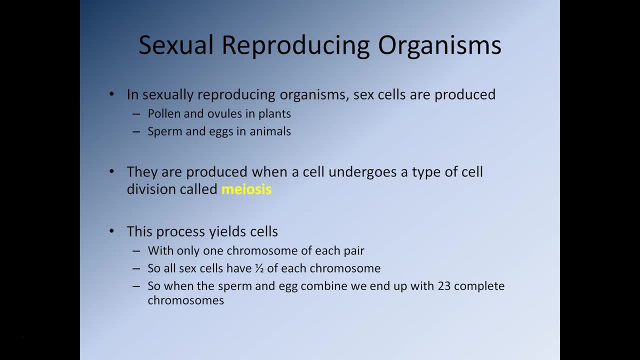 cell undergoes a type of cell division, which is referred to as meiosis. so this process yields cells that have only one chromosome from each pair, so essentially half of the genetic information from each parent, and so each cells only have half of each chromosome. and so when the sperm and egg 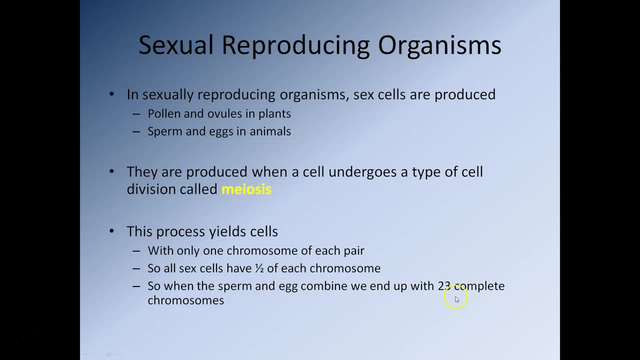 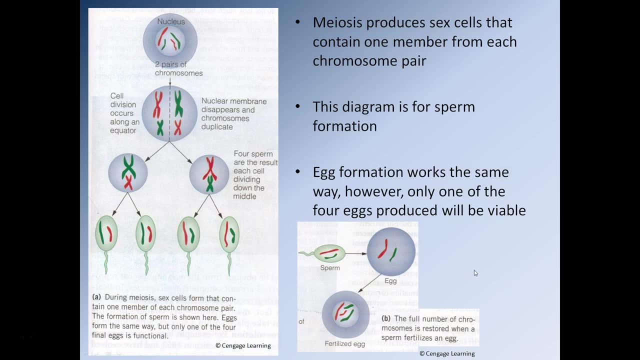 combine, you end up with essentially a complete set of chromosomes. in the case of humans, it should normally be 23 complete pairs. How does meiosis work? So here's our cell, and you can see it contains two chromosomes: a small one, so the green and the red sections, and a large one with once again green and red sections. 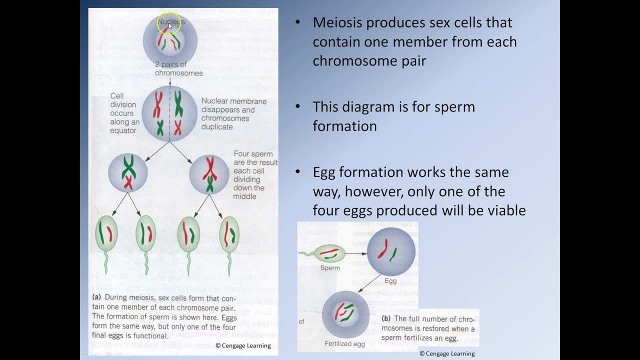 so the chromosome is going to be split into two, so we now have half of each chromosome. so what's going to happen is each half of the chromosome is going to be reproduced, it's going to be copied, and so we're going to end up with one big red chromosome, one big green chromosome, one small red chromosome. 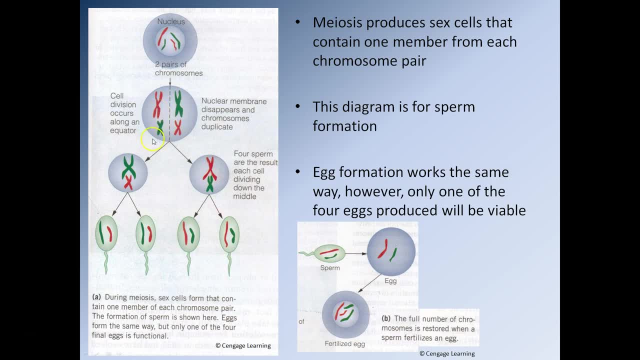 one small contact chromosome, one small red chromosome and one Azimuth chromosome, one small contact chromosome, small green chromosome. So, eventually, what's going to happen then is each of so the cells are going to divide in two, so the chromosomes are going to go this way and this way, so as you can. 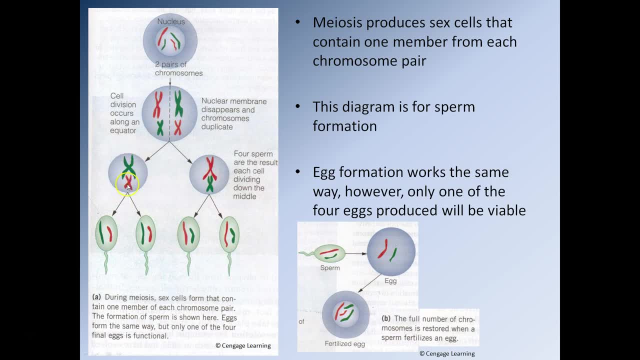 see, we now have a cell that has a big green chromosome and a little red chromosome, and a big red chromosome over here and a little green chromosome, and then this cell is going to divide again straight down the middle, the chromosomes are going to get split in two, and so now we have 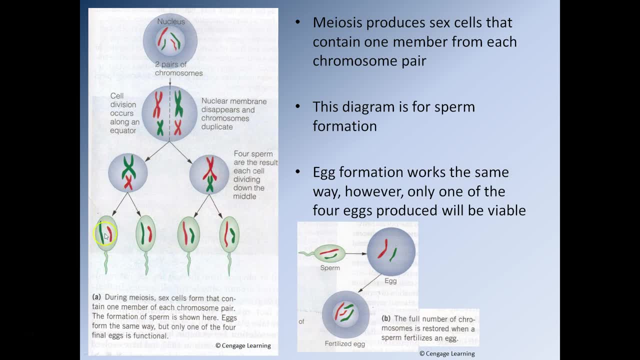 one, in this case sex cell- with a green and a little big green little red, another one with a big green little red, another one with big red little green and another one with big red little green. Okay, so essentially we've taken one cell and we've produced four sex cells as part of the 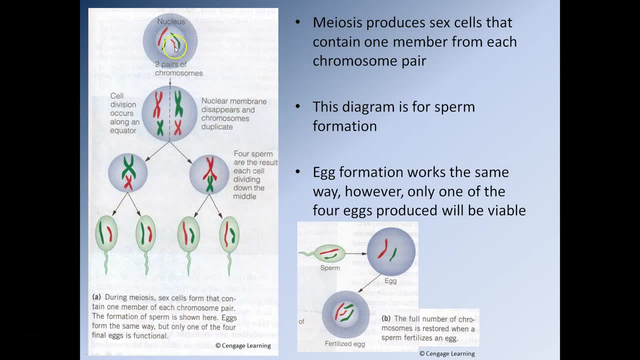 process. So this diagram is exactly the same for the formation of eggs. however, in the case of eggs, only one out of the four cells produced will be viable. the other three will unfortunately not be viable. So obviously, when the sperm and the egg combine, you end up with a complete set. 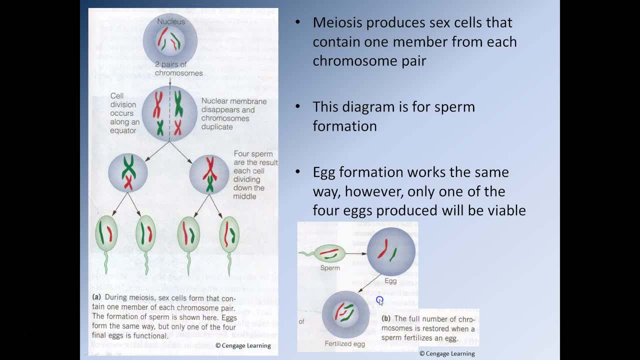 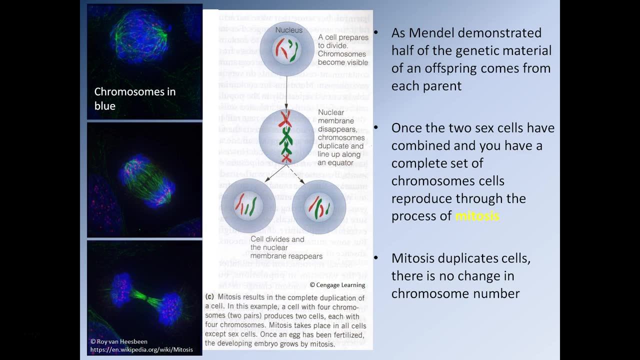 of genetic information. so that's meiosis. Now, once you have the cells they are going to want to reproduce, and cell reproduction takes place, or should I say replication takes place, through the process of mitosis. So once the two sex cells have combined and you have a complete set of 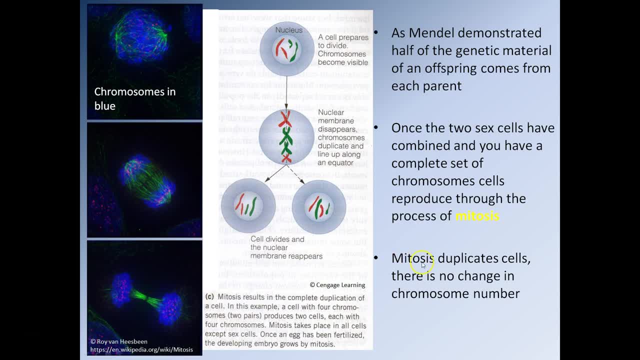 chromosomes. cells will reproduce through mitosis, So mitosis simply duplicates cells. there is no change in the chromosome number. So once again, here's our situation. we have two chromosomes. we have the big chromosome with the red and the green segments and the small chromosome with the. 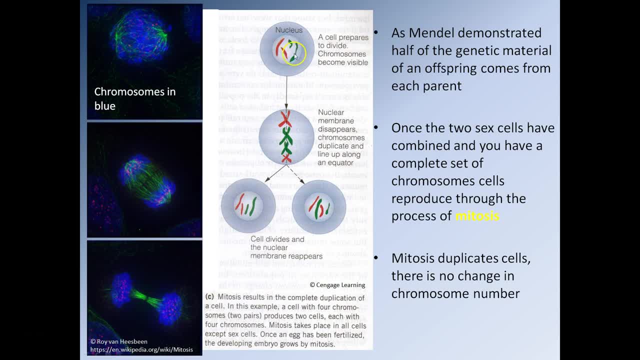 red and the green segments. So what happens is the cell splits the chromosomes in two. it then copies each half, so you end up with one big red chromosome, one big green chromosome, one little green chromosome, one big green chromosome, and then you have a complete set of 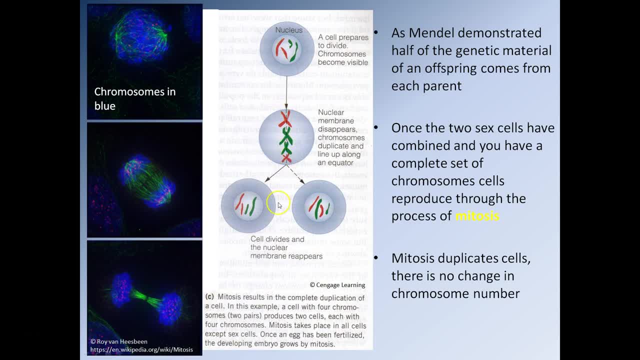 chromosomes, and then the cell simply splits straight down the middle and you end up with half the genetic information over here and half the genetic information over here, and so each cell essentially has a copy of the original genetic material from the parent cell. So it's all relatively straightforward, and you can kind of see it happening in this diagram here. So here's. 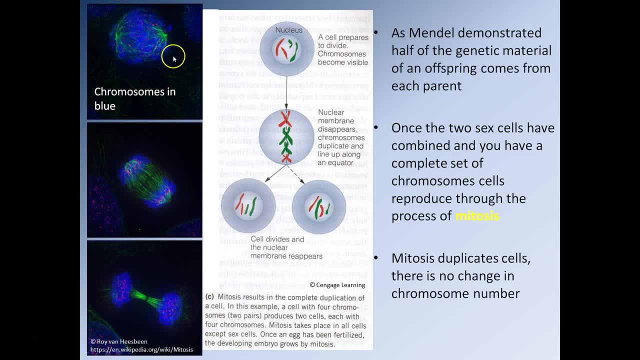 our situation. so in this case we have the genetic material is marked out here in blue. okay, so we have a set of chromosomes and then we have a complete set of chromosomes and then we have a pair of smaller them. we have a stream and then we have this- doctors and twins- and then we use the. 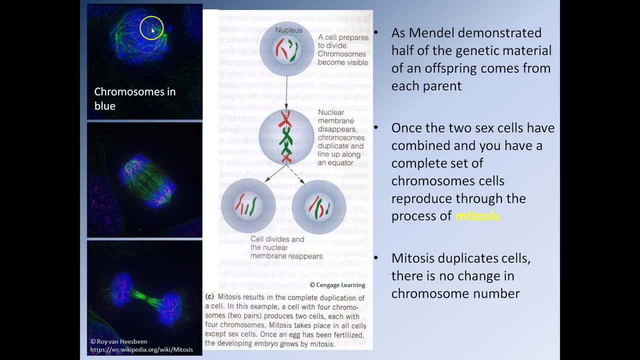 rowplex conseguir. so we look at that specific businessリhows key. my choice filled out in the sample, in theιοois muscle example, which is everywhere in the sample, where, as we can see, we have four cells and then we have a genetic material. and at this point here's our still. 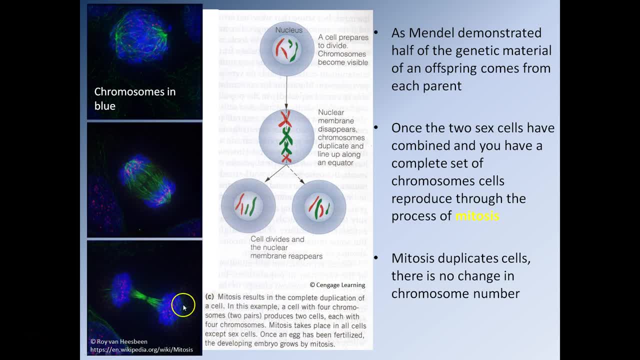 cell which is on the left hand side of theok. we now have 2 properties or a цвет, and then here's our sample of a small cell, and then we have a separated gen, eraeng. So now we've got 32, of which. we've got to be able to understand how they're separated, so it becomes a janganic. 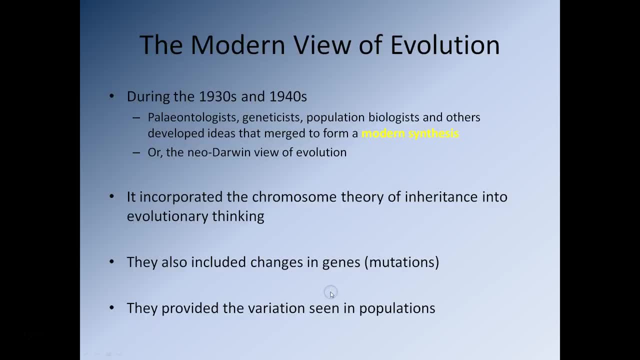 see the process happening. so what's the modern view of evolution? well, during the 1930s and 1940s things changed a little bit. so paleontologists, geneticists, population biologists and others developed ideas that merged to form what's referred to as the modern synthesis. it's also 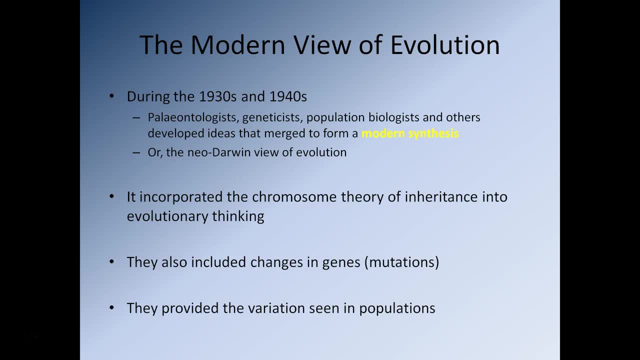 sometimes called neo-darwinism. so what neo-darwinism did is? it incorporated essentially genetic theory, so chromosome theory, the chromosome theory of inheritance, into darwin's model for evolution and essentially what that does is essentially, as soon as you do that it helps to explain how the inheritable characteristics can be passed on from one. 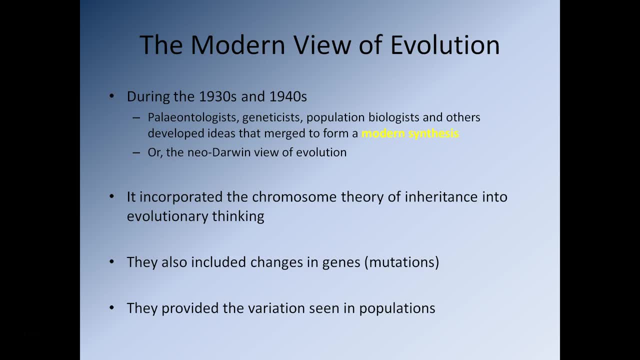 generation to another. they also included mutations in genes as part of the theory, so they they also included mutations and essentially mutations allow for variations, see, in population. so a mutation essentially allows a new variant to essentially pop up out of nowhere. so once we have this, you know, once we have this new modern synthesis put together, essentially, 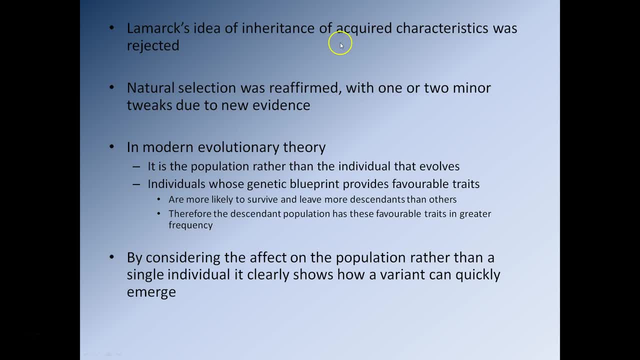 from that point on, it means the Marx idea of inheritance, of acquired characteristics, is now completely rejected. so once we have the modern synthesis, natural selection was reaffirmed, with one or two minor tweaks due to new evidence. so evidence so这里. so once you had that enough information to actually be able to. 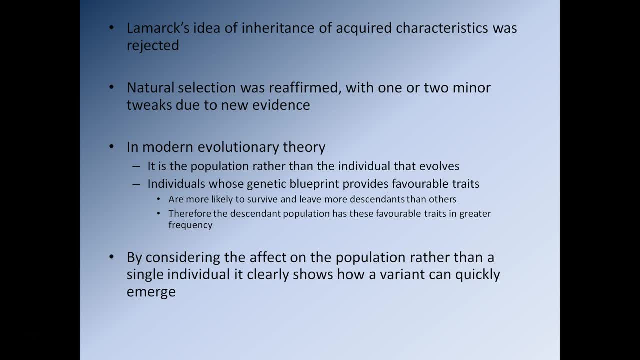 you know all you had an idea that you wanted to just stratify, and this et al math would意 fixture a. so this Zheng Tei is: survive and leave more descendants than others, and therefore the descendant population has those favourable traits in greater frequency. So you know, once we begin to consider things as a population, essentially these two points. 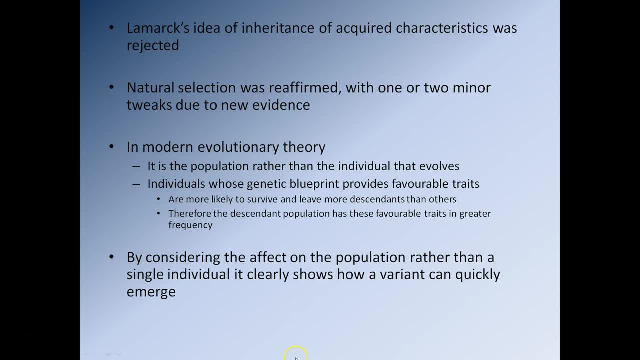 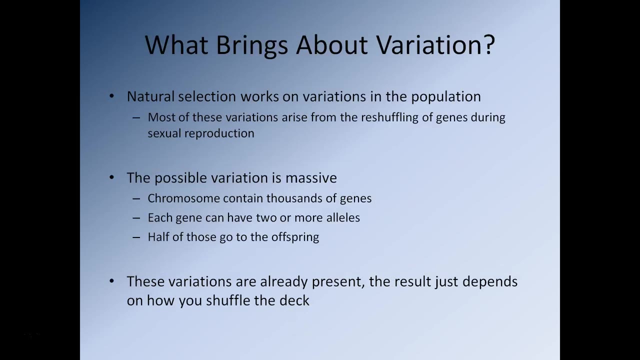 become more and more important. So by considering the effect on the population rather than the single individual, it clearly shows that how a variant can very quickly emerge from a population and become dominant within just a few generations. So what brings about variation? So natural selection works on variations in the population. 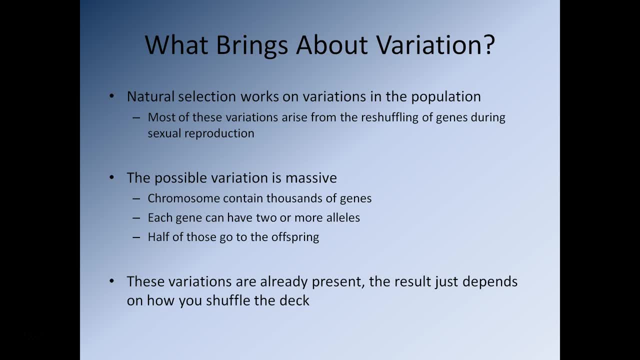 I mean just, you know, think about human beings. There is a considerable amount of variation. Every human being is different to every other human being. So most of these variations arise from the reshuffling of genes during sexual reproduction. So most of our genetic information, all of our genetic information, comes from our parents. 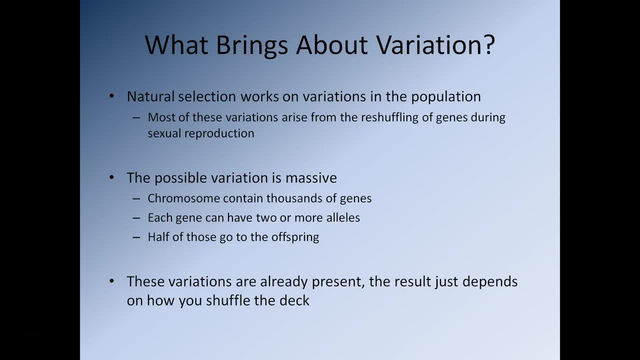 and therefore most of the variations we have are essentially inherited from our parents. So the possible variation is massive. So chromosomes contain thousands of genes. each gene can have two or more alleles, and half of those go to the offspring. So you know, there's a lot of ways that you can shuffle the deck. 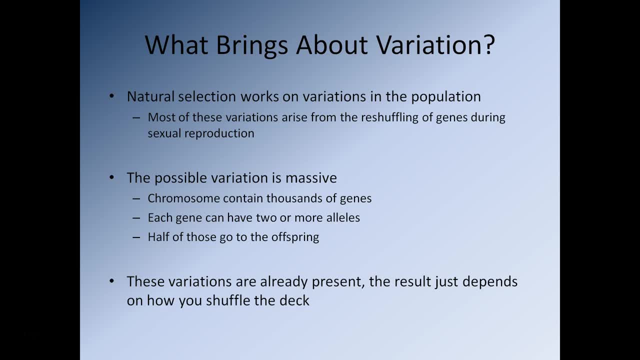 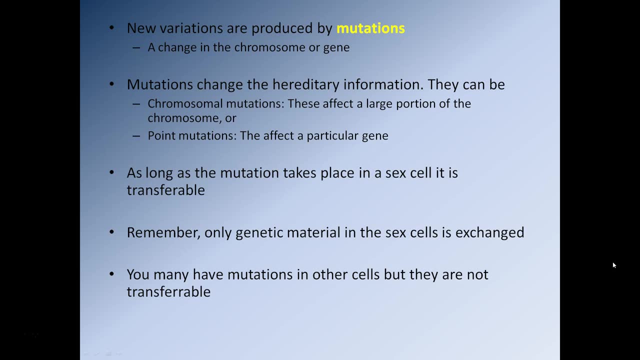 So these variations are already present, and the result just depends, as I say, on how things work out. What about new variations, though? Well, new variations are produced by mutations. A mutation is a change in the chromosome or gene, So mutations change the hereditary information. 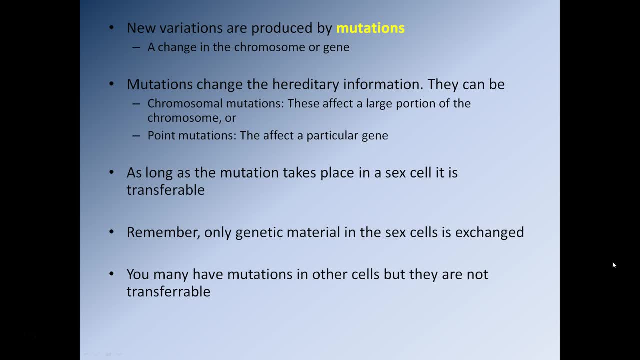 They can be chromosomal mutations that affects a large portion of the chromosome, or they can be point mutations that affect a particular gene. As long as the mutation takes place in a sex cell, it is transferable. So you know, if the mutation takes place in your liver cells, well, it's not valid in 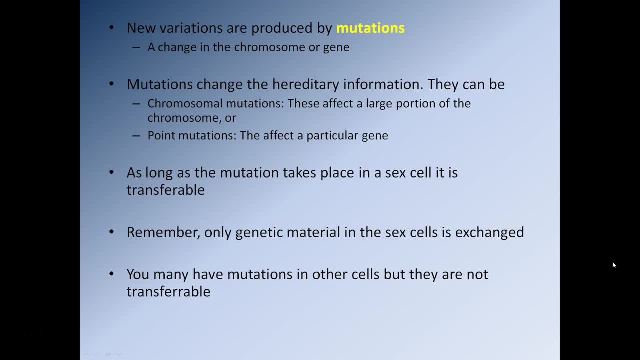 Well, it's not transferable because that genetic information will never be essentially used to essentially make offspring. So remember that only genetic material in the sex cells is exchanged And you know, as I just said, you can have many mutations in other cells. 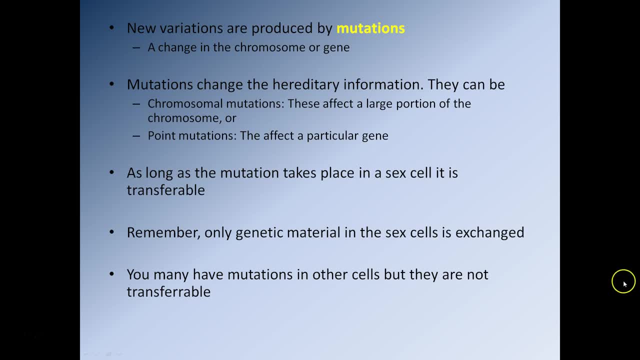 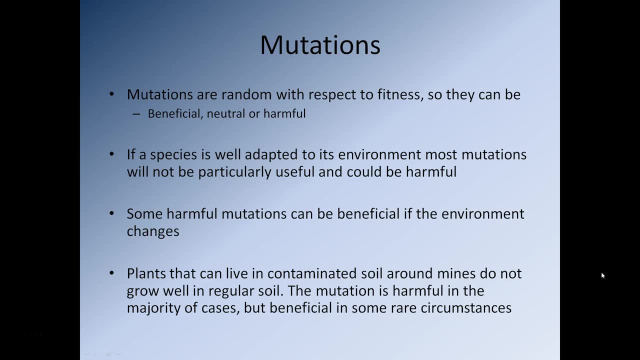 but they're not actually transferable to the next generation, so they're not important in this case. So mutations are random with respect to fitness. So essentially any member of a population can have a mutation and the mutation can either be beneficial, neutral or harmful. 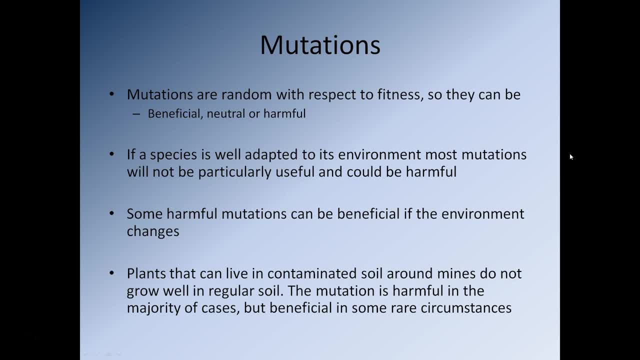 So if a species is well adapted to its environment, most mutations will not be particularly useful or they could be harmful. So let's think of something like the organism Lingula. So Lingula is a shelly organism. It burrows into sand and essentially it sticks out. 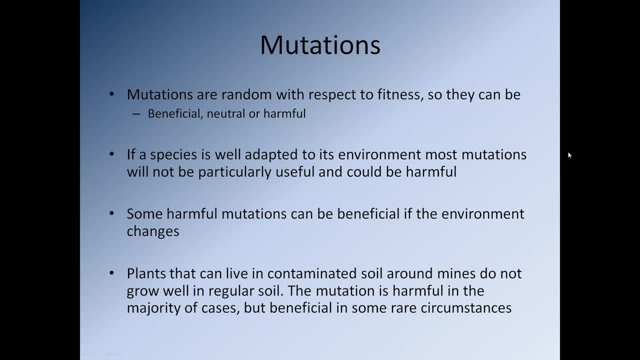 It's got a very long proboscis that it sticks out onto the seafloor, which it uses to grab stuff scuttling by, or it uses to grab food particles from the water. Now Lingula hasn't really changed in appearance. 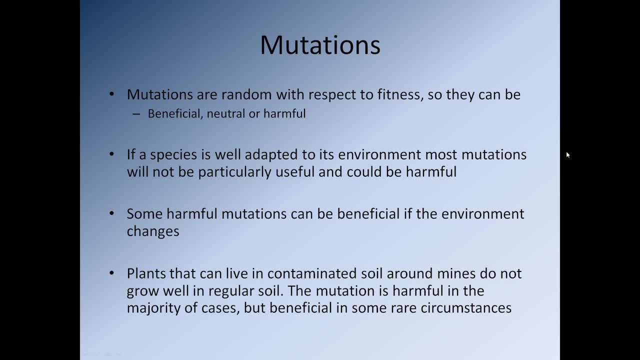 since about 420 million years ago, give or take a little bit, So it's extremely well adapted to its environment. So that means any change, you know, in its body shape, any change you know, any variation that occurs is more than likely either going to do no good or it's going to be harmful. 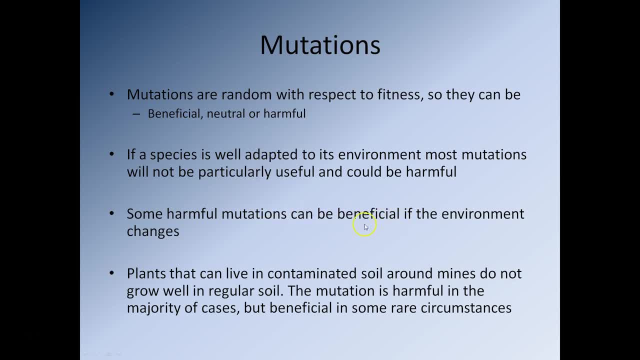 So some harmful mutations can be beneficial if the environment changes. So that's, you know, that's one of the key factors. So sometimes a variant can be bad, but if the conditions suddenly change and that variant, you know, suddenly becomes useful, 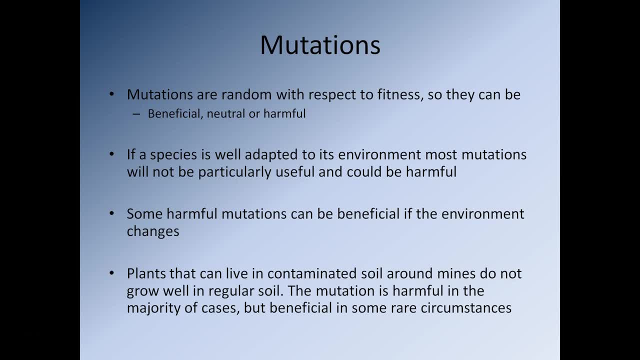 well, in that case you have the variant that makes you successful. So, for instance, you know there are certain types of plant that can live in contaminated soil around mines. Normally plants can't grow in that soil. You know it's full of, let's say, depending on the type of mine, you know, lead or mercury. 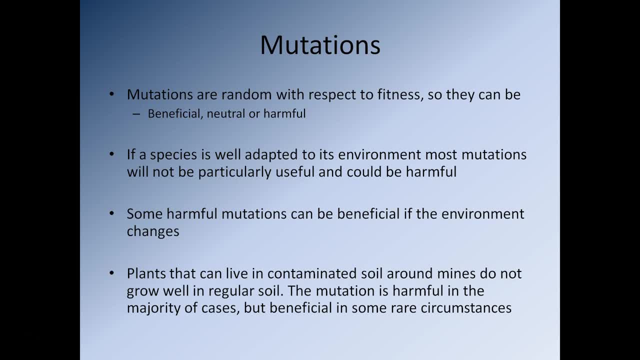 or lots of, you know, lots and lots of zinc or copper, And most plants, when they try and grow in that kind of soil, will just die. However, there are some plants that can grow in that very, very contaminated soil. 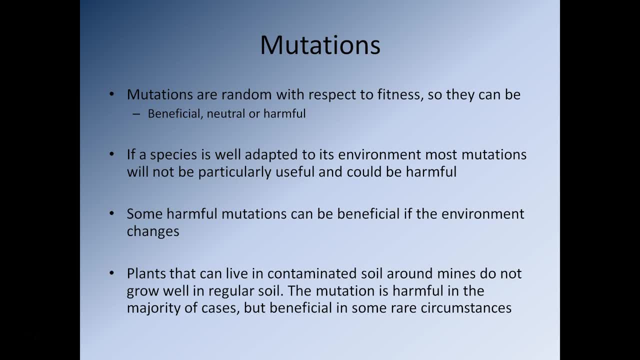 Interestingly, though, if you try and take that plant and you try and grow it in normal soil, it won't survive. So the mutation that makes that plant capable of growing in contaminated soil is beneficial when growing in contaminated soil but harmful when growing in normal soil. 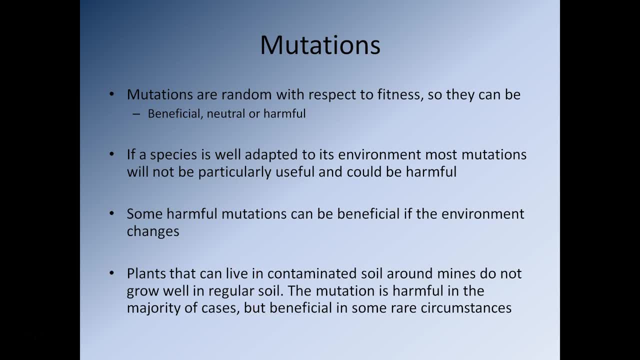 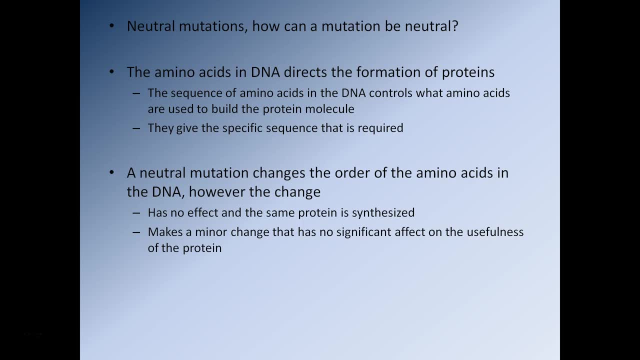 So you know whether a mutation is a good thing, a bad thing or neutral just depends on the exact environmental conditions at that time. So what about neutral mutations? How can a mutation be neutral? Well, the amino acids in DNA essentially directs the formation of proteins. 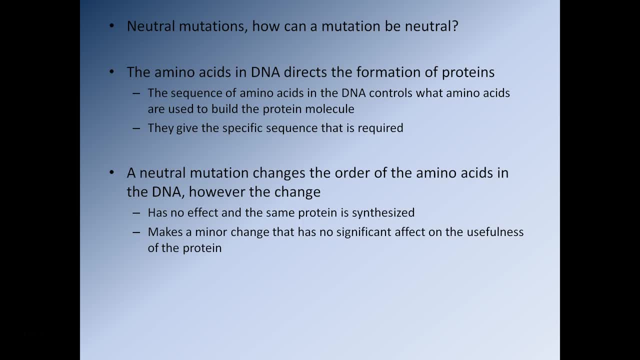 So the sequence in which the amino acids are stacked controls what protein is produced. Okay, So they give the specific sequence that's required to form distinct proteins. So obviously that means if you shuffle the order in which the amino acids in DNA occur, 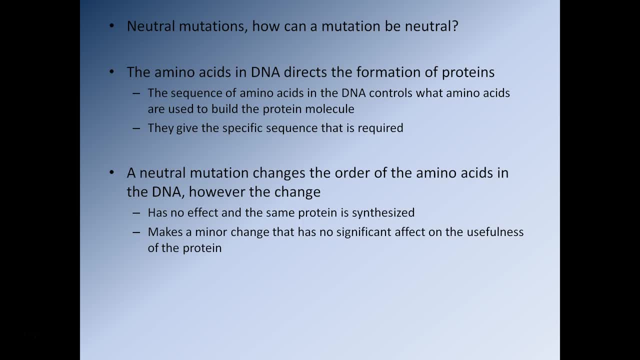 that means you're going to get a new protein. So a neutral mutation will change the order of the amino acids in the DNA. However, sometimes the change has no effect on the protein synthesized. So, even though you change the order of the amino acids in the DNA, 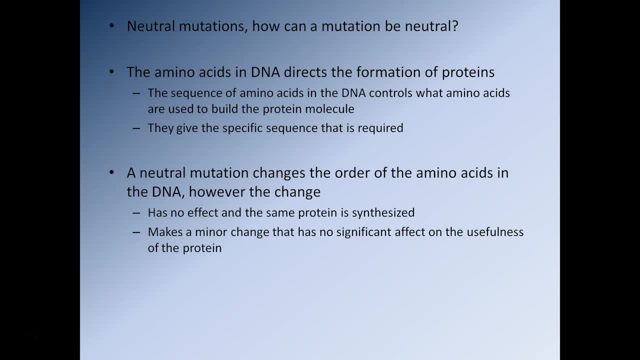 you still end up with exactly the same thing being made and it makes no difference. Or if it does change the protein that's being made, it doesn't change the protein in a way that significantly affects the usefulness of the protein. Okay. 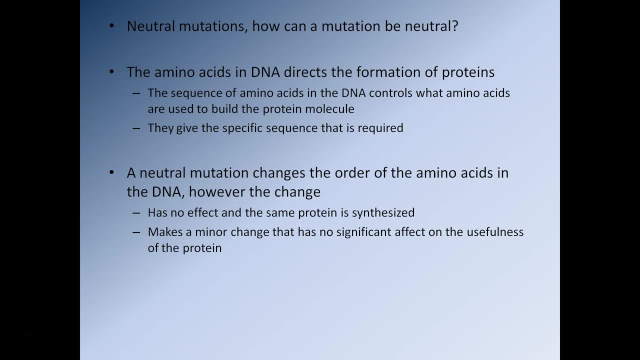 So you know you may be trying to make protein one. the DNA is slightly changed, it means you end up making protein two. but protein two can perform the same task as protein one, pretty much just as well. So you know there's no real loss. 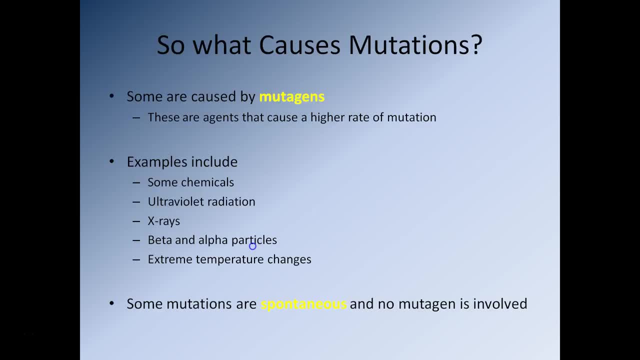 So that's how a mutation can be neutral. So what causes mutations? Well, some mutations are caused by a mutation that's not neutral. Some mutations are caused by things called mutagens, And these are agents that cause a higher rate of mutation to occur. 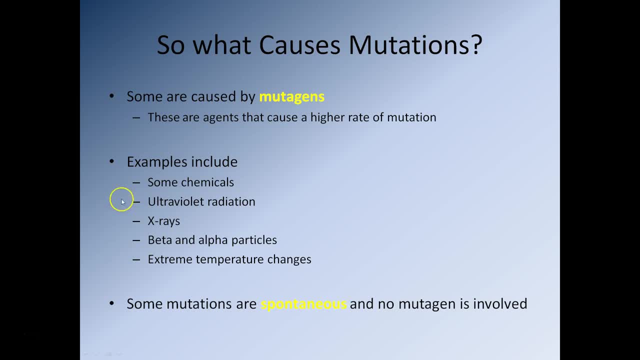 And examples of mutagens include some chemicals, ultraviolet radiation, x-rays, beta and alpha particles, so essentially particle. radioactive decay and some extreme changes in temperature can also cause mutations to occur, And some mutations are what we refer to as spontaneous. 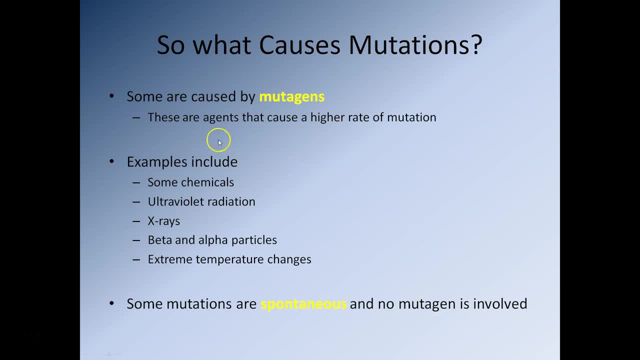 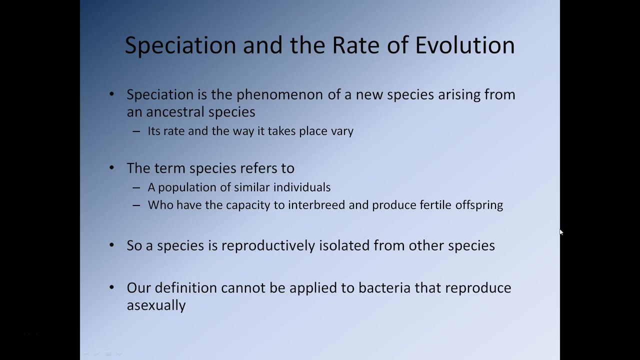 There is no mutagen involved. Okay, So if a change occurs due to a mutagen, essentially it's just due to a mutagen. If it occurs out of nowhere, it's referred to as spontaneous. So speciation is the phenomenon of a new species arising from an ancestral species. 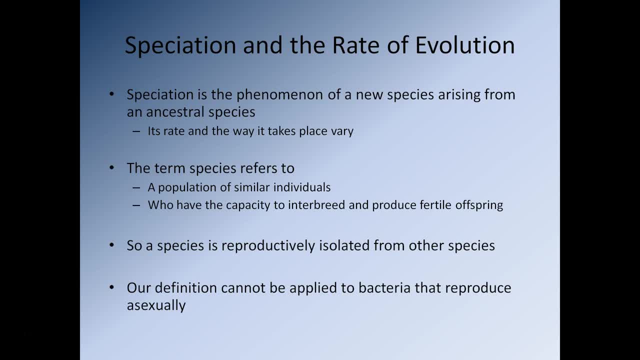 And, as we've discussed, essentially this is all due to natural selection, It's all due to the appearance of variants, due to mutation. So speciation is the phenomenon of which a new species arrives from an ancestral species. Its rate and the way it takes place vary. 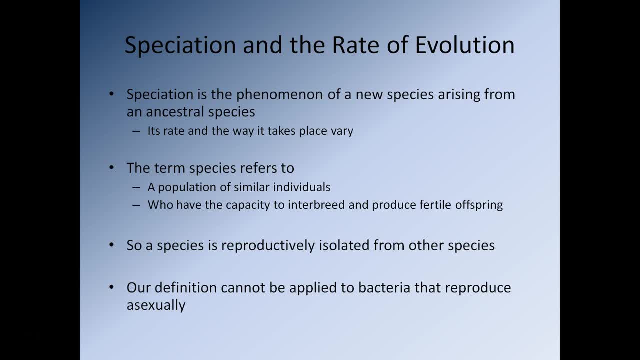 because obviously, you know, it's never a constant process. So the term species refers to a population of similar individuals who have the capacity to interbreed and produce fertile offspring. So a species is reproductively isolated from other species. So our definition cannot be applied to bacteria that produce asexually. 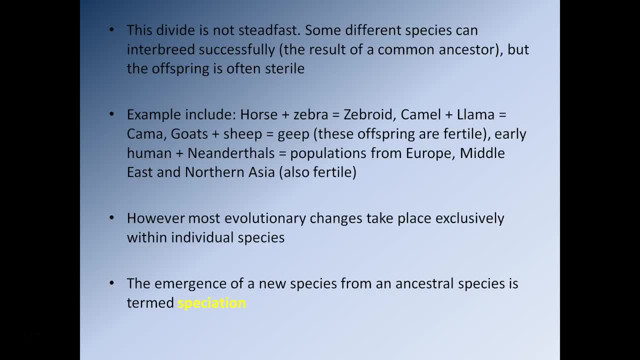 That essentially can reproduce themselves. So this divide, this species is reproductively isolated. this divide is not 100% steadfast. So some different species can interbreed successfully And that's typically because they have the result of an ancestor that's relatively recent. 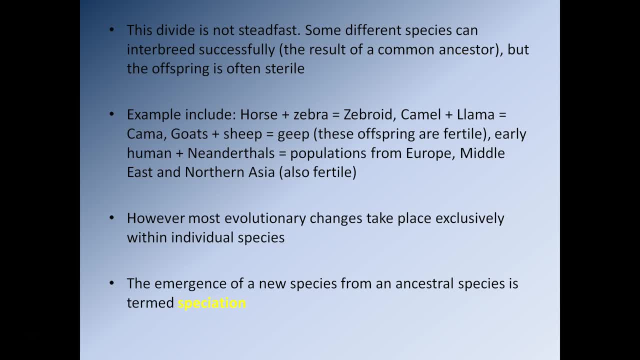 But the offspring is often successful, Okay, And the offspring is often sterile in most cases. So classic examples are: you can breed together a horse and a zebra to create a zebroid. A camel and llama produces a kama, Goats and sheep produce a geep. 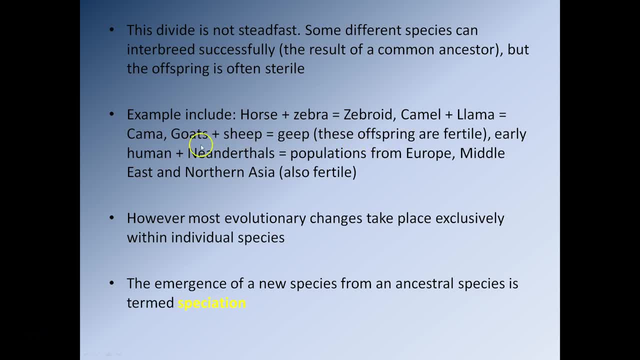 Geeps are fertile so they can reproduce And of course early humans and Neanderthals managed to reproduce and they produced fertile offspring. So Neanderthal DNA makes up a proportion of human DNA. The concentration of Neanderthal DNAs is typically highest in Europe. 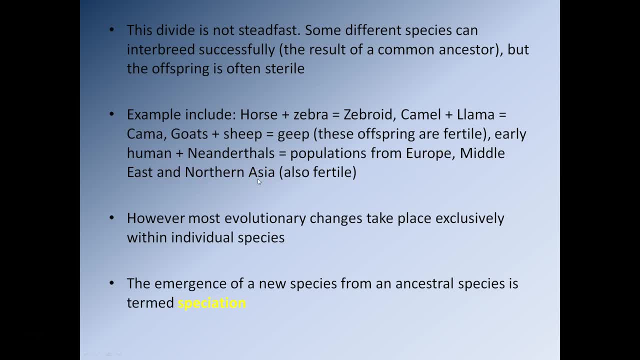 the Middle East and Northern Asia. Okay, I believe the highest population is found in Northern Italy And the next highest groupings are found in places like the United Kingdom, Denmark, Sweden, Finland, Norway, that kind of area- the Scandinavian and Northern European countries. 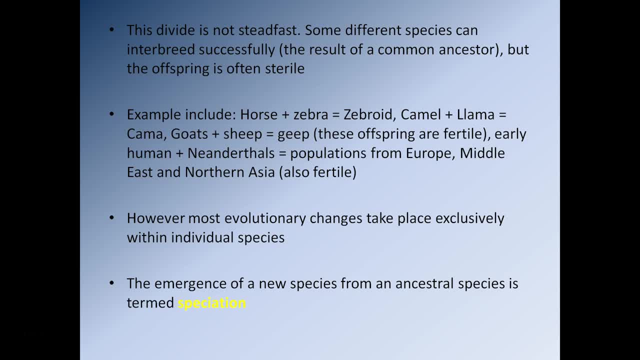 However, most evolutionary changes take place exclusively within individual species, So typically you don't really have species sharing genetic information. Most of the time, any genetic change that takes place within a species is just due to that changes within that species only. So the emergence of a new species from an ancestral species is termed speciation. 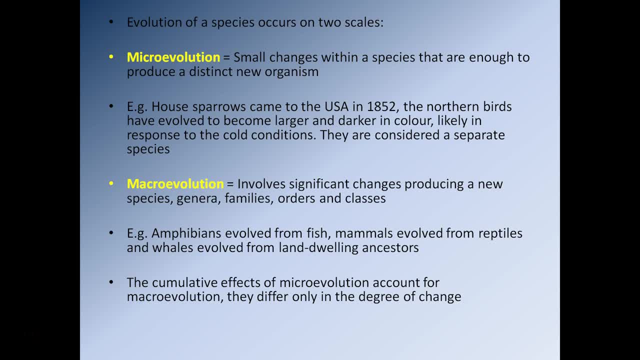 So speciation essentially comes through the process of evolution. There's two different types of evolution, So it occurs on small scales and large scales. So small scale evolution is called microevolution, And that's when you get small changes within a species. 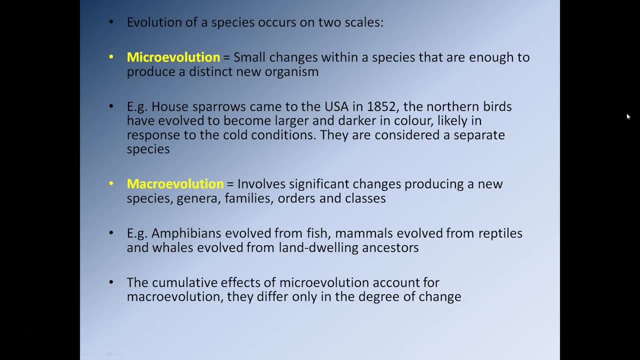 and they're enough to produce a distinctive new organism. So a good example of that is house sparrows. So house sparrows were introduced to the United States in 1852.. So they were introduced and some of the birds flew north and some of the birds flew south. 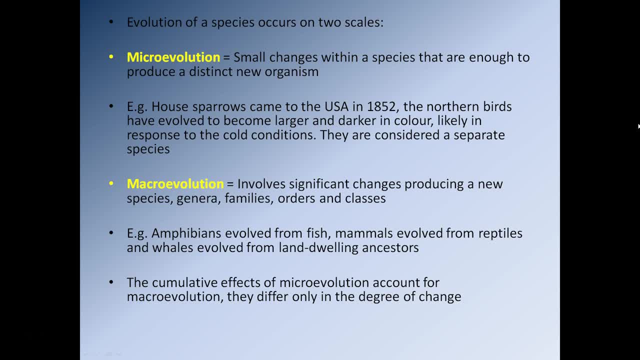 So, over time, over the last 60 something years- nearly 70 years in fact- the birds that flew north have evolved. They've become larger and they've become darker in colour because they have to survive in cold conditions. The birds, on the other hand, that flew south- 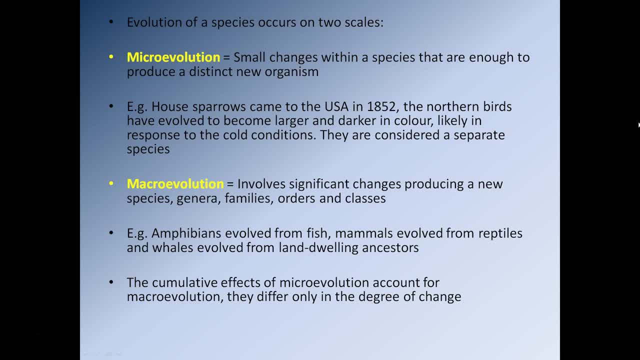 underwent relatively little change because they were living essentially in the kind of climate that species could live in without any need for any significant shift in body design. So essentially, the house sparrows that flew north are now considered to be a separate species. So just a few minor changes is sufficient to produce a new, distinct species. 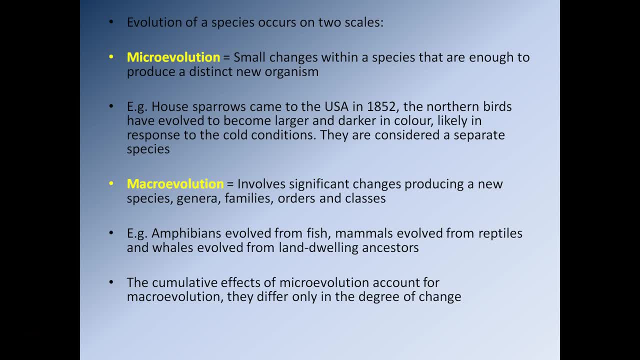 So then we have macroevolution. So macroevolution involves significant changes producing a new species, genus, family order or class. So for instance, you have amphibians, so you have fish. Fish slowly evolved over time, so microevolutionary steps eventually ended up in the production of amphibians. 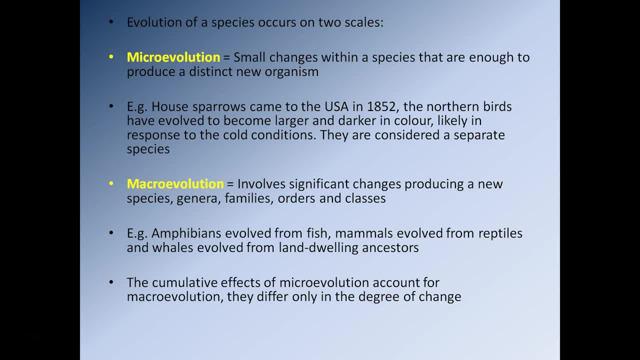 which are so different to fish that they are given their own family. Another example is mammals, So reptiles slowly over time began to develop more and more mammalian features. That's microevolution And eventually you get to the point where the offspring is so different. 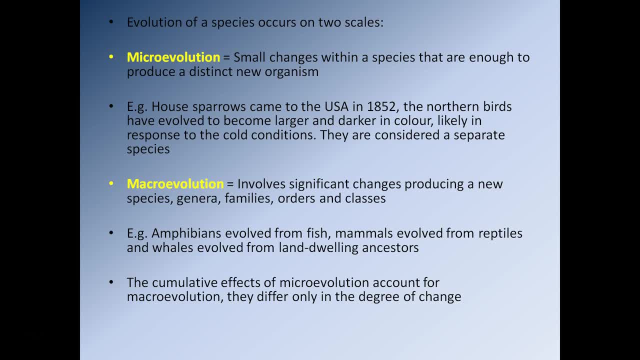 that it's once again given its own family, That's, the Ordo mammalia, And of course we have whales. Whales evolved from a land-dwelling organism that looked kind of like a cross between a kind of a wolf and a mouse. 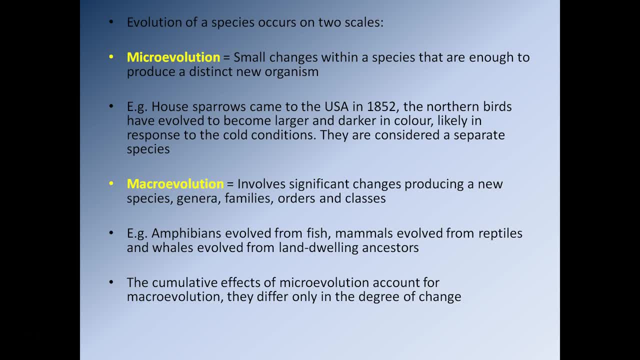 I should say a wolf and a rat. It was a very strange looking ancestor, but over time it's, you know, moved into the oceans and it's given rise to the whales, which are completely different in appearance, You know: huge tails, no limbs. 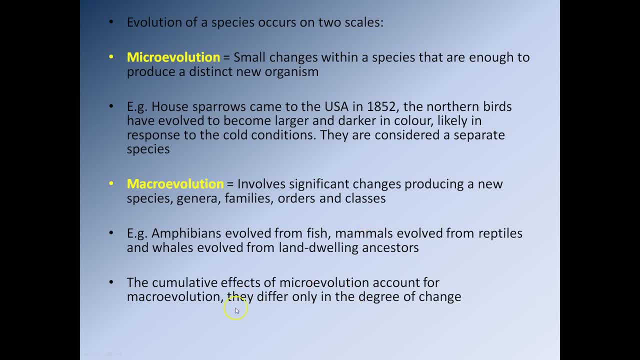 So the cumulative effects of microevolution account for macroevolution. They differ only in the degree of change, So microevolution tends to be a lot faster and it tends to produce individual species. Macroevolution will typically produce significant changes over time. 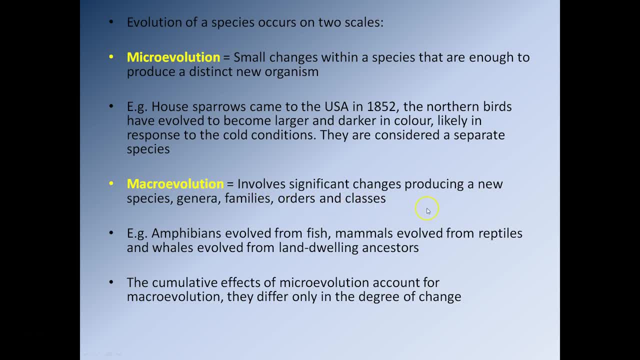 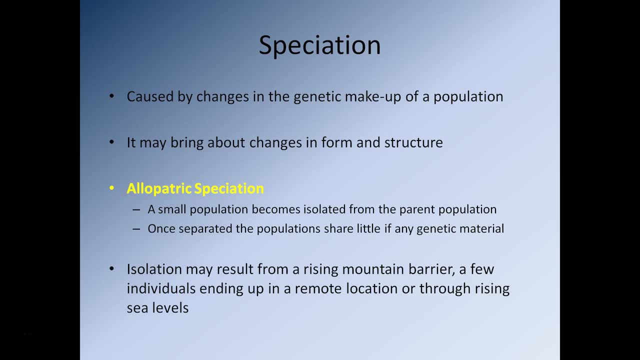 and typically it will give rise to new genuses, families, orders and classes. So speciation is obviously the result of changes in the genetic makeup of a population. So obviously, in order to adapt to any new environment, a population has to select certain variants. 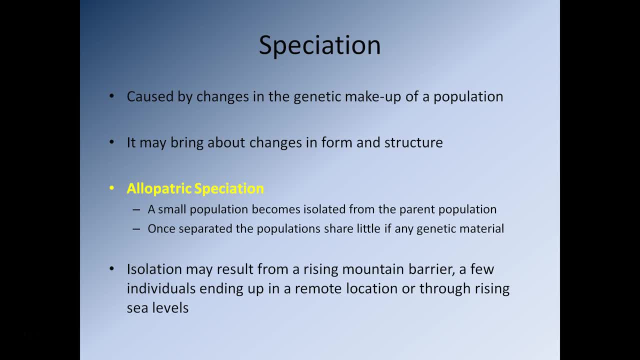 which are, you know, which are positive for that particular environment, and it will obviously reject some variants that have negative repercussions for that environment, And so that will lead to the evolution of a completely new and distinct species, designed for that particular area. So speciation may bring, you know, may bring about changes in form. 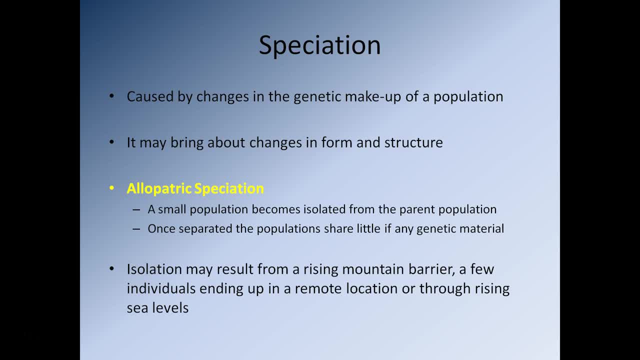 and structure. So you know, sometimes the species, sometimes the changes can be visible. Okay, You know changes in size, changes in limb design, for instance, And sometimes you know the changes may not be visible. It could be something like a change in digestive enzyme, for instance. 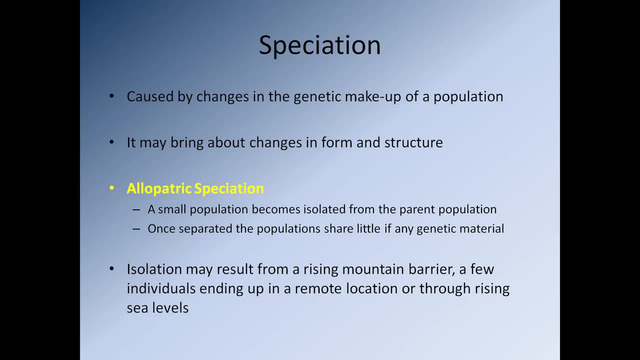 So speciation occurs in a few ways. So the first one is allopatric speciation. So that's when you have a small population that becomes isolated from the parent population And once separated, the populations share little, if any, genetic material. 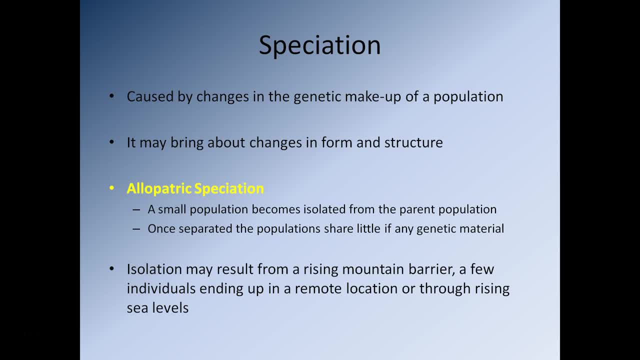 Therefore, they evolve in isolation from one another. So this kind of isolation may result from, you know, a rising mountain barrier, a few individuals ending up in a remote location or through rising sea levels. So, you know, a good example would be Madagascar. 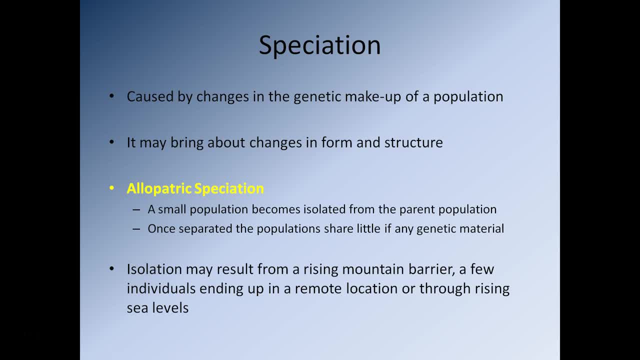 Once upon a time, Madagascar was attached to the east coast of Africa and eventually it rifted. It rifted off and went to form its own island, And so from that point on, essentially, the animals that were on Madagascar were isolated from the African communities. 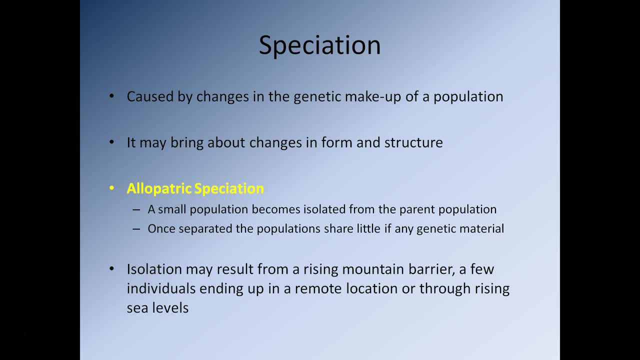 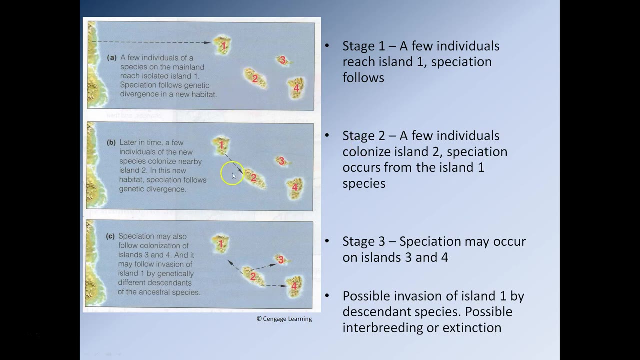 and therefore they evolved in their own way And they've been evolving for somewhere in the region of about 200 to 250 million years in isolation. So they are very, very different to the populations seen on the African continent. So this kind of gives you some idea. 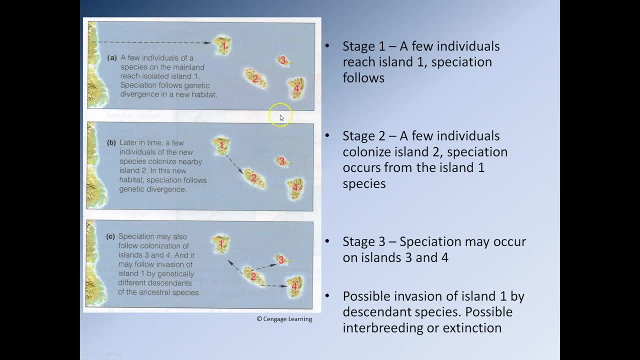 This is allopatric speciation based on, essentially, isolation due to being trapped on an island. So let's say we have some birds, Let's call, let's say, grass-quit finches, in fact, So they get caught, you know, on a very, very strong wind. 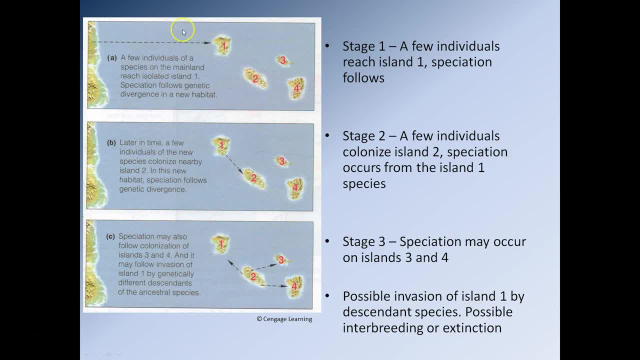 They get pushed out over the ocean. They end up all the way over here. They suddenly realize they've got to find somewhere to land And they spot this island. so they fly straight for it And this is their new island, This is their home. 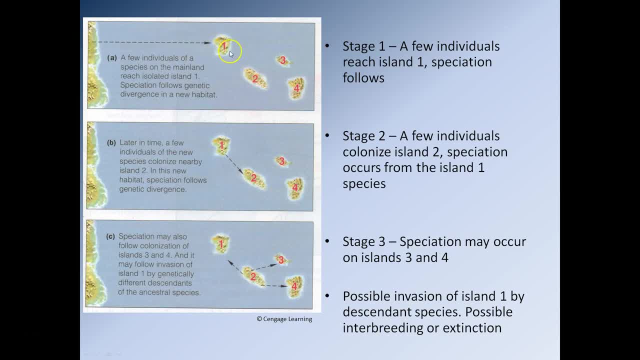 And, of course, they have insufficient energy to be able to fly back to the mainland. now They're an isolated population And so, obviously, the population will start to breed And natural selection will kick in, And certain variant types will be selected that are advantageous for the particular environment. 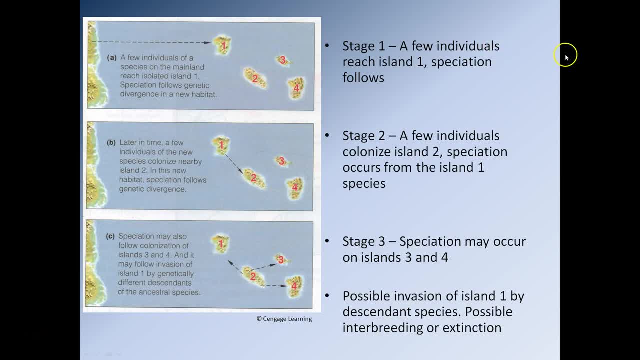 on island number one. Obviously, after a while, some of the birds from island number one will spot island number two and they think, all right, I'm going to give that one a go. So they go over to island number two. Island number two is going to have a slightly different environment. 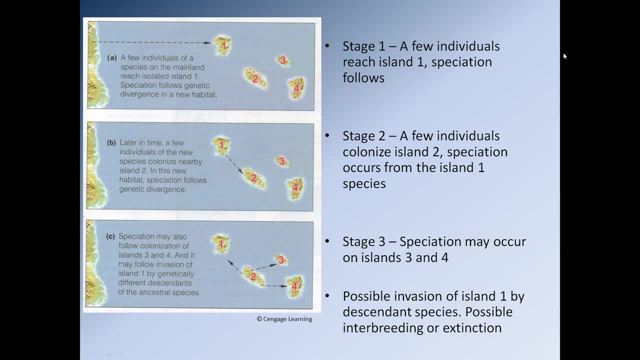 So, once again, the birds that make it to island number two, as they reproduce, each generation is going to produce a change, essentially a speciation, as the organism adapts to the conditions on island number two. From island number two the organisms go to three and four. 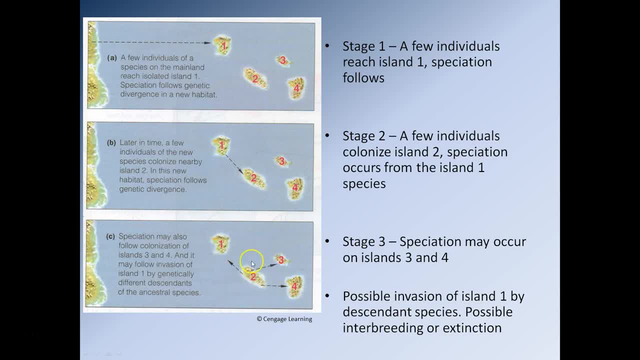 Now sometimes, let's say, the organism from island number two suddenly decides to go back to island number one. Well, only a couple of things can happen at this point. The birds on island number one and the birds from island number two will try to out-compete each other. 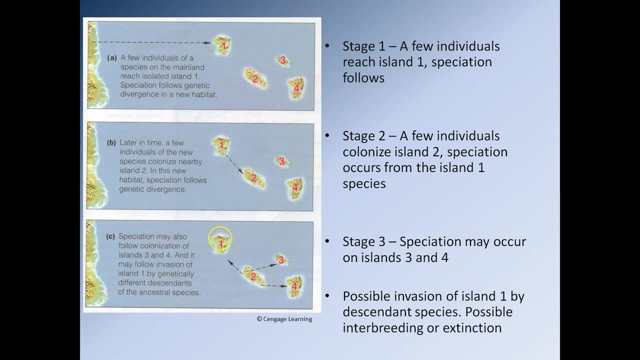 and one group will eventually win, Or the birds from island number one will interbreed with birds from island number two to create some kind of intermediate between the two distinct species. So those are your possibilities, But essentially this is speciation based on isolation. 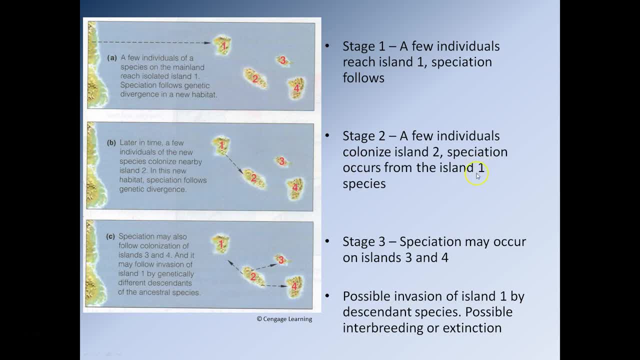 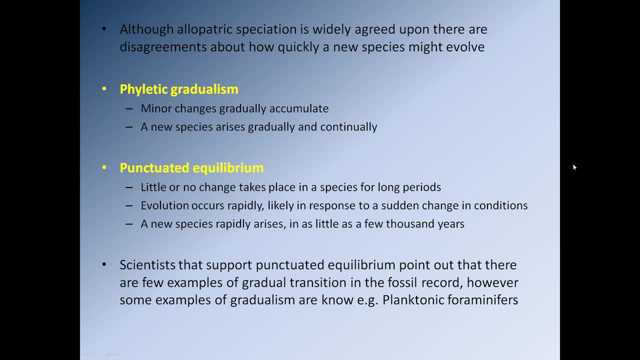 So each individual island has its own environment and the birds will adapt, evolve to each of those new environments. So although allopatric speciation is widely agreed upon, there are disagreements about how quickly a new species might evolve. So first of all, there's a phyletic gradualism. 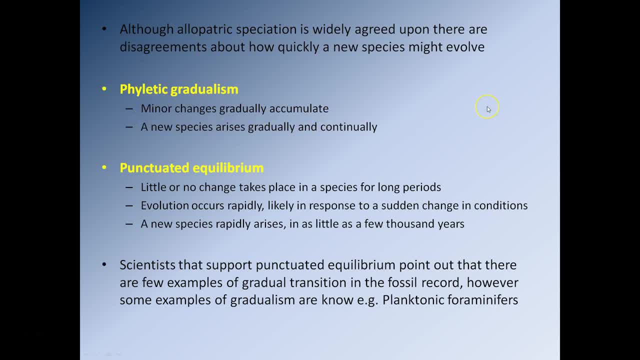 and that says that minor changes gradually accumulate over time and this means that new species arrive slowly and continually. Then we have something which is referred to as punctuated equilibrium And that says little or no change takes place in a species for long periods. It says evolution occurs rapidly. 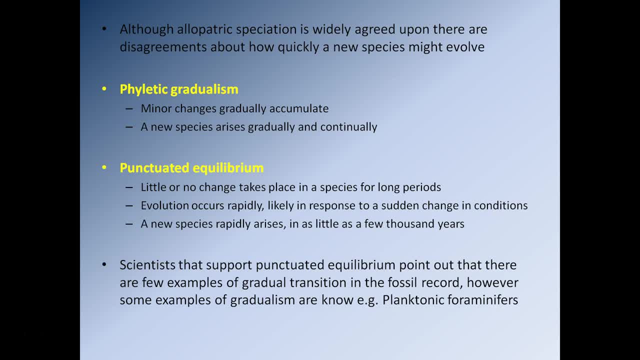 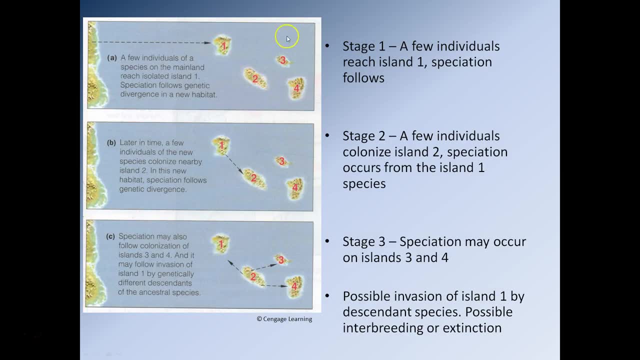 likely in response to a sudden change in conditions, And a new species will arise rapidly, in as little as a few thousand years. So let's think of our situation here: The birds on the mainland over here- well, chances are they are very well evolved. 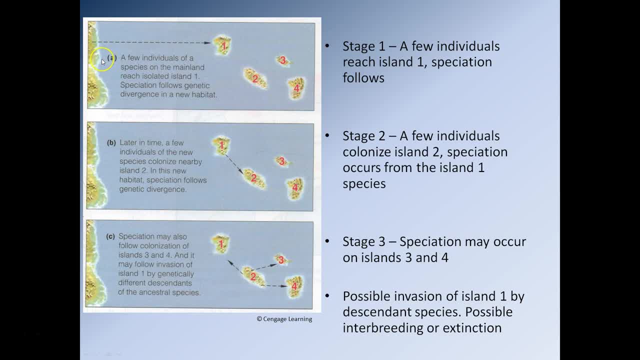 to their conditions, and so, as long as the environment isn't changing in any significant way, there's probably very little reason for them to evolve, for them to adapt, And so the animal will in all likelihood not evolve that much. Now, of course, as soon as some of the birds 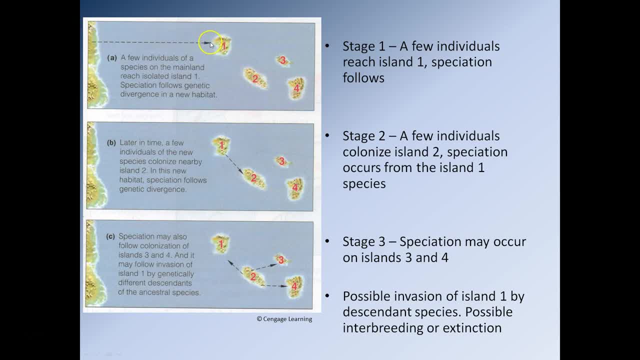 get blown out onto island number one. well, all of a sudden, island number one has a completely different environment, and in order for those birds to survive, they have to start adapting quickly. And so, in this instance, evolution is going to kick in very, very fast, because the organisms have to adapt. 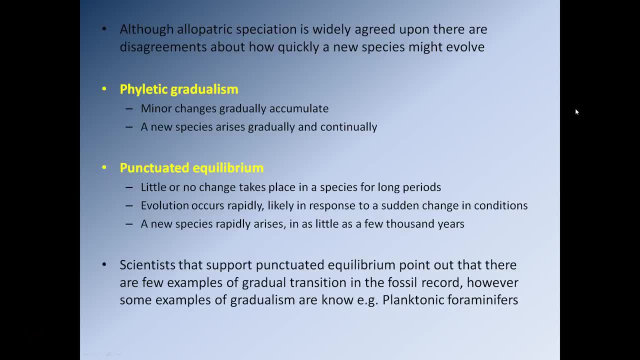 to the environment if they want their species to be able to survive on that island. So scientists that support punctuated equilibrium point out that there are very few examples of gradual transition in the fossil record. Most of the time when there is a change in the fossil record, it's often driven. 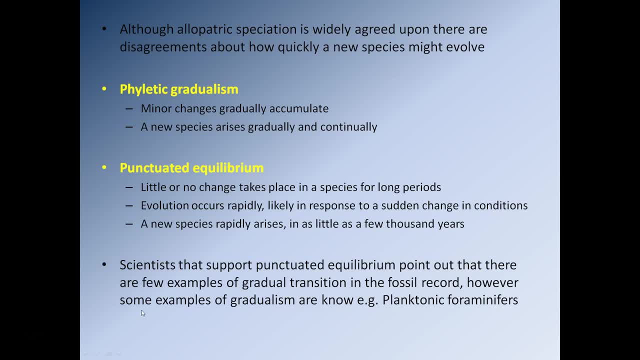 by some kind of event which we can see in the rock record. However, there are some examples of gradualism that are known, So things like planktonic foraminifera- these are little organisms that float in the ocean water, So both of these examples are correct. 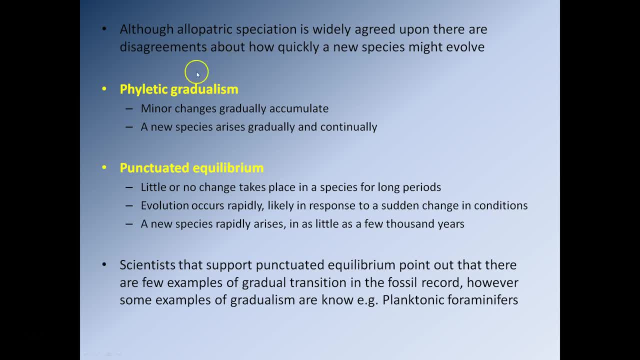 You can have lots of gradual change, producing new species, or you can have change driven by sudden changes in the environment, producing new species.